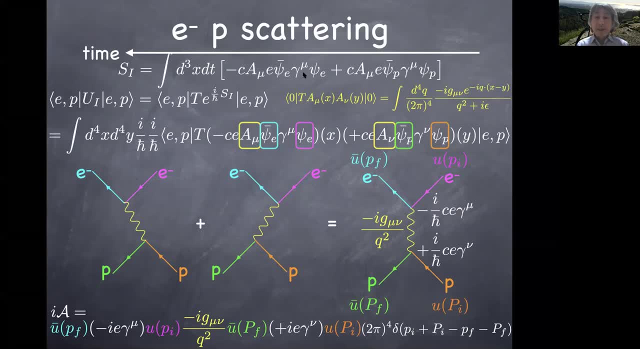 from the exponent, which is, in this time, evolution operator. And so, in this particular example of electron-proton scattering, I have one term for the proton field interacting with the electron magnetic field, another term for the electron field interacting with the electromagnetic field. 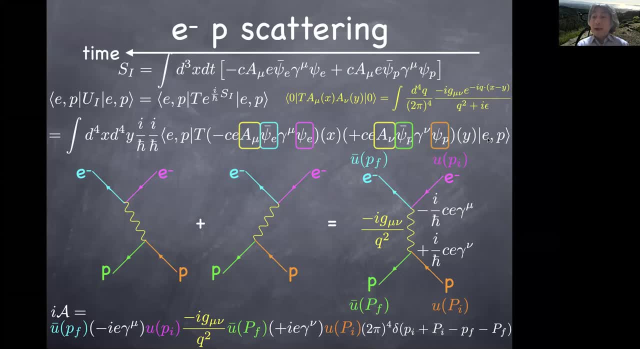 and these Dirac fields extract basically the positive energy solutions out of the mode expansion, because when you expand out the Dirac field it comes out to be the momentum integral of the annihilation operator of the particle times. the positive energy solution, and I use the 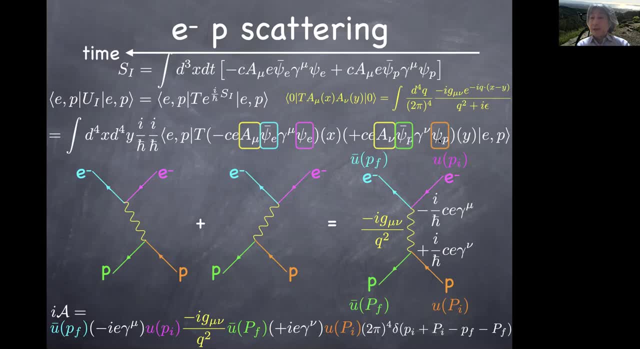 annihilation operator to annihilate the electron initial state. so part of Psi. what that remains is this positive energy solution. The same way here, the positive energy solution with bar on it. positive energy solution here for the electron. positive energy solution for the electron. 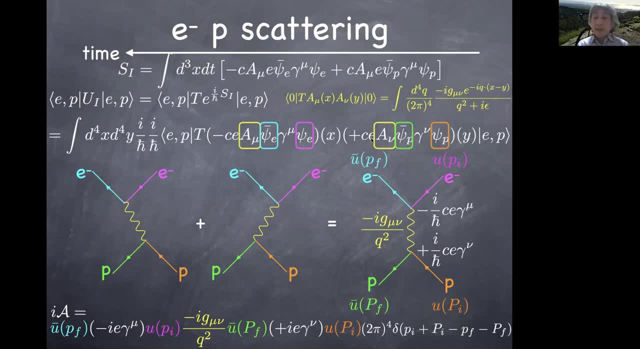 and bar on it, and then I use this propagator I talked about on Wednesday and you have been working on the propagator for the complex Klein-Gordon field, so I hope you're getting the idea how this time-order product or field operator works. 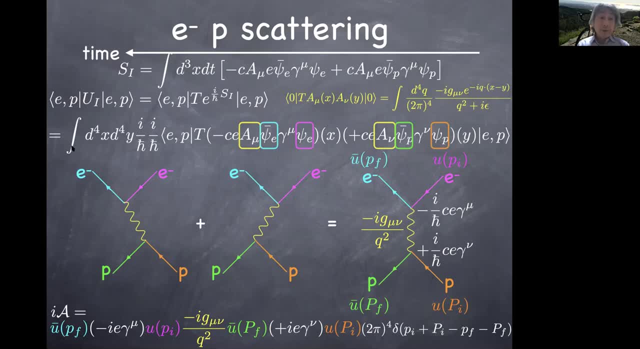 in momentum space and when you do the spatial integrals, then at the end of the day you find this overall momentum conservation as a result, but you also get additional constraint, namely that the full momentum you're supposed to use for this photon propagator. 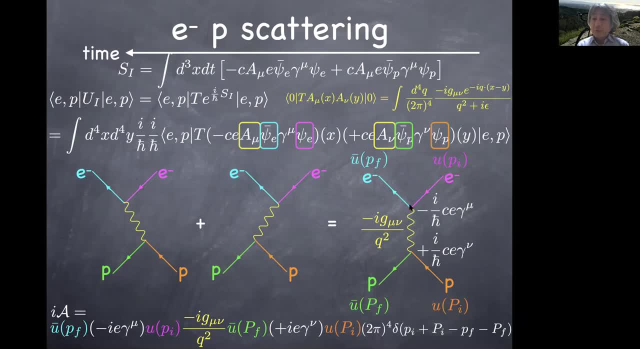 is really the difference between the initial full momentum of the electron and the final full momentum of the electron, which is what we call the momentum transfer. So in some sense there is this energy momentum conservation at this vertex, The amount of momentum that changed from initial state to final state. 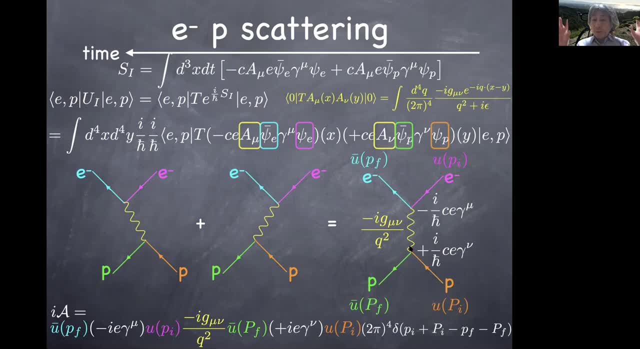 is what is emitted as the full momentum of this, what we call the virtual photon. It is virtual because the q squared of this photon is not zero. so that's the violation of actually energy conservation, because true photon with a full momentum are given a 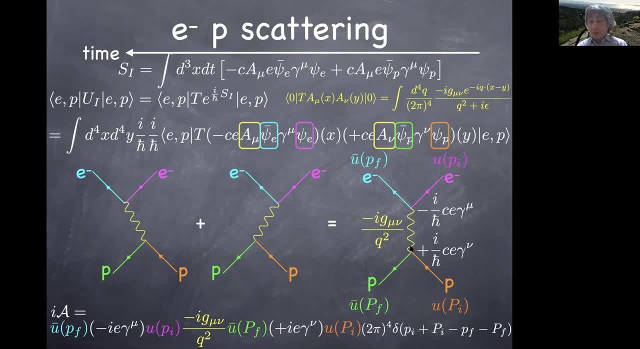 spatial momentum as the energy given by the spatial momentum and speed of light. But this photon, if you work out the kinematics, carries no energy. so you are emitting the photon whose existence already violates the energy conservation. So that's the reason why this corresponds to the intermediate state we talked about. 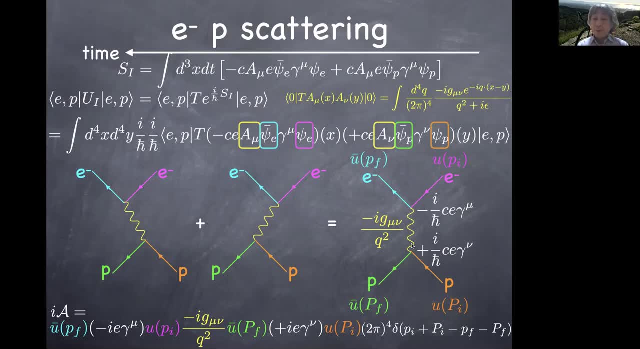 when we discussed the Rayleigh scattering using time-dependent perturbation theory. So intermediate states may not respect the wake-up density, but they don't have the opportunity correct energy conservation, and that's the meaning of being virtual. But in the Feynman rules the full momentum Q has to be exactly the same thing as the. 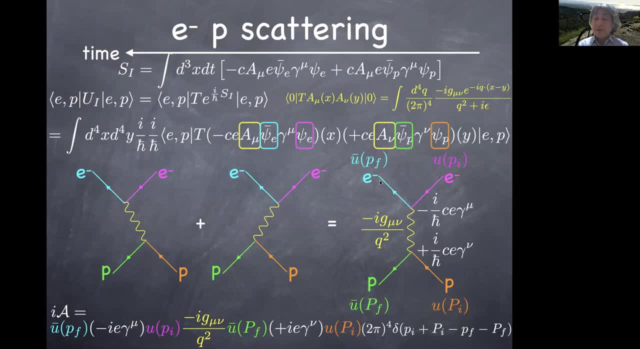 change of the full momentum between initial and final electron. So each vertex conserved full momentum, both energy and momentum. but existence of photon here, with non-zero Q squared, indicates that this is the virtual intermediate state. So that's the idea of deriving this Feynman diagram. 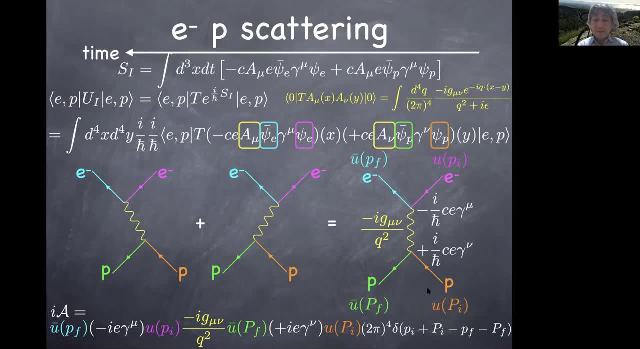 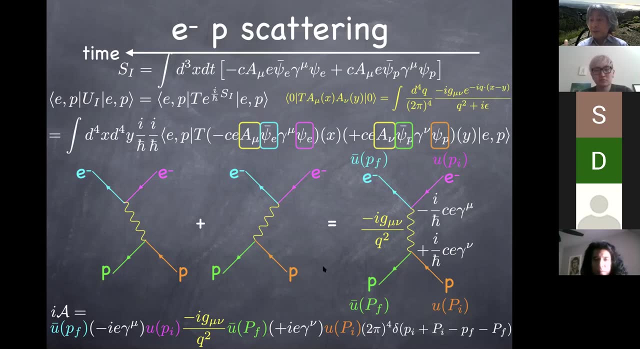 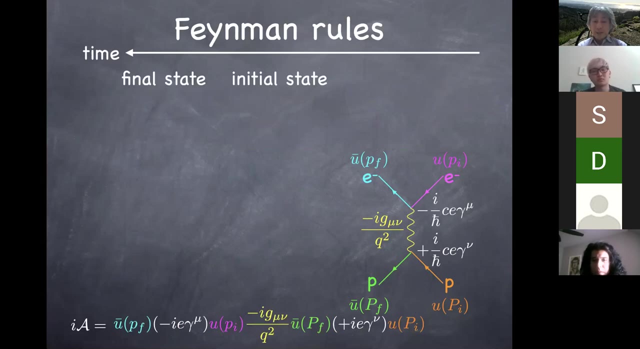 So any questions about this? You're working on this right now. I believe We went through this on Wednesday, so it's not new, But anyway, All right, So I don't see any questions. So once you know this Feynman rule, then you can immediately associate the Feynman amplitude. 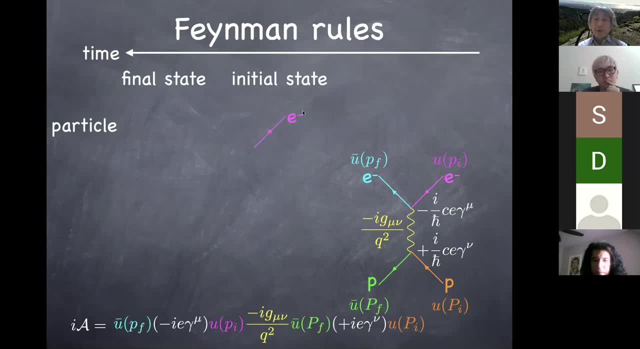 So here's the summary. So you have the initial state particle, you associate it with the positive energy solution. You have a final state particle, you associate it with the positive energy solution, with bar on it. So dagger and gamma naught. So that's how we actually got in this amplitude. 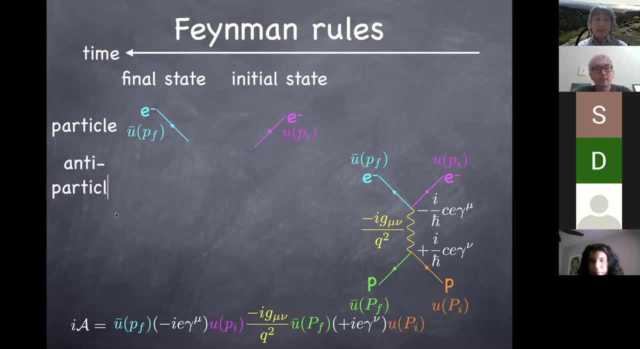 So that's actually general rule. On the other hand, if you use the, look at the antiparticle, we have to use the negative energy solution, And if you have antiparticle initial state, you use actually the negative energy solution. So that's the general rule. 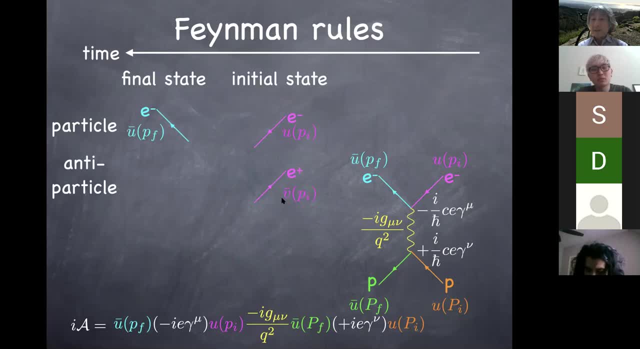 The negative energy solution with bar on it, Because it is the psi bar field that has the annihilation operator for the antiparticle. So that comes together with the negative energy solution with bar on it. So initial state particle is V bar. That's now the Feynman rule. 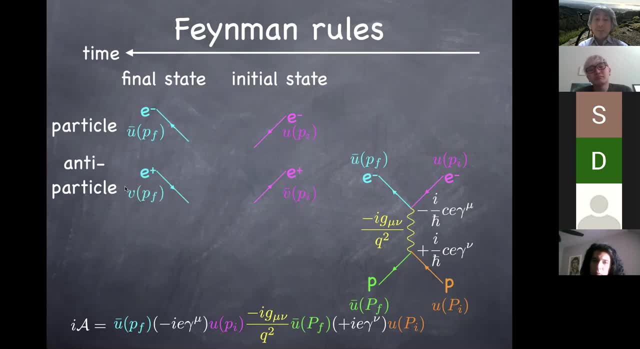 And the final state antiparticle is V instead, without bar on it. So it seems as if this is V, which corresponds to psi, And so that's why we use the cyan color here And that's why we use this backward arrow to indicate that this one for the particle. 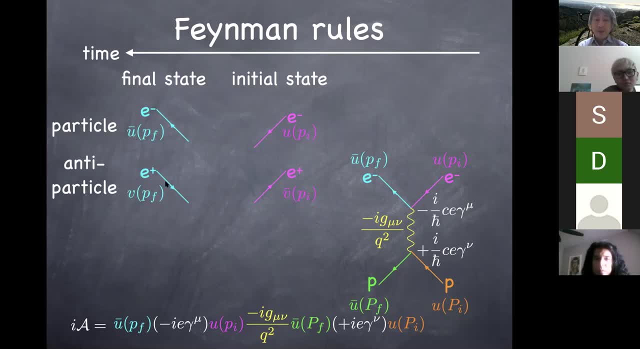 is U bar, But this one for the antiparticle is V, without bar on it, And hence the rewarded arrow. So the backward arrow in time is not meant that the antiparticle is going backwards in time. that's impossible, But it's just a mnemonic, or the way you remember. 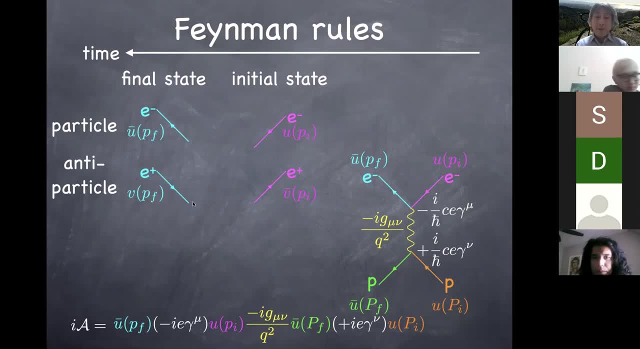 So that's why we use the backward arrow to indicate that this one for the particle is U bar. remember that the backward arrow always refers to antiparticle, forward arrow always refers to particle, And once you know which one is particle and which one is antiparticle, you know which. 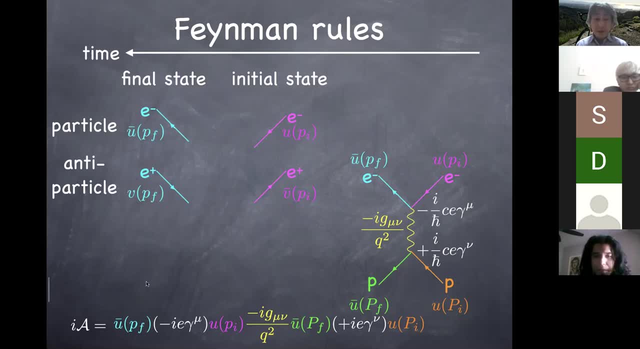 solution you're supposed to associate with initial state and final state, And we talked about the propagator for the photon, which is one of our Q squared, basically just like Klein-Gordon field, except that you have minus G menu in the numerator because the photon field has the Lorentz index. 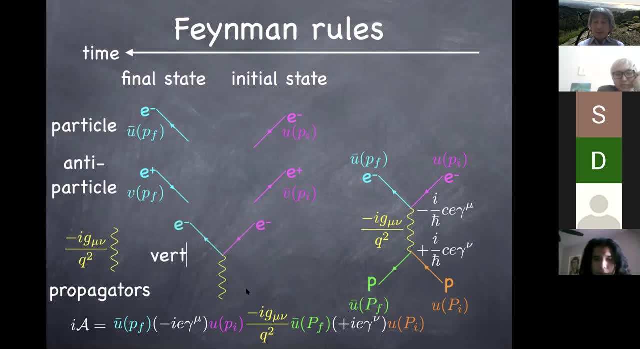 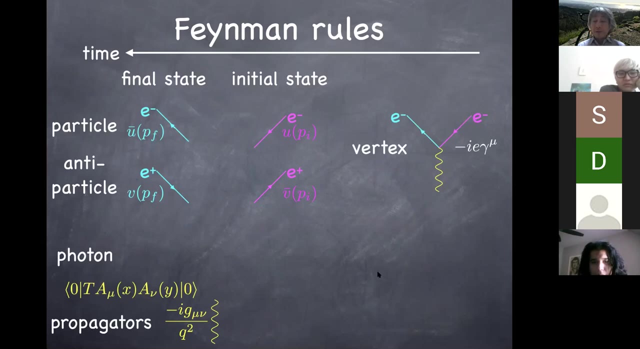 And then we talked about this vertex, which is given by minus E, gamma mu, when you set C and H bar to be one in the natural unit. And in addition, sometimes you also want to talk about photon in the initial state or final state, for example when you talk about the Compton scattering. 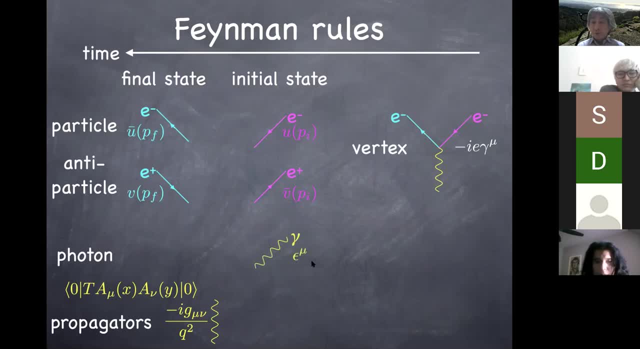 Then you associate the polarization vector for the photon, which we talked about when we quantized the electromagnetic field in Coulomb gauge, And for the final state you associate the polarization vector with complex conjugation. So for plane polarization it's real, it doesn't matter. but if you're talking about the circular, 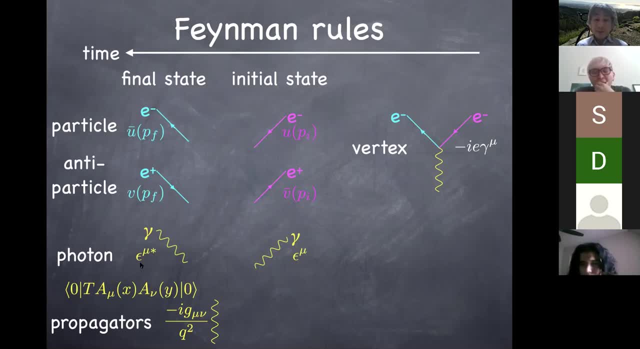 polarization. you need to be aware that you have to put this complex conjugation on it, So that's something we also talked about already about a month ago. Sometimes you also need to have a propagator for the fermion field too, And I'll show you some examples of that later on. So then, 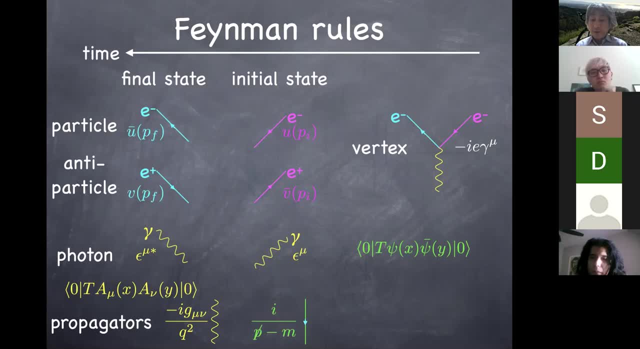 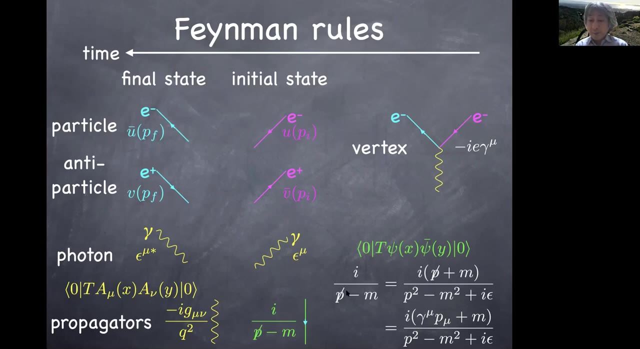 let's go back to the previous slide And you can see here we have a few points of negative randomness. We have this line for the fermion And you associate this factor as a propagator. So this p? slash is a new notation which is just meant to be gamma mu and p? mu with the Lorentz index contracted, So it's a matrix. Putting matrix downstairs sounds strange, but if you multiply p slash plus m, both in the numerator and denominator, the denominator just becomes a number. This is not a matrix anymore And this looks basically the same as the denominator. So you have this line with the fermion, you have the Type X matrix and you associate this factor as a propagator. So you have this line for the fermion And you associate this factor as a propagator. 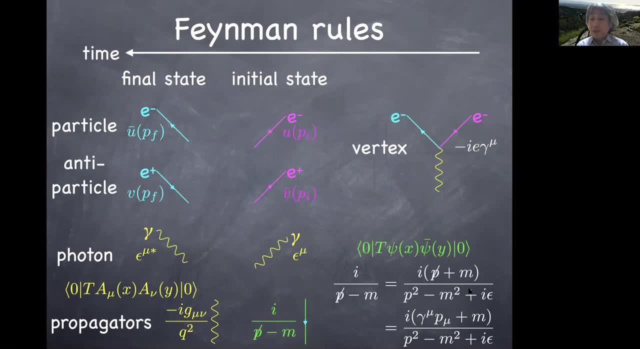 similar thing as the propagator for the Klein-Gordon field, except that you have this p slash plus n upstairs. So that is what you're going to use when you have an internal line of the fermion connecting to vertices. So that's it. So this is the Feynman rule. So in principle, if you consider any process, 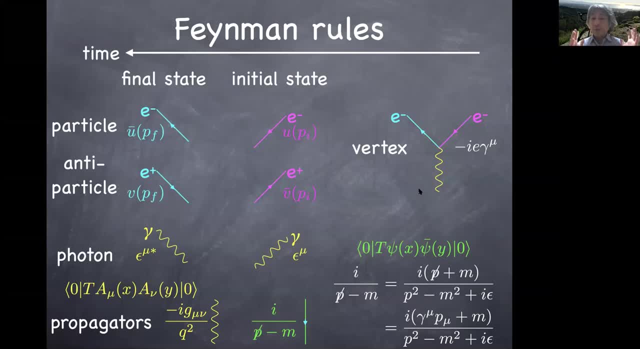 you like in quantum electrodynamics, then the first thing you do is draw as many diagrams as possible allowed by these rules And once you have a diagram, each piece of the diagram, every line and every vertex corresponds to something very specific, as you see on this slide, And you can. 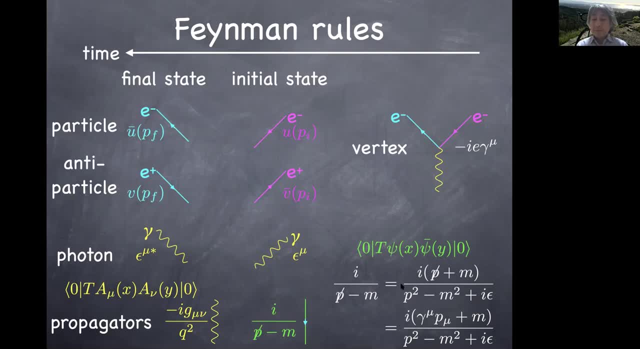 immediately write down the amplitude of that process. So that's a very, very convenient and practical way of computing processes in quantum electrodynamics, Quantum field theory, and of course we are talking about QED here as a prime example of this. 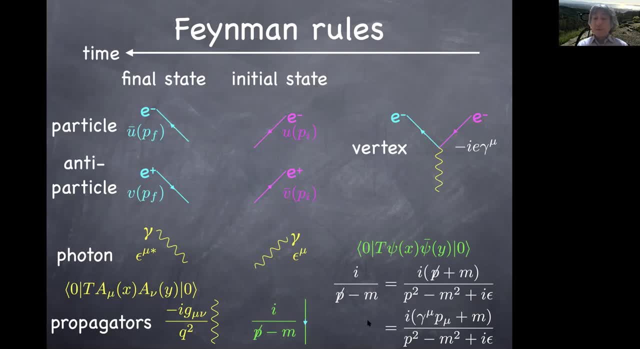 but the same technique would also work for the Schrodinger field in non-rhetoristic case. If you have some other interactions in QEFT, you can apply also the same idea. The vertex may be different depending on what theory you're looking at. Propagator may be also different if 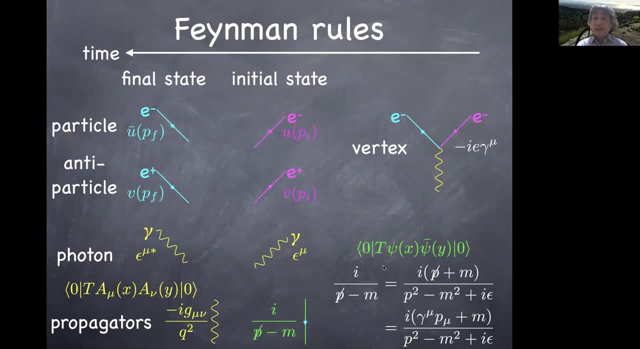 you're looking at the non-rhetoristic field theory, but the idea is always the same. You have initial states, you have non-rhetoristic fields, and you have non-rhetoristic fields. You have initial states, you have non-rhetoristic fields. So if you have non-rhetoristic fields, you have non-rhetoristic fields. 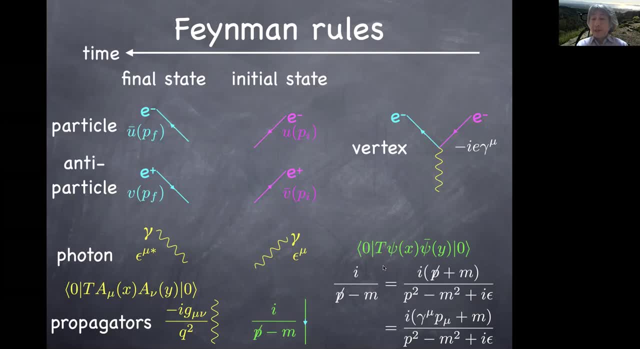 you have final states, you glue them together with the vertices. If you have an internal line, you put the propagator in there, and that's the way you can do perturbative calculation in any quantum field theory. So it's a very general idea. 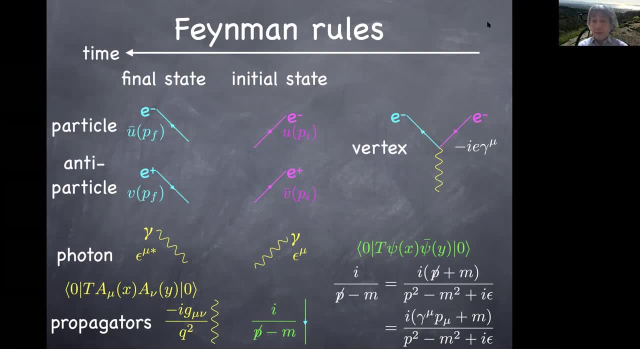 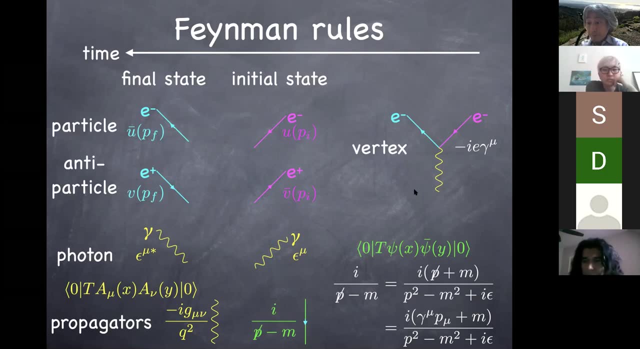 Here is a very concrete case of the quantum electrodynamics. Okay, any questions about this? Jose, are you trying to speak? No, okay, Okay, anybody else? Of course I'm- Oh, go ahead. I was just gonna ask. 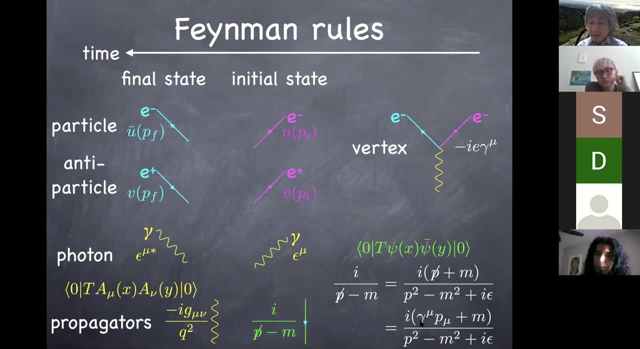 what's the particular definition of P slash again? So P slash is this gamma mu times P mu. So if you compare this line and that line, you see this P slash is the same as gamma mu, P mu And that's a matrix or an outer particle. 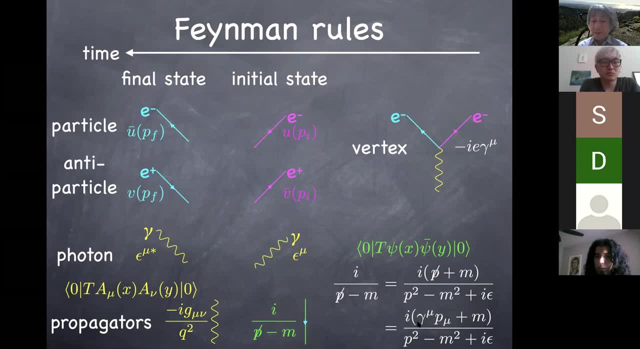 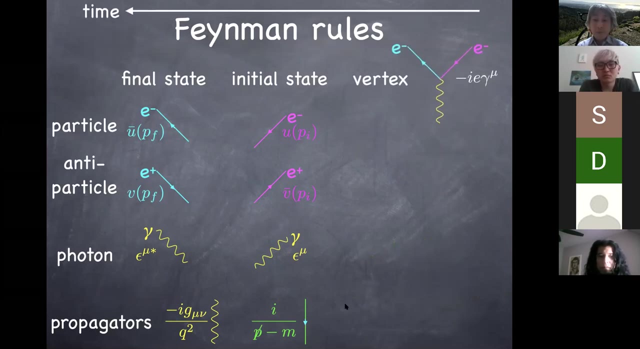 Yeah, it's a matrix. yeah, Okay, Four by four matrix, And this is a notation Feynman introduced, apparently, So he was very, very practical guy. Any other questions? Okay, So let's look at a couple of examples here. 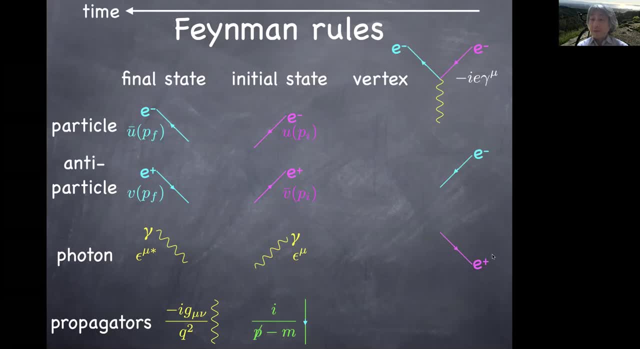 Suppose you are looking at a process where you have electron and positron in the initial state, which is the particle and antiparticle, So they can actually annihilate and disappear from the world, but instead you have energy, which is the particle and antiparticle, So they can actually annihilate and disappear from the world, but instead you have energy. 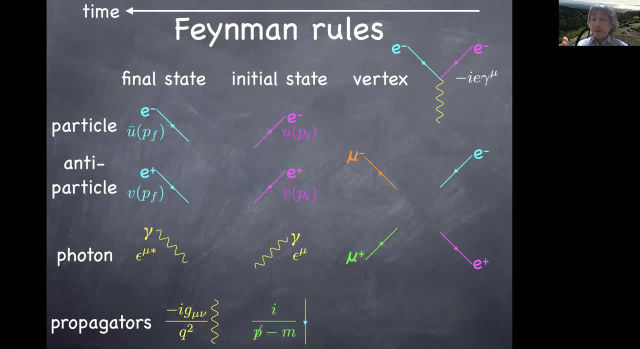 coming from this initial state And that energy might materialize into a pair of particle and antiparticle, but different kind of particle, In this case a muon, And if you don't know what muon is, it is actually a particle that actually shines on you like a thousands of them going through your body every second. 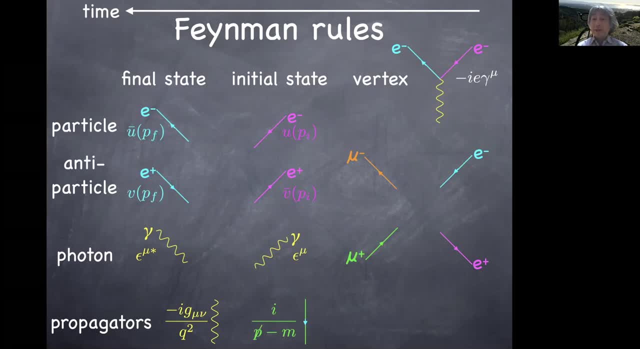 actually It's a cosmic gray particle And so this is actually just a heavy version of the electrons, as far as we can tell, About 200 times heavier than the electrons. It's not that heavy than electron with exactly the same properties. It's a Dirac particle spin one half same charge. 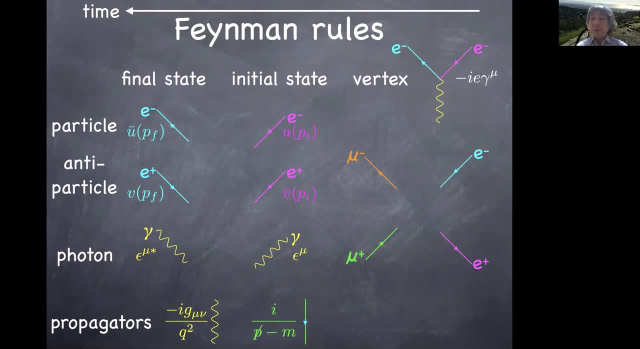 I don't know why such a particle had to exist in nature. When the muons discovered in cosmic ray, a famous Nobel laureate physicist, Isidore Isidore Rabi, actually complained. Who ordered that? Because apparently there was no particular reason why such a particle had to exist. 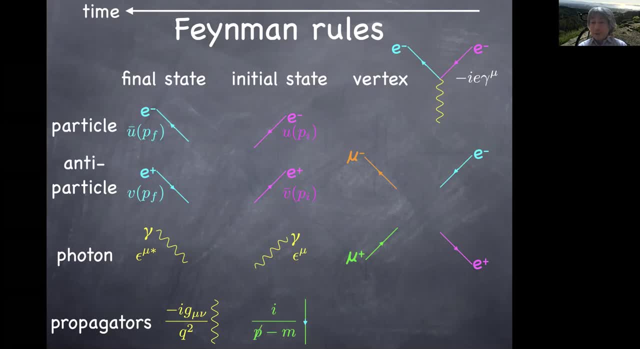 But it does exist and we can make them using this process, Namely that when electron and positron come together using this vertex in QED, it can go into this virtual photon and because muon has the same charge as electron, it has exactly the same Feynman vertex. 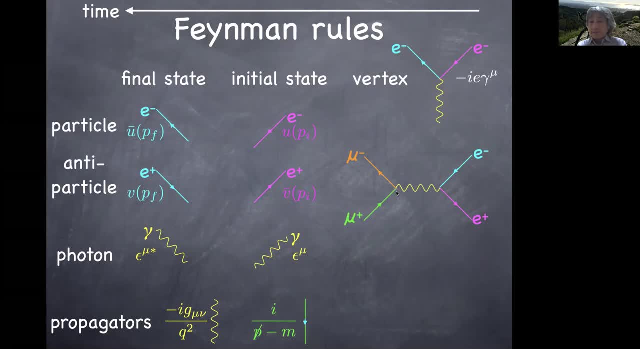 so you can put them together using this vertex. and there is the Feynman diagram. So this is the process where electron and positron annihilate and briefly becomes a virtual photon, and this virtual photon now materializes into a real particle- muon and anti-muon- And we're going to actually compute this. 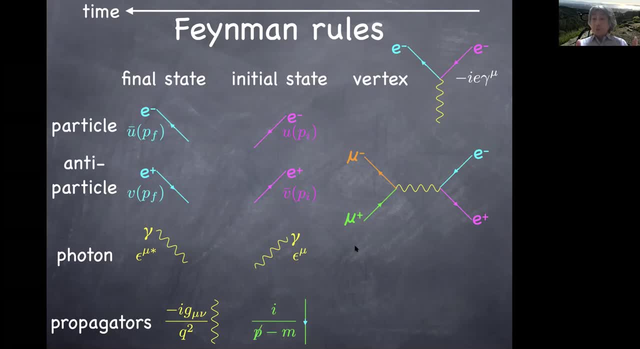 Feynman amplitude explicitly later on. but I hope you see that this diagram can exist And the minute you see this diagram you can immediately associate these different factors of the Feynman rules into this diagram and immediately write down this amplitude. 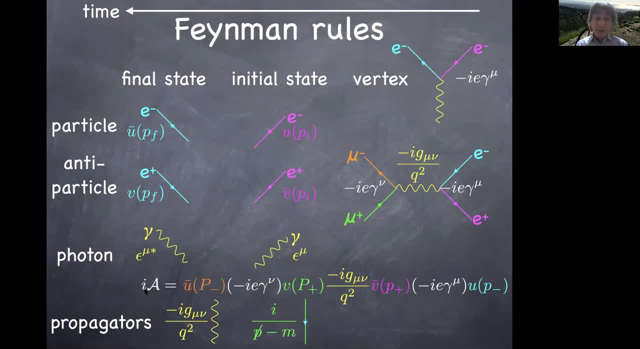 So amplitude A is typically coming with factor of i, for historical reasons, and then you see that you have initial state electron. so, using this Feynman rule, I associate a positive energy solution with its full momentum p-, indicating this is for e-. 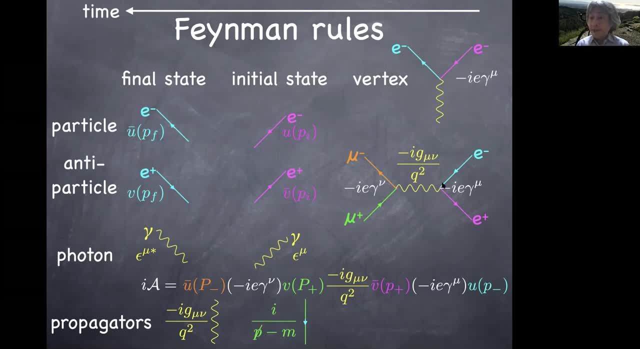 And then, following the arrow, next comes this vertex minus iu, gamma, mu, and for this initial state, antiparticle, I associate this, the negative energy solution, with bar on it with full momentum, P plus for E plus. So that takes care of this side of the diagram. 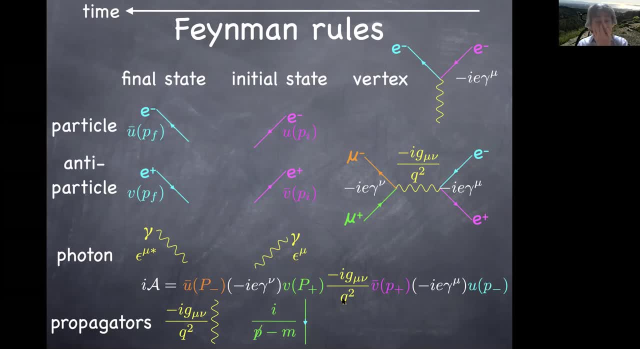 Then comes this propagator in yellow. That's this factor here. And then again we follow the arrow for the mu one side. So you start with final state antiparticle. That's the negative energy solution with full momentum capital P plus. 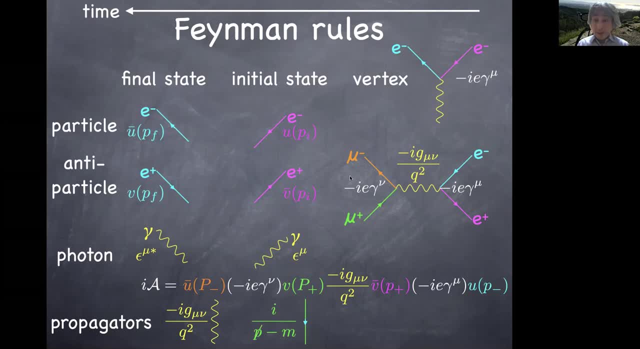 Here is this: Feynman-Vutex minus I, gamma nu, And the final state particle is associated with the positive energy solution with bar on it for the full momentum capital P minus for mu minus, And that's it. So you can see that once you draw a diagram like this, 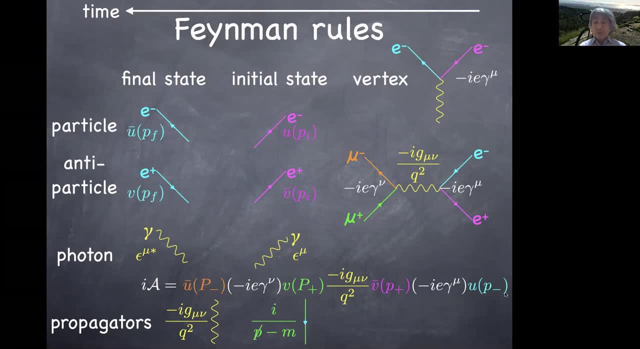 you can immediately write down the amplitude for that process And you know everything in here. You we have solved the Dirac equation. You have the solution in some of the earlier slides And also for the negative energy solution. you know what the gamma matrices are. 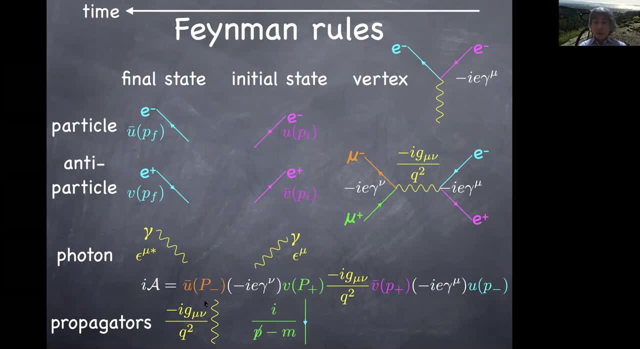 And Q squared is the full momentum of this virtual photon. So you know everything in this factor. You can just plug them in and out comes the Feynman amplitude. Then you can actually use the formula. I'm gonna tell you in a couple of minutes. 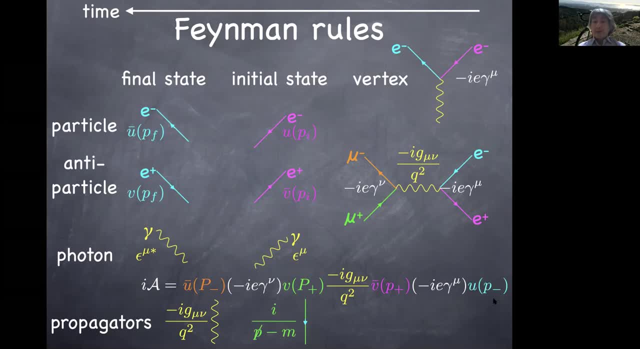 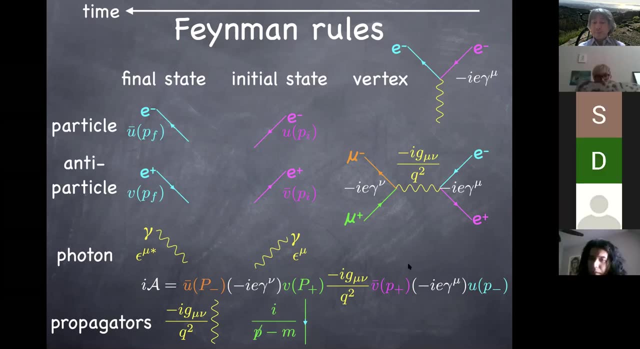 to compute the cross section for this process. So that's the idea. So it's actually very simple, very intuitive, very practical, And then, in principle, you guys can now compute any process you like In QED. In practice it can get pretty tedious. 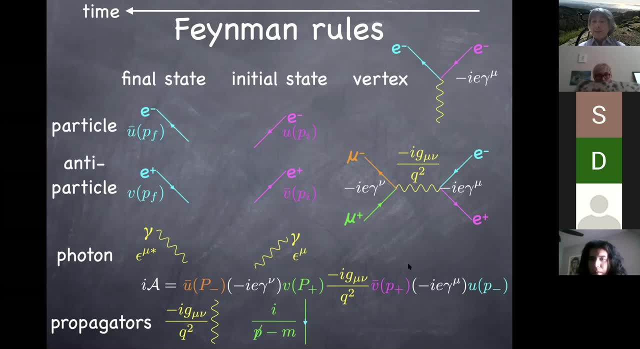 And I can tell you more examples in this class today. But anyway, the idea is just this And that's everything you need to know about how to do the perturbation theory in QED. Any questions here In terms of actually drawing the diagrams? 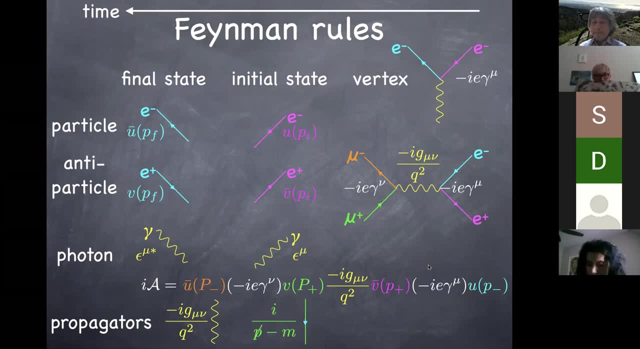 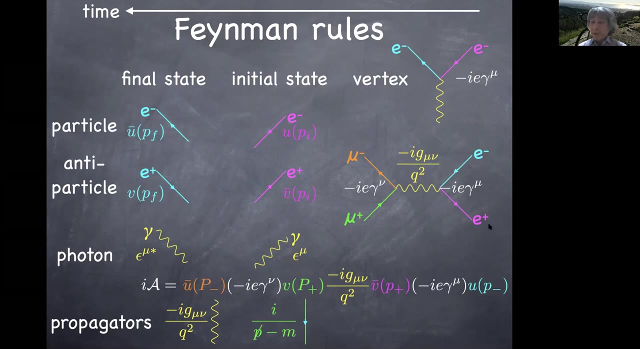 are there particular things besides just having vertices and the arrows being consistent? Like: how is a conservation of energy or momentum enforced in these diagrams? Yeah, so in this case the electron full momentum and positron full momentum are added together at this vertex. 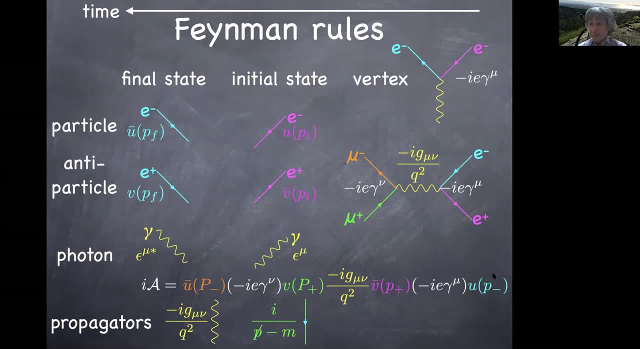 So the full momentum of this virtual photon Q mu is P minus plus P plus. And then this Q mu full momentum turns into the full momentum of capital P minus plus capital P plus. So, as a result, P minus plus, P plus is the Q mu. 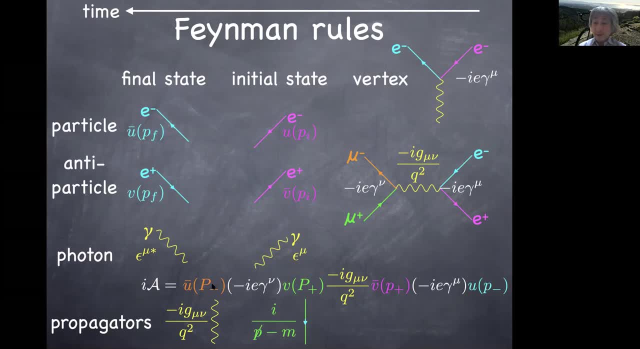 And Q mu is the capital P plus plus capital P minus. So at the end of the day, little p minus plus, little p plus is capital P plus and capital P minus, And that's the overall full momentum conservation of this process, right. 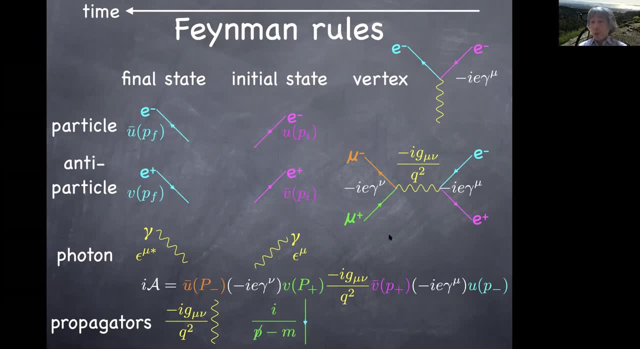 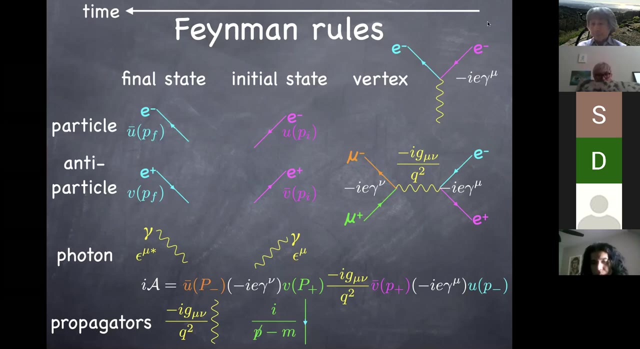 So as long as you conserve full momentum at every vertices, overall full momentum conservation comes out automatically. So I didn't write full momentum delta function here, but that is satisfied. once you actually glue them together in a consistent fashion, Does that answer the question? 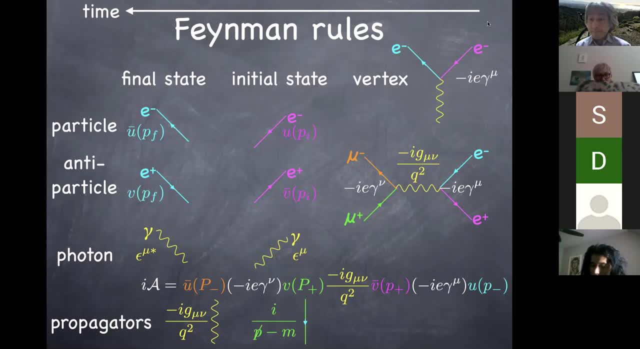 Yeah, yeah, Any other questions here? So, as you see more, oh, go ahead. go ahead, Anna. Oh well, I was just gonna ask, I just wanted to make sure. so, like we have to write these factors in order as determined by like the arrows. 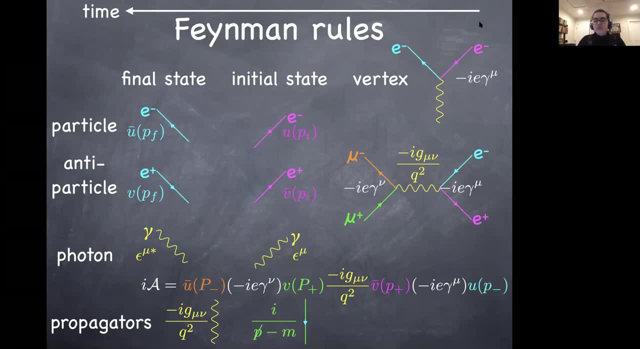 you were saying: or does it not matter? No, no, you do, wanna write arrows, So the arrows indicate which line is meant to be particle, which line is meant to be antiparticle. So again, I'm following this convention that time flows from right to left. 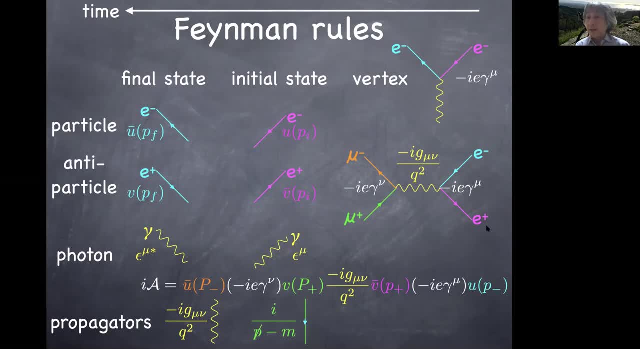 So you see immediately that this E minus and E plus are in initial states, because that's the rightmost lines. But given these arrows, I can tell that this is electron, this is positron. So in practice you don't color lines. 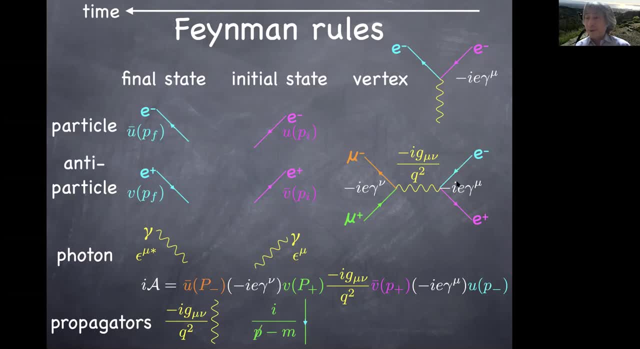 So you know they are all black and white, but you can still tell that this is particle, this is antiparticle, because you can draw these arrows consistently And arrows don't clash, Electron comes in. You cannot let electron annihilate with electron. 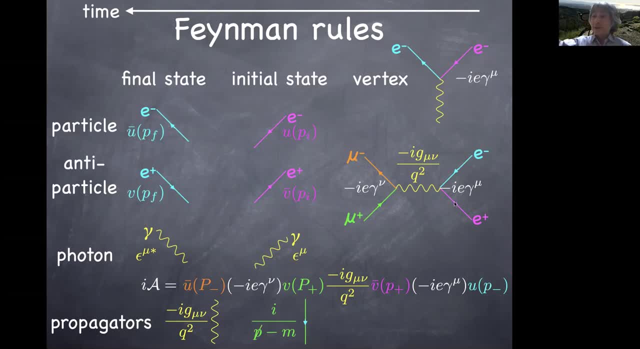 because then the arrows clash. So if you consistently assign arrows so that they flow constantly, then you don't need to. don't make a mistake, Like you know, pretending two electrons can annihilate into photon. that's of course impossible, But electron and positron can annihilate. 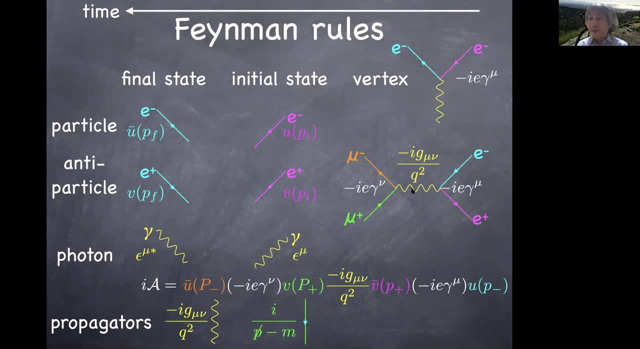 because arrows don't clash and have a consistent final vertex to go to this virtual photon. I guess I was also wondering, like just for the ordering of the terms and the like amplitude expression, if we have to follow the arrows like you did. That's right, Right. 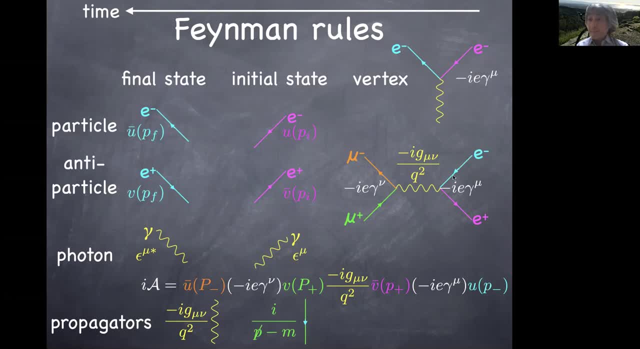 So you always begin with the arrow coming into the diagram- and that's this U spinner here, and then vertex, and end with the arrow going out of the diagram. Of course, arrow going out in this case is still initial state in terms of time. 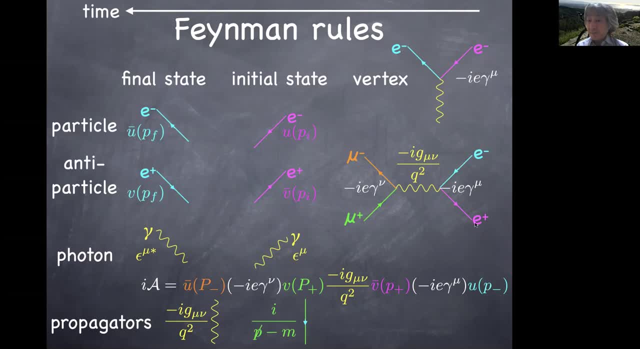 but in terms of diagram, this is the arrow that goes out of the diagram and that comes last. So you always follow the line of arrows for the fermions: You start with incoming arrow, You end with outgoing arrow and keep everything in between. 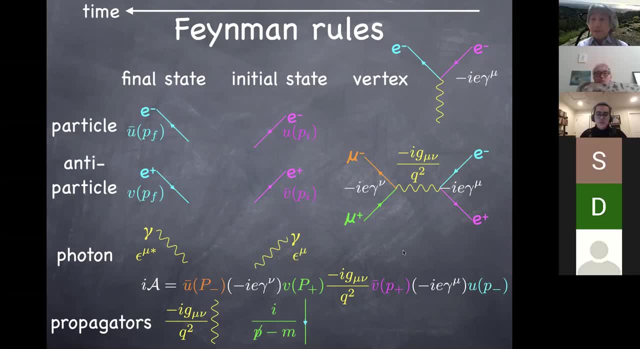 Does that answer your question? Yeah, And I hope it makes better sense when you actually look at the next example of E plus, E minus annihilating into two photons. So here this is a different process. Again, you have electron and positron in initial state. 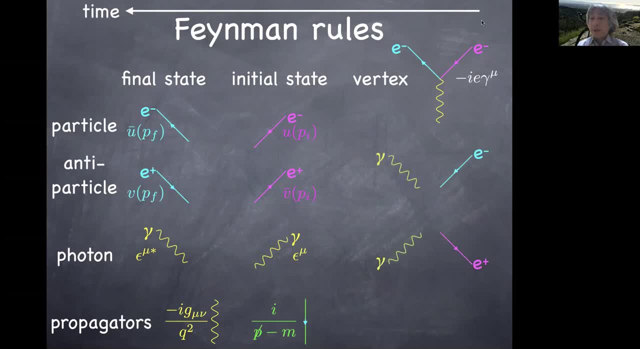 I have two photons in the final state and now I need to figure out how to glue them together into a consistent diagram. So first thing is that this electron now is connected to the positron using this internal fermion line. This is the first time you see it in use. 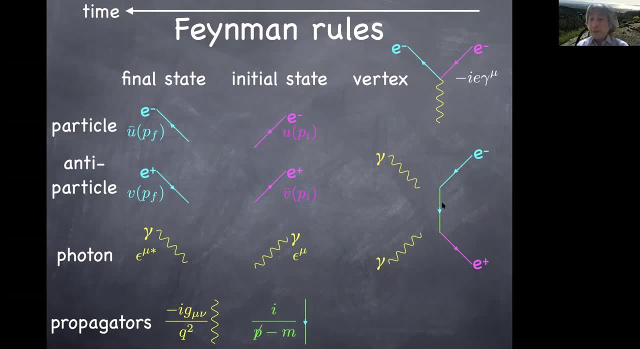 of this fermion propagator And by using this internal fermion line, I can bring this photon to this diagram and using this Feynman vertex, over. here again, you see that arrows are flowing consistently along this solid lines. The second photon can be also brought together into this diagram using another Feynman vertex. 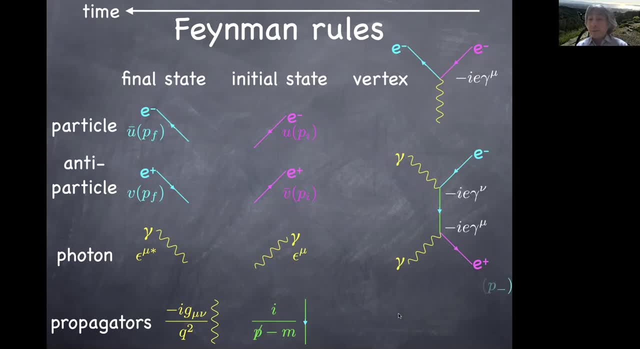 And then again you can immediately write down the Feynman amplitude by associating all the factors we talked about. So again, following this arrow of the fermions, you start with line with arrow coming into the diagram. So that's a positive energy solution for the electron. 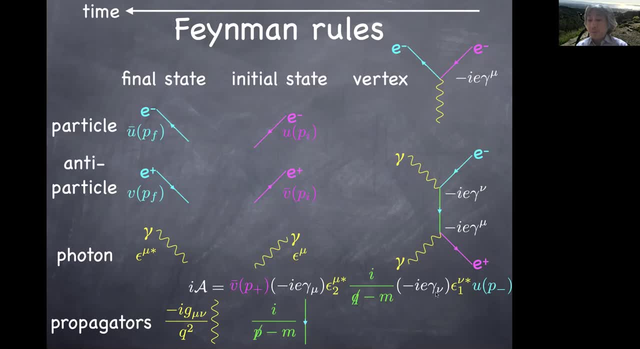 Then I have this vertex minus i e gamma nu. But here I have to also associate this photon with the final state polarization vector star. So that's the first photon polarization vector star whose Lorentz index nu is contracted with this Lorentz index nu of this Feynman vertex gamma nu. 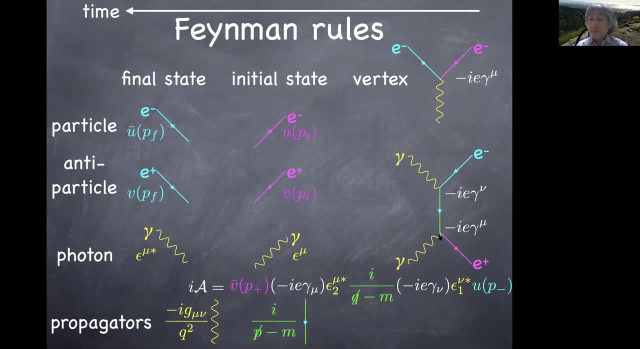 So that's this vertex over here. And then comes the fermion propagator, which we talked about two slides ago. So this is the matrix downstairs, But you know it's actually a matrix upstairs instead. It's just a shorthand notation for it to basically save writing on the slides. 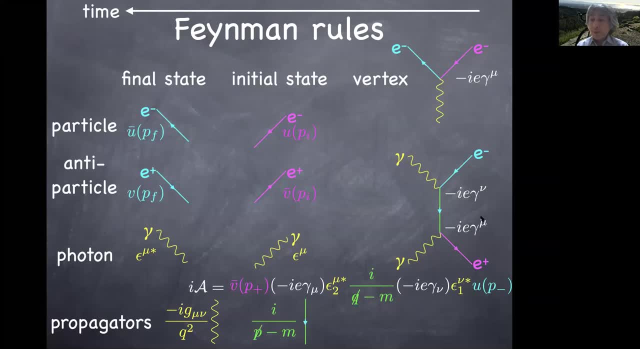 Then comes the second vertex minus i, e, gamma, nu, where nu Lorentz index is again contracted with this polarization vector of the final state photon, Second photon here with complex conjugation And you end with this outgoing atom. This is the outgoing arrow from the diagram for the positron in initial state. 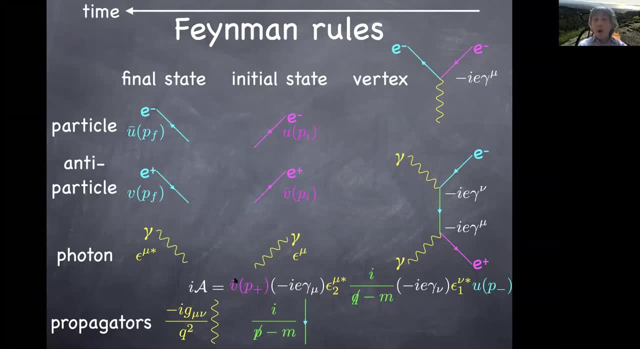 So that would correspond to the negative energy solution with bar on it. So if you follow the fermion line, you always start with u or v and you always end up with u bar or v bar. And that makes sense because, after all, everything here is a four by four matrix. 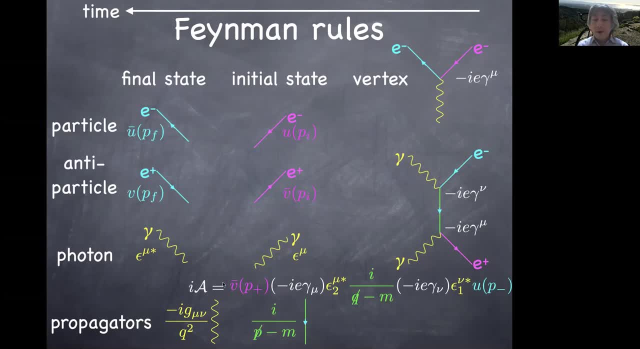 U is the four component column vector. V, bar is the four component row vector. So that's the way I have the row vector, bunch of matrices in between and upper column vector, And so that whole thing becomes a number and that's what we want for. a amplitude is supposed to be a complex number, as we all know from the quantum mechanics. 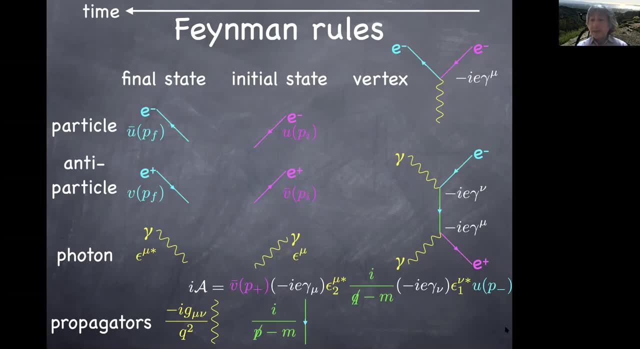 So that's the way it works. So again, exactly the same ideas. The only new ingredient here is that I used this internal fermion line with this propagator, and this is the point I would also like say, like a quote, another one verse by the notebook: 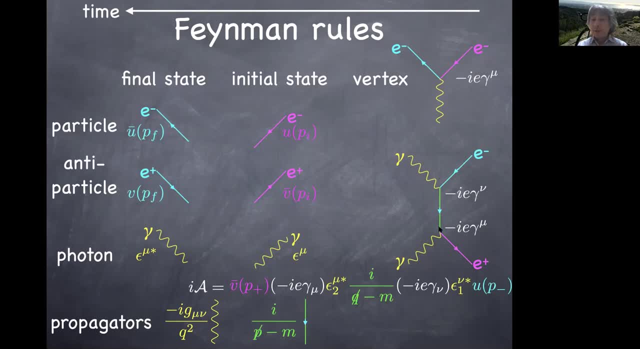 when we are going to write, actually reduce theposition, write down therefore, a first, second, third or transcendental inch that we could also apply in abroad class, And you know, is the same thing with the stick. So the next: we add a overall vector única price value. 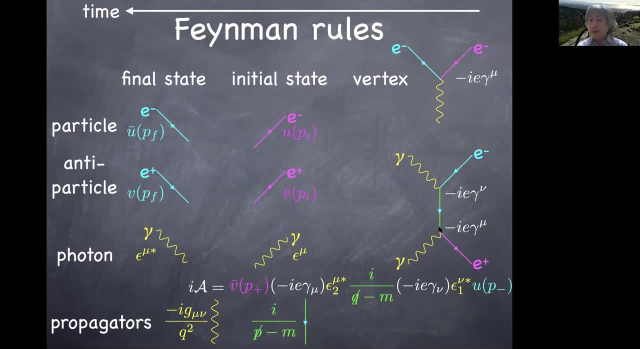 actually answer some of the questions I think Sahil asked before. So why don't we put label of positron electron on each line instead of drawing these arrows? So, remembering that this Feynman diagram actually sums already two time ordering between two vertices, it could be the case that 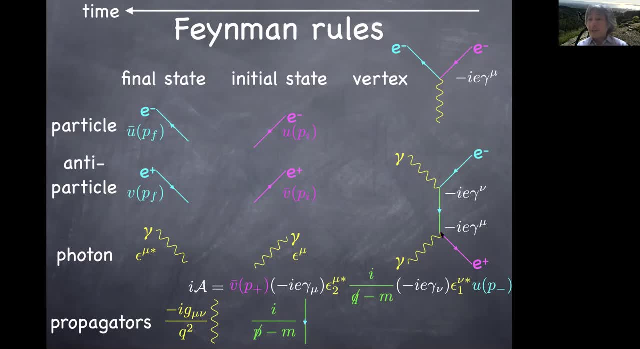 this vertex is early. this vertex is late. So in that case you're talking about the process that electron emits a photon first and then keep going as an electron then annihilates together with the positron to become another photon. So then this line is an electron. But if you think 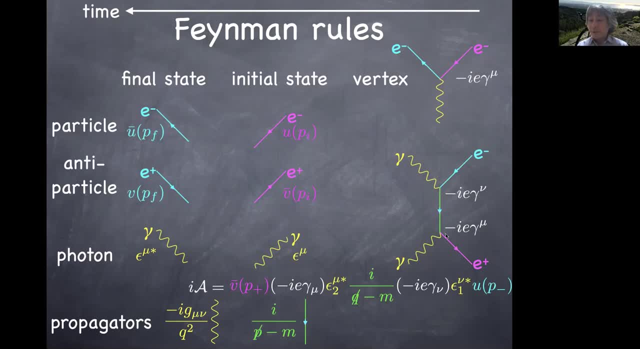 about the other time ordering. let's say this happens first, then this is the case where positron comes in, emits a photon, then it has to keep going as a positron instead and that positron annihilates, with this electron to become. 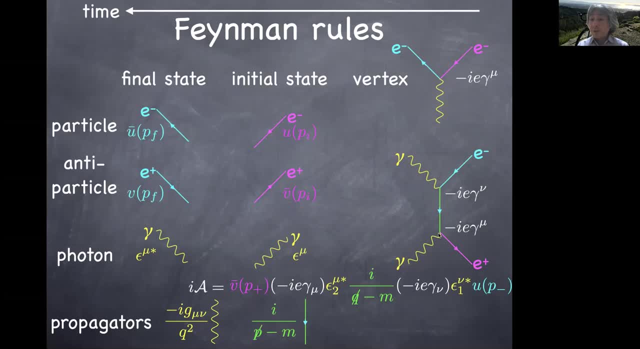 this the other photon. So this green line actually represents both possibilities at once. because it's a time order product of Dirac field and Dirac field bar. It has both possibilities in it. So I cannot label this line as an electron or positron, because the answer is: well, it depends. 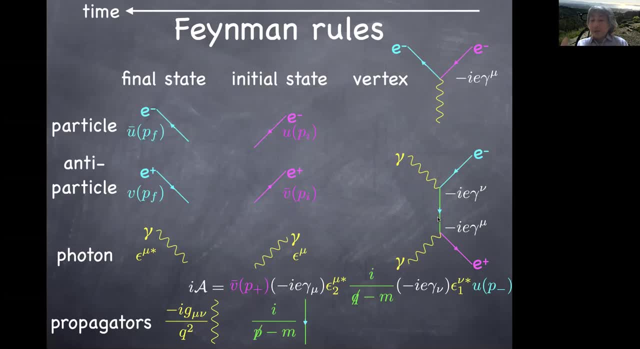 Depending on which time ordering that is. this line may be electron, this may be a positron, or maybe a positron, But the beauty of the Feynman diagram is that you don't have to worry about it. This is just the internal line. You associate this propagator. 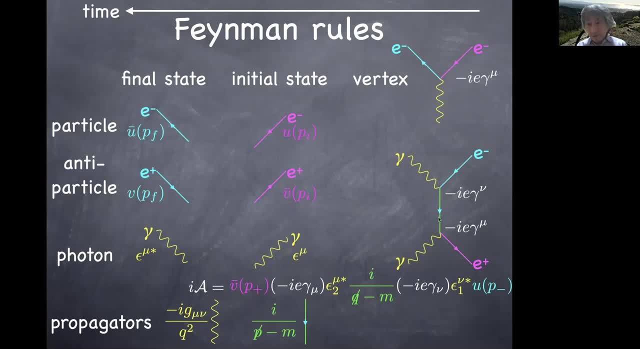 And you just keep drawing these arrows consistently. You don't need to ask the question: is this an electron or a positron? It's both one or the other that it doesn't matter. So that's the answer to was this here? actually, I'm not totally sure. 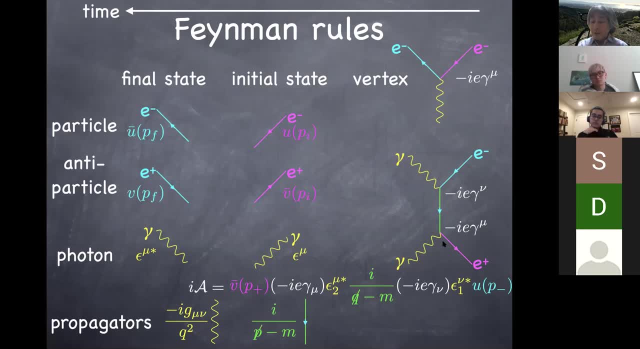 Dr Hau, Dr Hau, Dr Hau. either as electron or positron, specifically, but instead relying on these arrows. for that reason, Arrows are consistent, but which lines electron? which lines the positron? is not clear for internal lines. 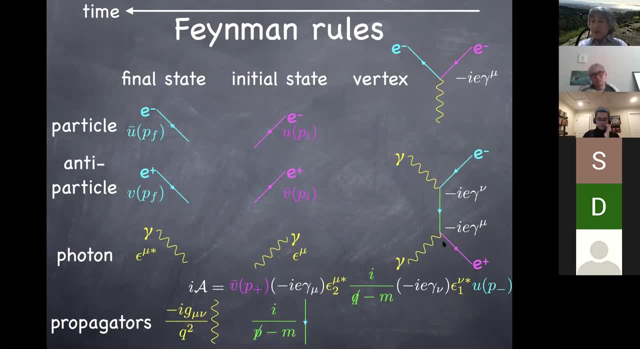 for the propagators. They are clear for the external lines. they're not clear for the internal lines because of this business of time ordering. but it doesn't matter, You don't have to worry about it, because all you need is the consistent arrows. 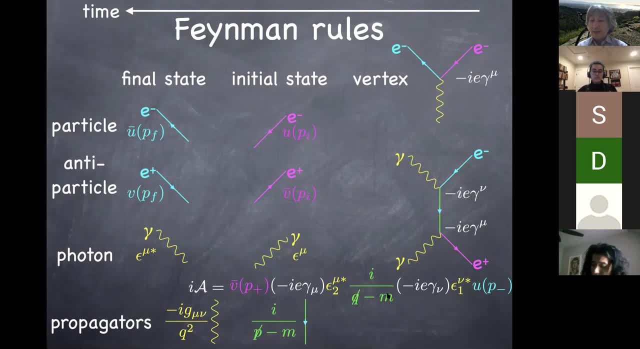 and you associate this propagator for every internal line in a consistent fashion. Okay, any questions about this. It's okay, Professor, Go ahead, Is it Andrew? Yeah, what is it? I'm a little confused about what is it on the? 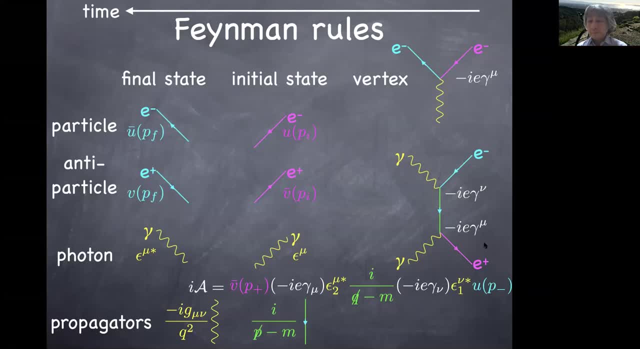 on the vertex factors in the amplitude. What is it you? what is it like? can you go over again why you forward the indices on the gamma matrices? Yeah, so this and new has to be contracted with the polarisation vector which you associate for the final state, photon right. 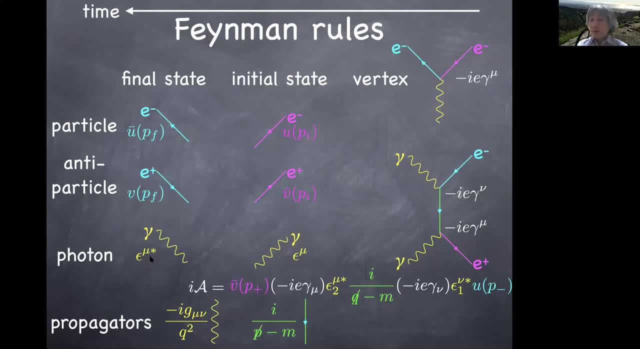 And to contract to indices. one of them has to be upper index, Another one has to be lower way index to make low end invariant contraction. Okay, yep, Duca, So that's why I move this upper index to a lower index, so that I can contract the index mu. 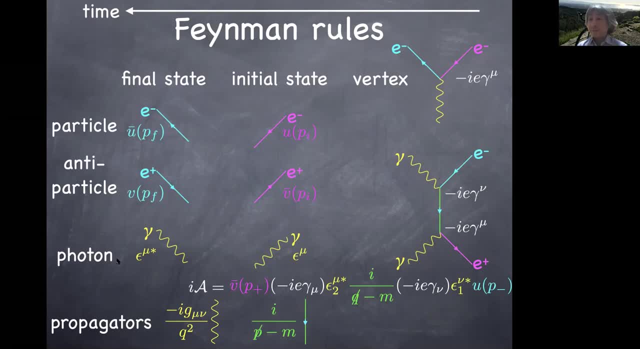 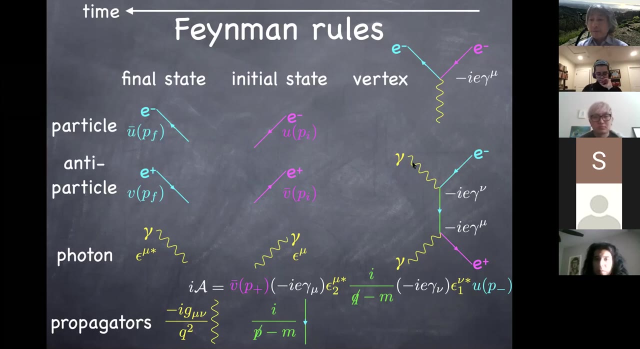 between this Feynman vertex and this polarization vector. Okay, All right, thank you. Okay. Any other questions on this example? Okay, But it turns out that for this process, this diagram is not it, There's another diagram. Because when you actually go back and think about 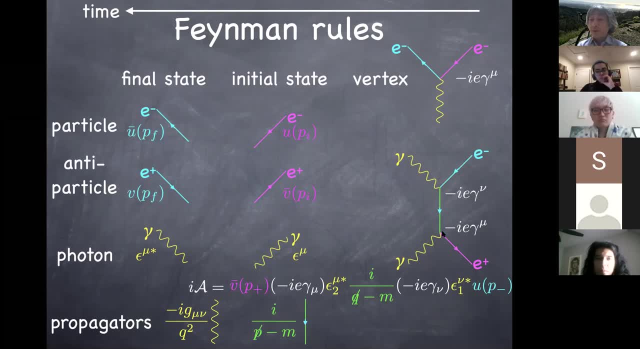 how this diagram came about from the time-dependent perturbation theory. I have a mu operator here. I have a mu operator here, But a mu operator can create either this photon or that photon. They have different momentum. So there is another diagram where you interchange two photons. 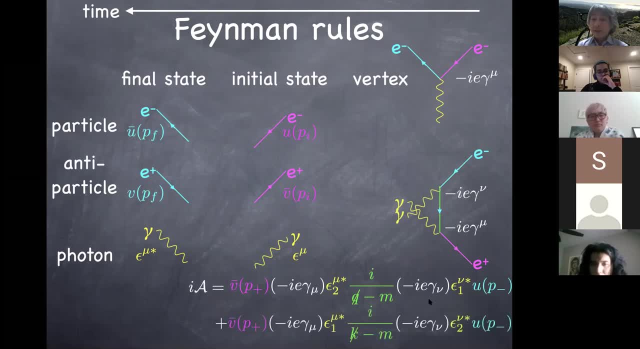 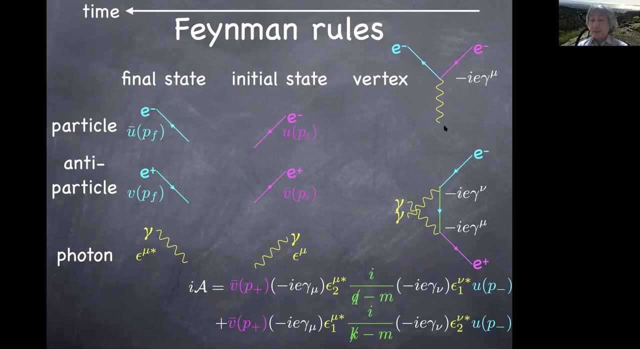 and you have to sum it. So this is sort of something that looks similar to the symmetrization of the wave function you have seen done in quantum mechanics class And, of course, in QFT. as I emphasized already, there's no ambiguity. 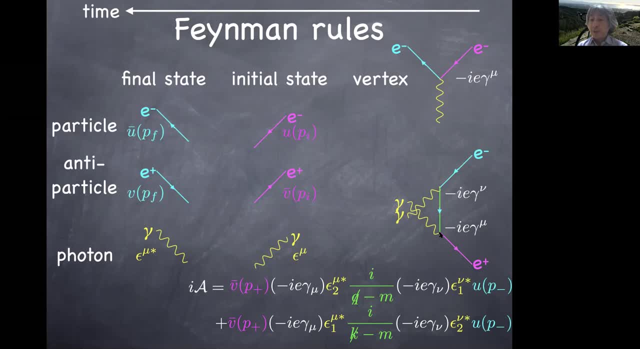 There's no choice because this comes from time-dependent perturbation theory. with a mu operator creating a photon, You automatically get these two amplitudes from the time-dependent perturbation theory. So this symmetrization is automatic. But when you draw Feynman diagrams, 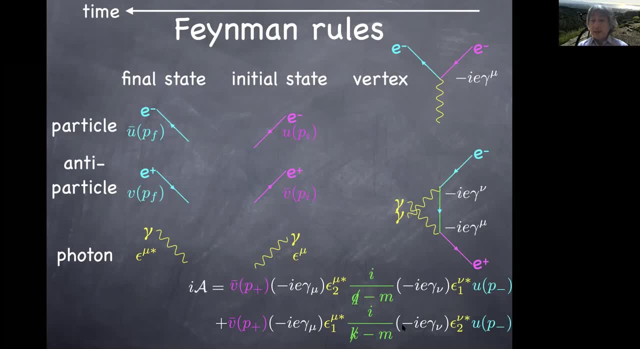 you have to draw two diagrams for each of this process And for each diagram. for example, this internal line for the electron line would have different full momentum. So here I denoted one of them with full momentum Q, another one with full momentum K. 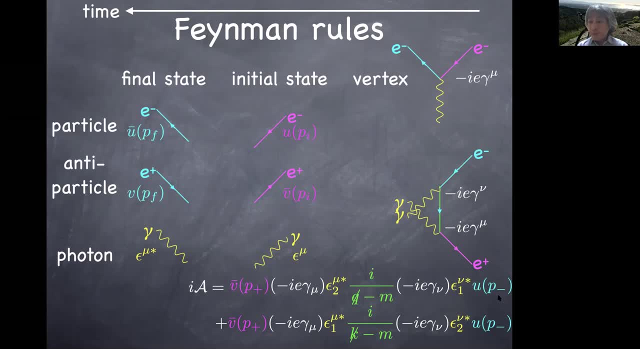 because the full momentum Q would be P minus minus the momentum of the first photon. That would be this full momentum Q, But for this diagram I interchanged them. So this momentum in the green line would be P minus for the electron full momentum minus the photon momentum. 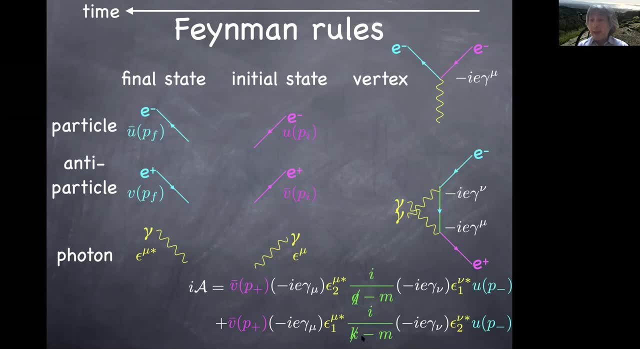 for the second photon And that is the full momentum K for this internal line. So you know again. the idea is exactly the same. You conserve full momentum at each vertices, but because this epsilon one and epsilon two refer to a photon of different full momentum, 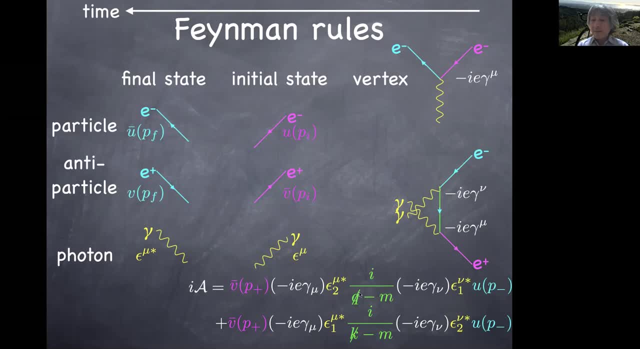 So, depending on which diagram you're looking at, you again assign full momentum for this internal line by carefully looking at this sequence of events of P minus emitting a photon and you subtract that full momentum to figure out the full momentum of the internal line. 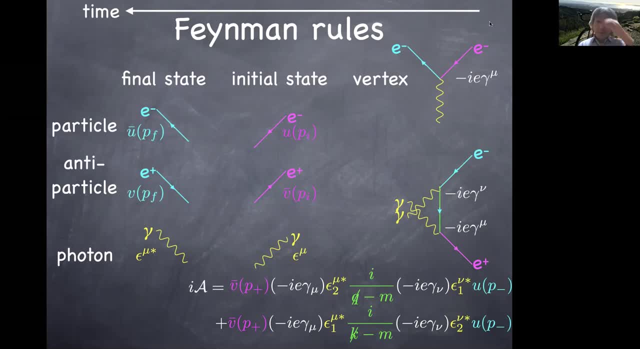 and so on and so forth. So that's the idea of: if you have a photon, you can do this. So that's the idea of if you have a photon, you can do this. P plus E minus annihilation into two photons. 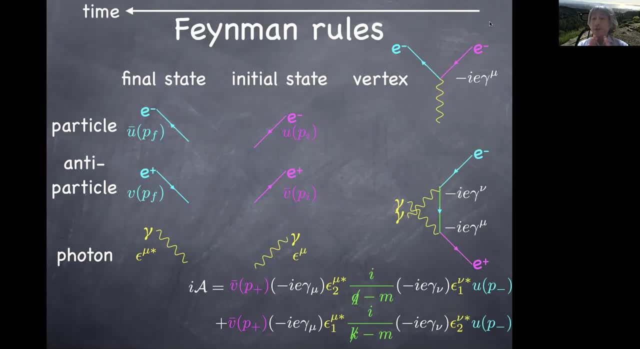 And then we emphasize here that this is the process you could never ever have talked about in quantum mechanics, Because, as I mentioned earlier, quantum mechanics relies on Schrodinger wave function. Schrodinger wave function has fixed number of arguments. You can never talk about particles being destroyed. 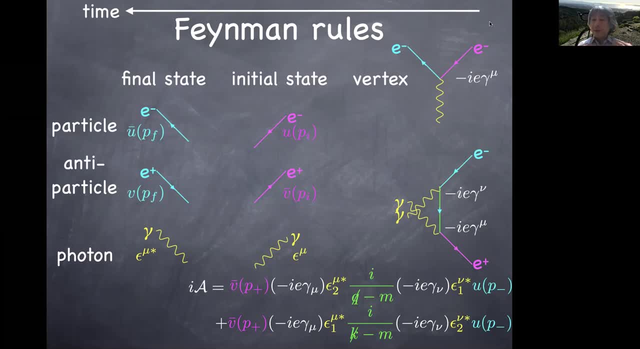 or appearing, but this is an example where electron and positron inertial state just totally disappear from the world and then instead you see two photons appearing. So particles annihilate, particles get created, and that's a process we can talk about in quantum field theory. 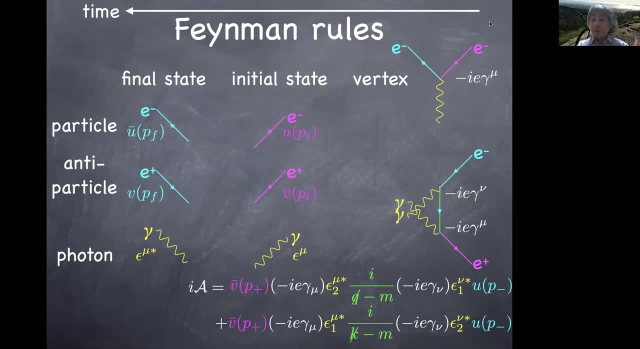 but never, ever in quantum mechanics. And now you see that in action. So this is an advertisement I did long time ago at the beginning of the class, and now you see this in action. This is the first time you're looking at the process. 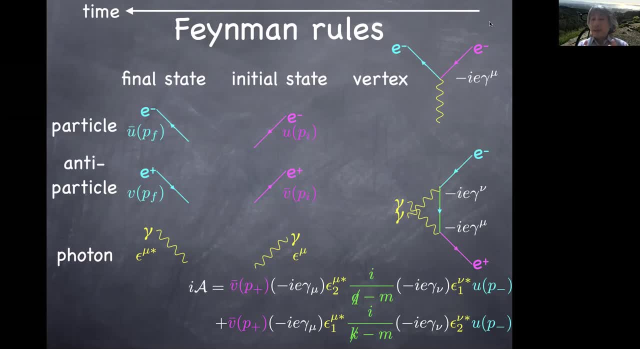 where matter, particle can really disappear from the universe. and it does happen. And that's the example actually you have seen in some of the slides I've talked to you, like the anti-plot on coming into the photographic plate on the Berkeley Hills from Bevatron accelerator. 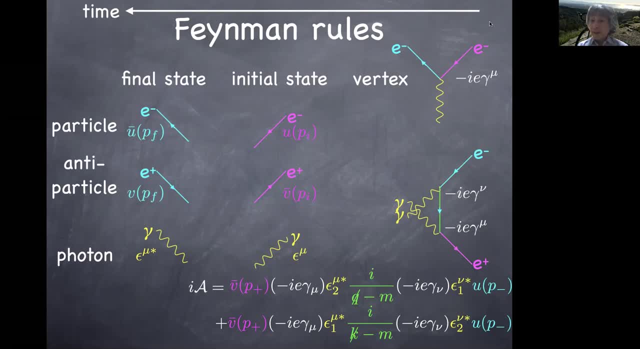 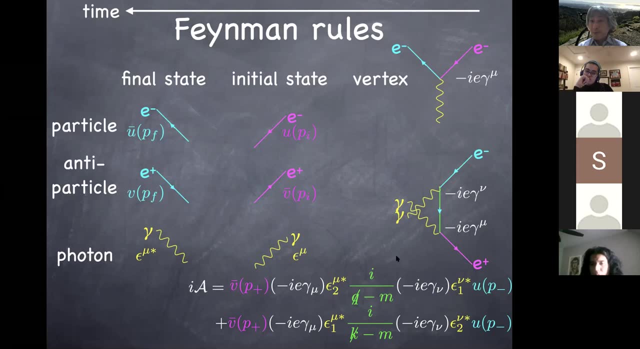 which annihilate into a bunch of other particles, and you have seen a picture of it. Now you see how that is described theoretically in quantum field theory. Okay, any questions about this? I just had a quick question about the conservation. So you'd mentioned previously the propagator. 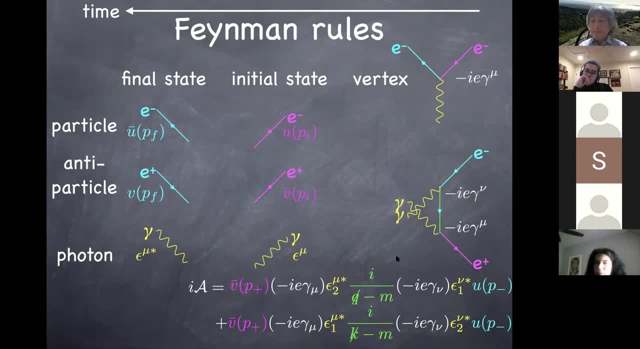 when a virtual photon does not preserve energy or momentum. Right, In this case, our four momenta are conserved at each vertex. So I guess I just see some sort of inconsistency. Yeah, yeah, So I realized that's confusing because I'm using the word conservation. 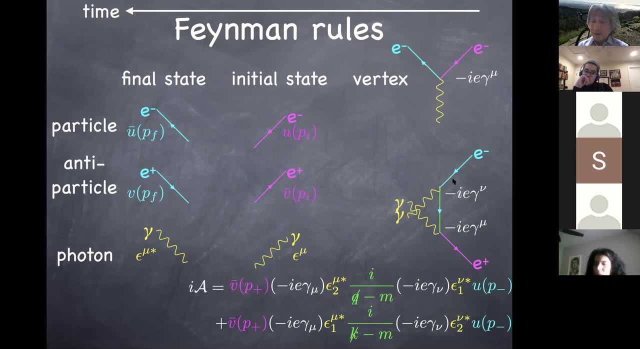 in actually two different ways, So I apologize for this. So in this example, electron emits a photon, and full momentum of this green internal electron is indeed the difference between initial state electron minus energy of the photon you emitted. So this vertex conserves all four components of momentum. 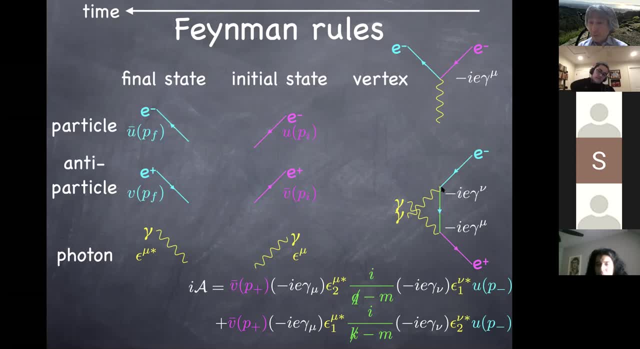 namely energy and spatial momentum. So full momentum is conserved at this vertex And when you do the formal problem, that conservation comes out automatically. Okay, are automatically from the spatial integral. But the full momentum of this electron doesn't square to electron mass squared. So the energy of the electron here is not the momentum squared plus. 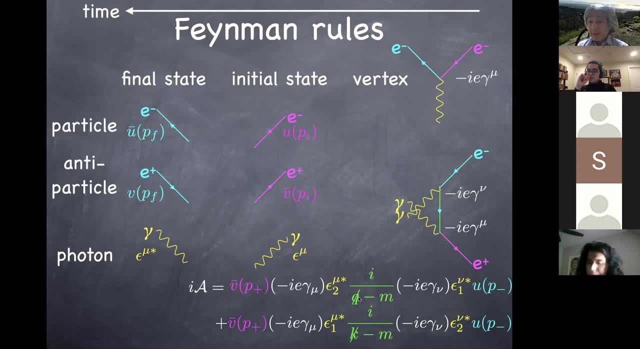 m squared, square root. So that's what I meant: that internal line doesn't conserve momentum, It doesn't have the right energy for a given spatial momentum. So maybe I should have used a different word here, that when you actually have this internal line, full momentum is conserved. 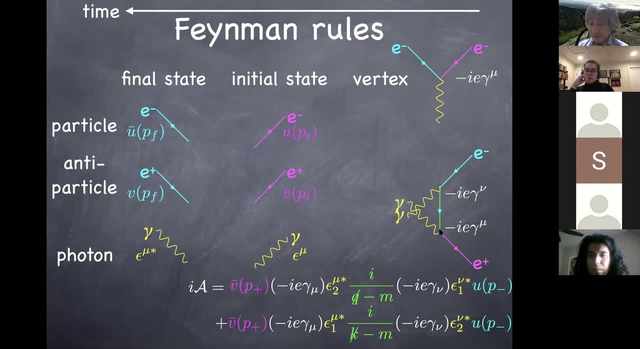 but you get wrong: full momentum for the electron, because energy and momentum don't satisfy the usual rule that energy has to be square root of momentum squared plus m squared. So instead of saying this line doesn't conserve energy and momentum, I should have said, probably, that this: 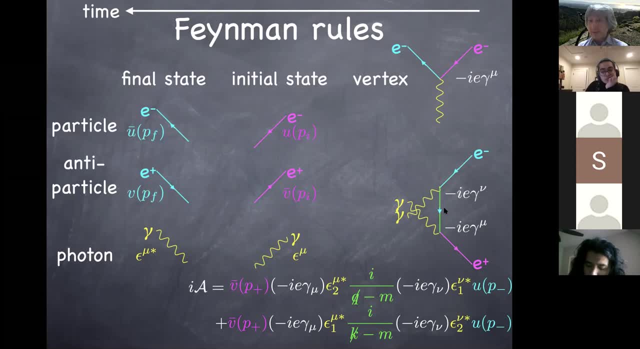 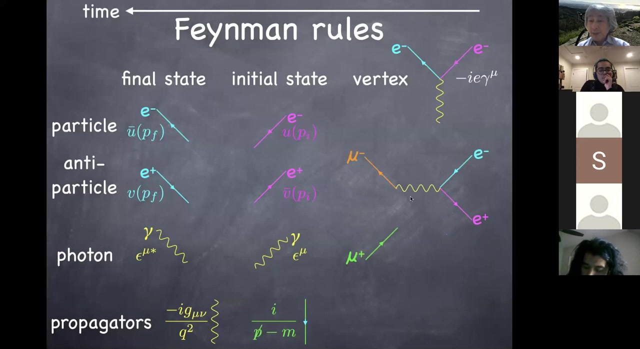 has the wrong energy and momentum And that's the virtual electron. And if you go back a couple of slides when we talked about electron-positron annihilation, and that's also the wrong full momentum for the photon. so electron-positron come in, muon, antimuon go out. you glue them together and this full momentum. 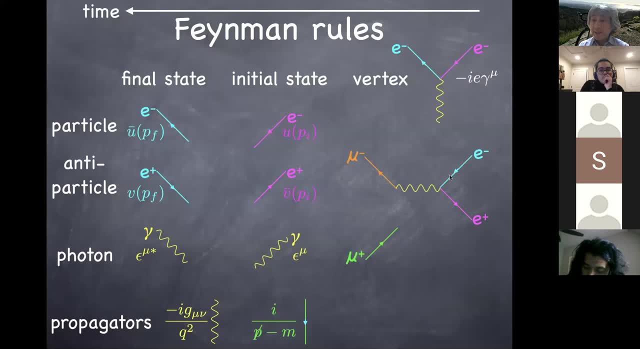 of the photon is conserved in the sense that it is the sum of full momentum of electron-positron. it is the wrong for momentum, If you actually look at this incentive momentum frame, that electron and positron come head on with the opposite momenta, So the spatial momentum cancels. 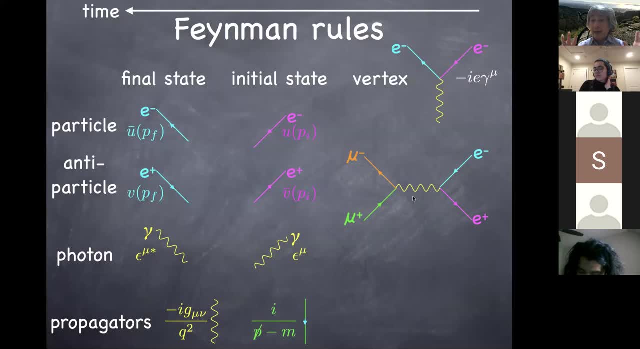 but energy. sums up, So this photon has energy but no momentum. So again, that's the wrong energy for a given momentum, which is zero in this case, because energy is not zero. So that's the situation with the virtual particle or internal lines. So in terms of Feynman diagrams, every 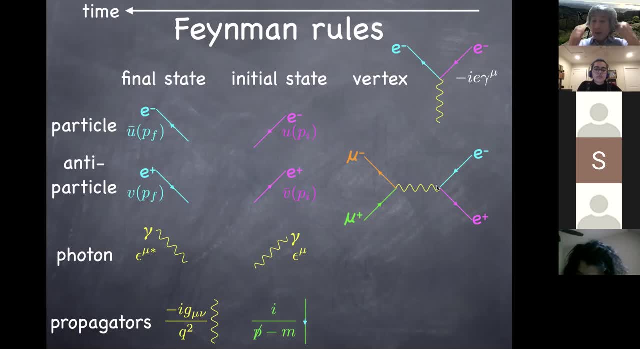 vertex conserves for momenta, but internal lines from that conserved for momenta are wrong for momenta for that particle because the energy is wrong. It's not the right energy for a given momentum for this particle And that's the case of the virtual particle And that corresponds to this. 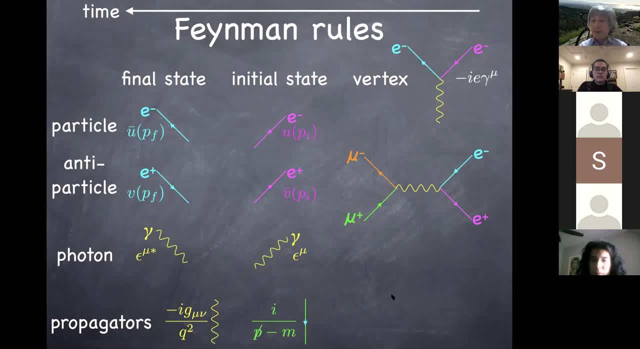 intermediacy state we talked about in Rayleigh scattering some time ago. So I'm sorry for this confusing terminology, but did I clarify this question? Yeah, yeah, So since it's a virtual particle, it doesn't obey the standard dispersion relation we normally have for a particle with some 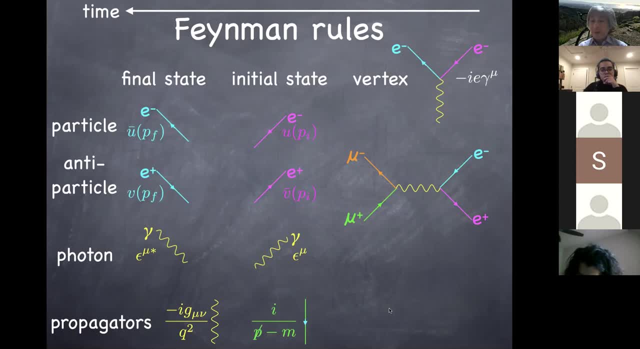 given mass or momenta. That's exactly right, Thank you. Thank you, Right. And so when that energy momentum satisfies the usual relation, energy squared minus momentum squared is m squared. then we say the particle is on-shell. The virtual particles have wrong relationship between energy and momentum. 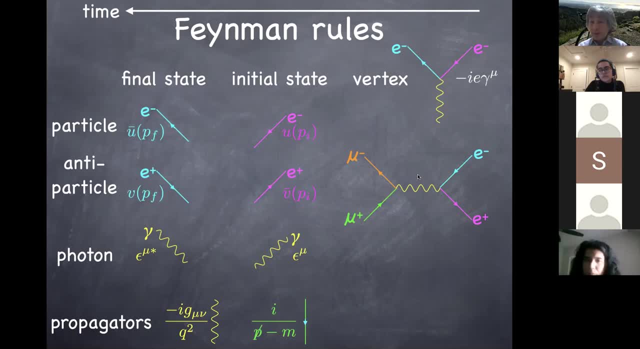 Energy squared and momentum squared is not m squared. Then we say the particle is off-shell. So being on-shell is the right relationship between energy and momentum. Being off-shell is the wrong relationship between energy and momentum. And virtual particles are said to be off-shell. 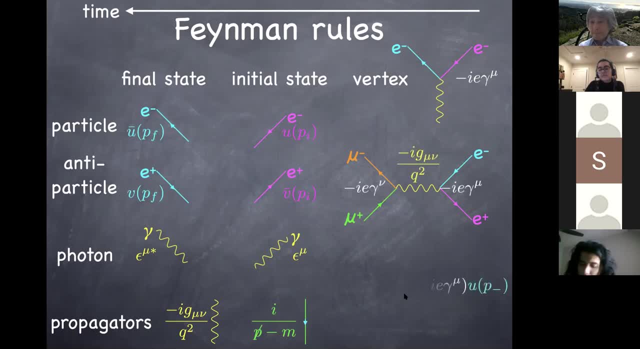 because of that. Okay, So going back to this slide. So here we talked about these two different Feynman amplitudes, like this: And when you have a process where you have to interchange two fermions, as you can easily imagine, you actually get a relative minus sign. Again, there's no ambiguity. 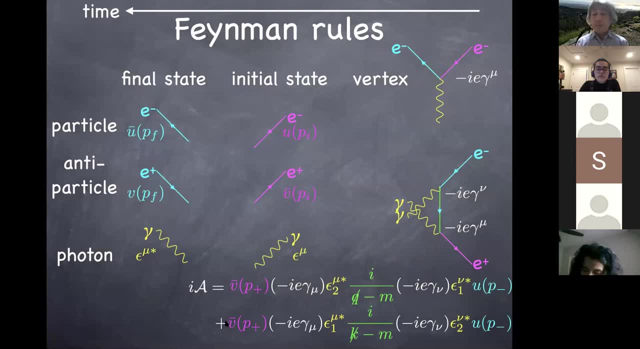 If you follow through the timing-dependent perturbation theory with operators, that minus sign comes out automatically, because it's QFD, not quantum mechanics. You don't impose it, It's automatic. But in terms of Feynman diagrams, you still do have to draw two diagrams by two. 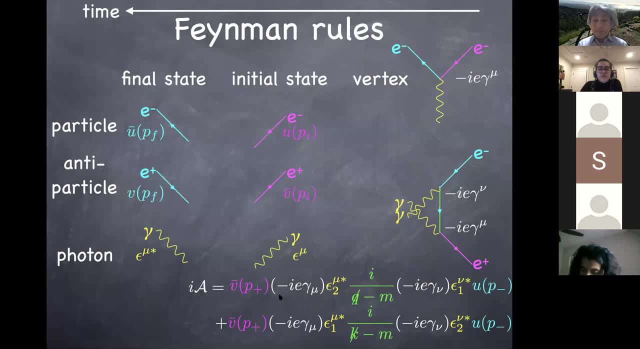 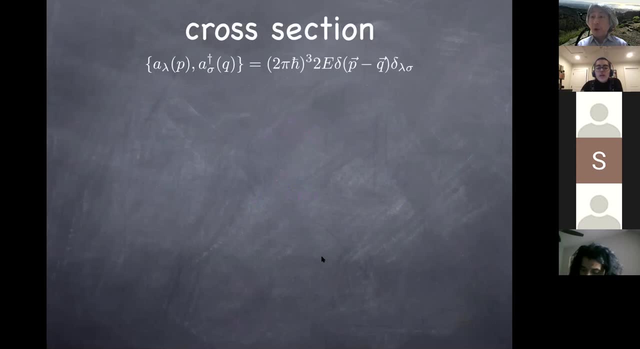 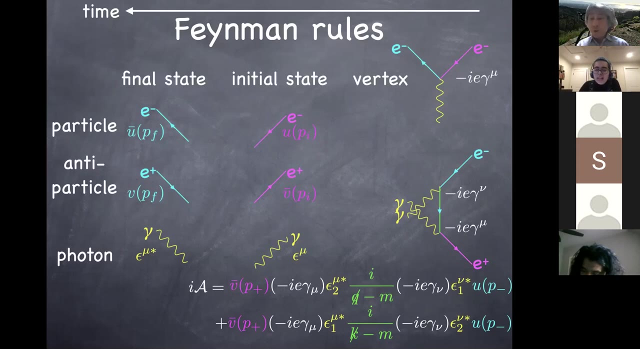 amplitudes and put the relative minus sign in between. So that's the basic idea. Okay, So now that we know how to, Oh, go ahead. I just have one question, which is maybe silly, but like if we want to describe this. 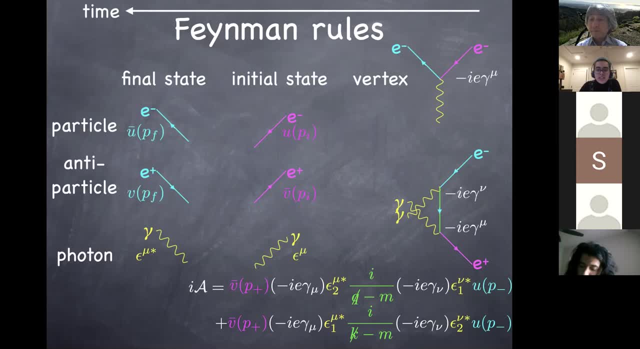 process of an electron and a positron annihilating and creating a photon. why is it not sufficient just to have one of our vertex, I guess? why do we have these two photons instead of just one? That's a good question. Yeah, So, as I said, there are no silly questions. 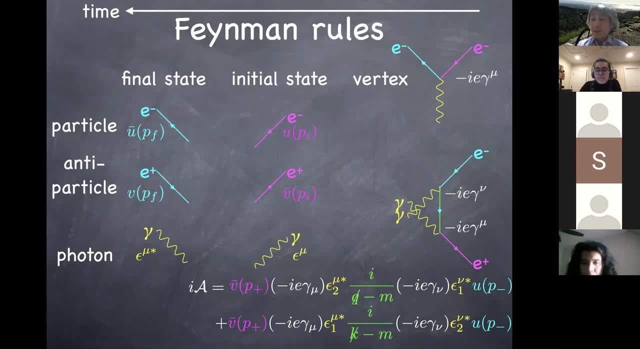 So you can ask the question: why cannot electron and positron annihilate into a single photon? So electron and photon, let's imagine. So. if one is a photon, let's imagine that both of them are at rest. then electron for momentum is mc squared for the energy, and zero momentum because it's at rest. 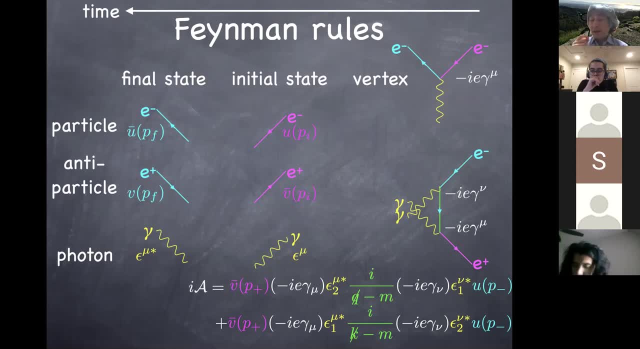 So if you put together electron and positron, TOTAL energy is 2 mc squared and TOTAL momentum is zero. But for the photon the energy has to be the same as momentum times speed of light. So it doesn't satisfy again the correct equation. It's the same as momentum times speed of light. So it doesn't satisfy again the correct equation. 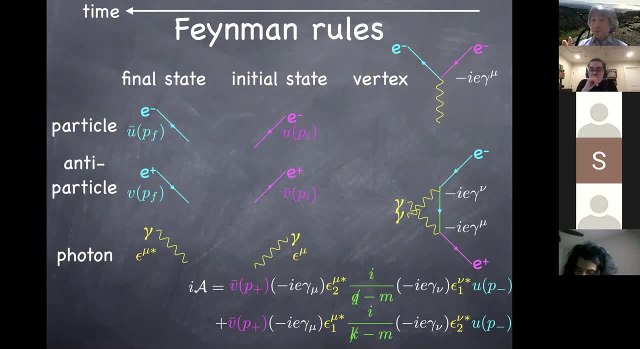 dispersion relation. So if the photon is virtual, like in the case of e plus, e minus, going to virtual photon, and mu plus, mu minus, you can go to single photon, but that's not a real photon. Therefore it cannot exist in a final state. It is allowed to exist only with an uncertain principle. 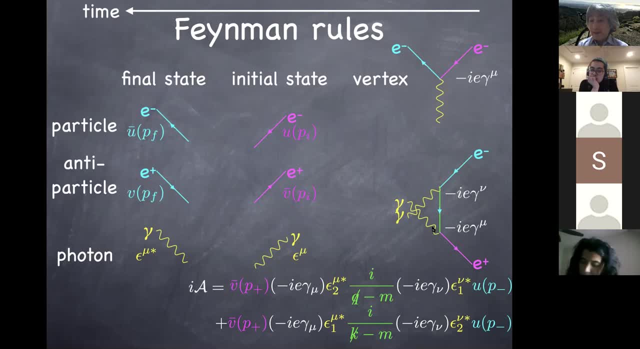 In order to go to a real photon. it turns out, then, that the minimum number is two. Then you can satisfy energy momentum conservation. So you have two-MC: squared: energy in the initial state, but no momentum. Then the final state, photon as one of the photon carries. 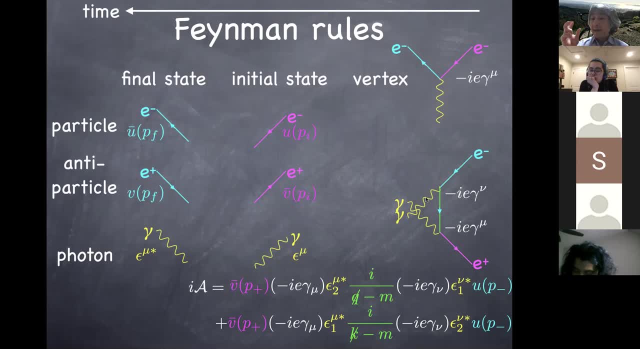 energy of MC squared away and it carries finite momentum and C. Then it satisfies the correct dispersion relation And the other photon has energy MC squared and negative MC for the momentum, so that total momentum during the företier becomes MC squared minus tau Roger's sine wave square. So the problem there is also in the mental state. 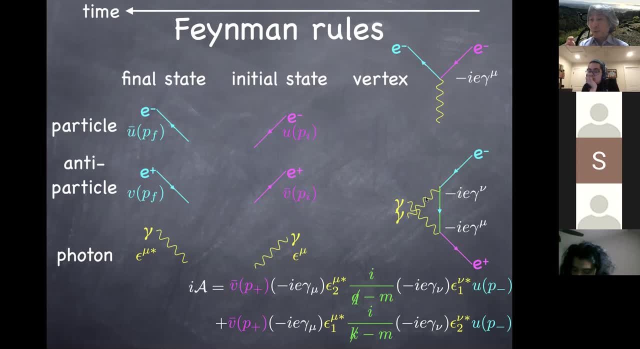 momentum cancels to be consistent with initial state zero. total momentum and energy is also conserved now and dispersion relation is also correct. so in order to satisfy both requirements, that the four momenta, namely energy and momentum, are conserved between initial and final states, but every particles are on shell, namely they satisfy the correct dispersion relation then 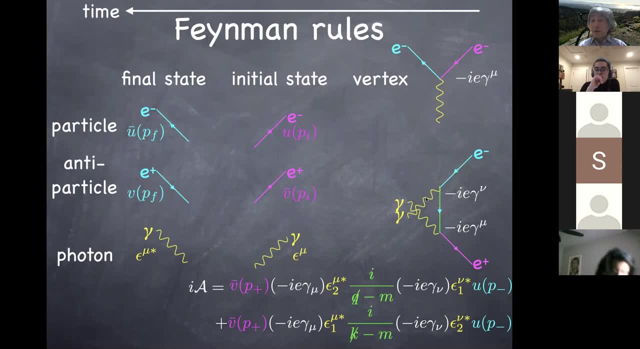 E plus, E minus cannot go to a single photon, but can go to two photons or three photons. does that answer your question? yeah, thank you, okay, good, good, any other questions here? um, I actually have. I'm sorry if I missed this when you were going over it, but when we 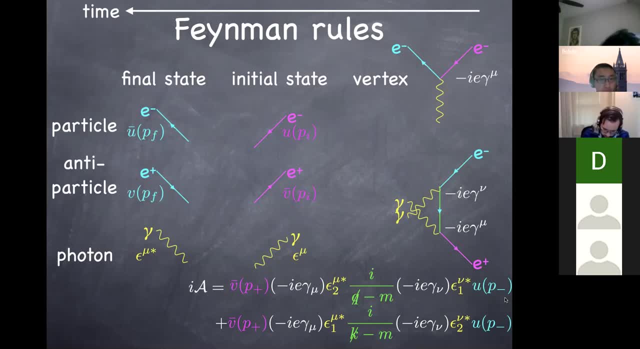 write the Feynman amplitude for this process of E plus E minus the two photons. um, we're adding the terms in the amplitude. do we always add them? or are we adding them there? because the photons are symmetric when you interchange them, so like, yeah, would we subtract? yes, you're completely right, so I 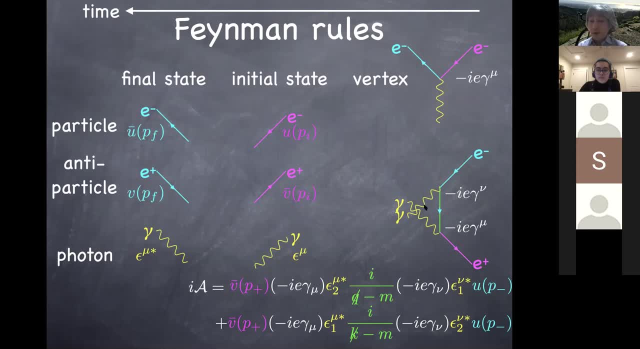 think I briefly mentioned this. so when you interchange two bosons, then there's a positive sign in between. when you interchange two electrons, for example, then you have a negative sign in between. for example, when you talk about the process of the scattering between two electrons, two electrons come in and you exchange a photon. 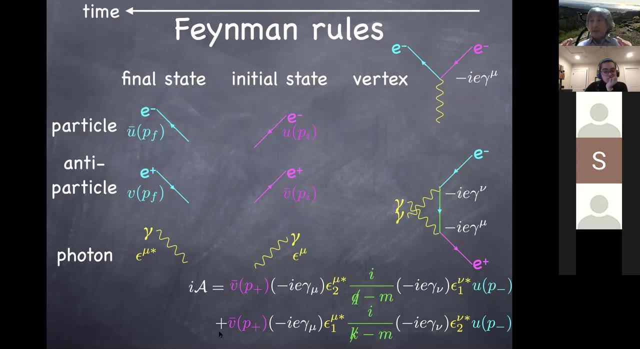 and in between end up with two electrons. so then for a given initial state two electrons you can exchange and go like this, or can also be interchanged to go like that, and you write two diagrams, two amplitudes, but the relative sign between them is a negative sign. 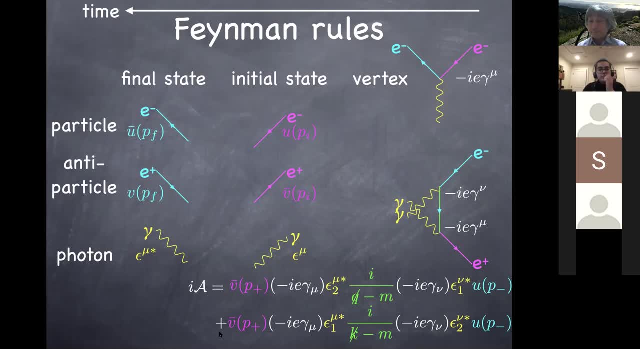 in that case because you're interchanging two electrons. okay, cool, thank you. okay, and again, once you actually go through the time, independent revision theory by sticking in operators. we know two fermion fields and the commute, and that minus sign comes out automatically because of anti-commutation relation. so no, ambiguity is not a sign you're putting by. 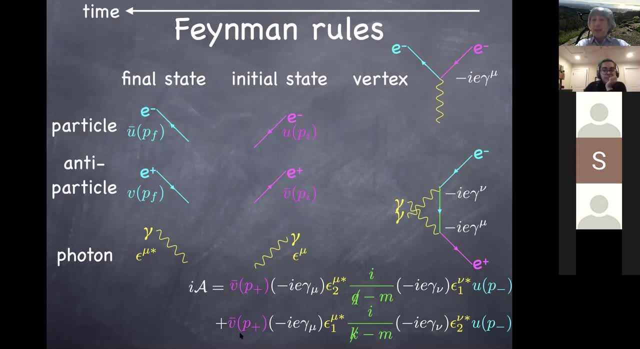 hand it comes out automatically. but when you do the Feynman diagrams you need to be aware that that the minus sign is there. all right, thanks for asking the question. any other questions here? okay, so now I hope you have gotten this idea of how you draw diagrams and how you write down the Feynman amplitude once you have the diagram. 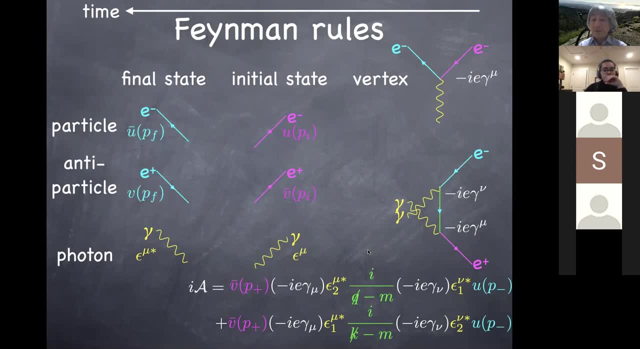 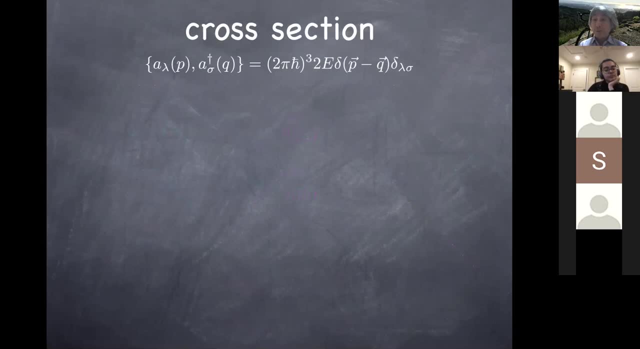 pretty much automatically, now and then the next. the remaining thing you need to know is how to put this amplitude into a square and basically compute the probability, and that's the cross section we already talked about in the case of the weighty scattering. so we have this normalization of the creation annihilation operator given by 2 pi k. 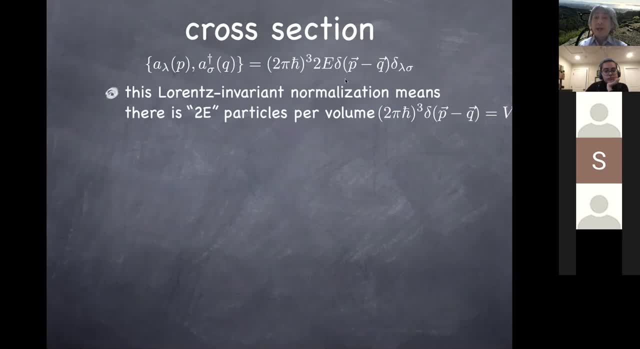 cube 2 e times delta function, and this is the Lorentz invariant normalization. and, and so in this case we need to figure out how to actually take the square of the propagator, how you sum over the final states, and we also need to know the flux factor to divide the probability to obtain 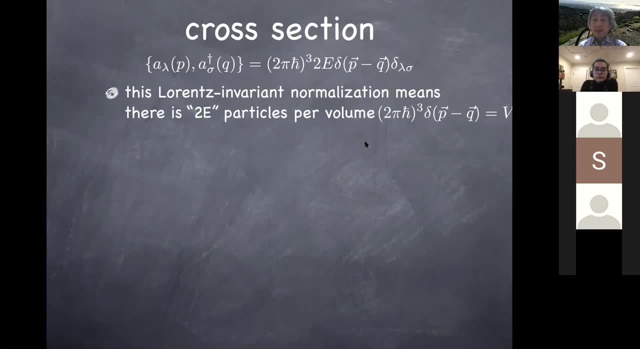 the cross section, like what we did in the case of non-rotoristic uh, the rate scattering. so it's the same idea, but now that normalization is different and it's not the box normalization anymore. so we have to figure this out a little bit more carefully. and the first thing you 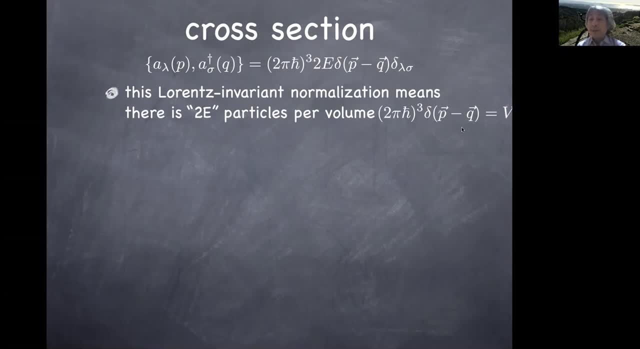 identify is that 2 pi cube delta function in momentum basically has the meaning of space volume. so you may remember this from the Fermi's golden rule. where delta function in energy times, 2 pi h bar could be replaced by the time interval, and that's how we obtain the probability. 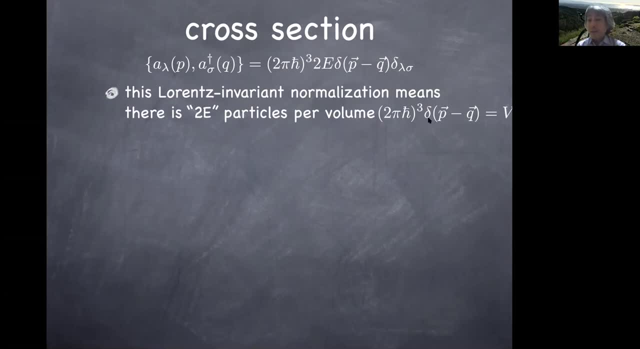 of transition per unit time. so in the same way the delta function in space momentum with 2 pi h bar cube has the meaning of spatial volume. so what that means is that in this normalization of creation, annihilation operator, so this creation operator actually creates two e. 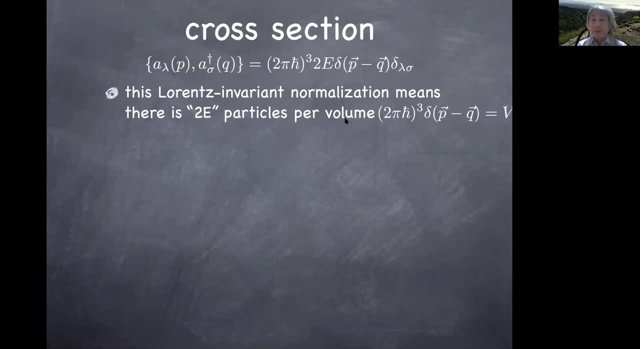 particles in unit volume because of this normalization. so we are not using box normalization so it looks kind of obscure and subtle, but basically that's the meaning of the normalization. so we need to be aware that we have two. e is energy particles per unit volume and using that idea, the sum over final states for each particle also comes with 2e downstairs. 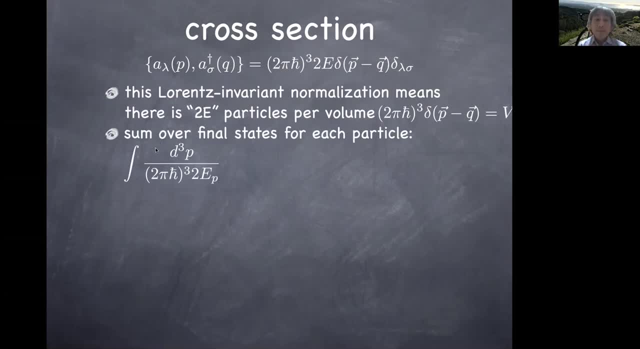 so when we did this box normalization we had v d cube p over 2 pi h bar cube for one particle in the entire space. but here normalization is 2e per v, so you have to divide it by that. so that's why some of the final states would be dpq, d3, dqp over 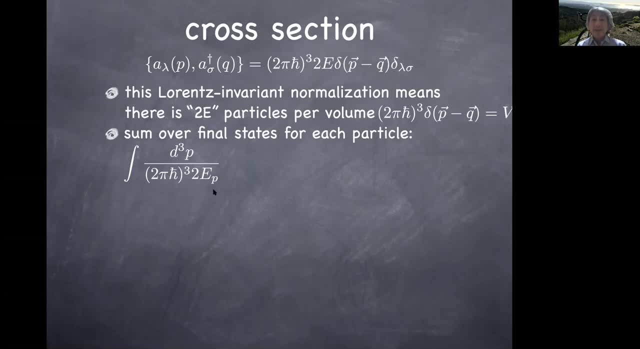 2 pi h bar cube over 2e, and this is the way you sum over the final states for each particle. so this is what is called the Lorentz invariant phase space. and then we also need to figure out the flux of the incoming particle, because you divide the probability by the flux to get the cross section. 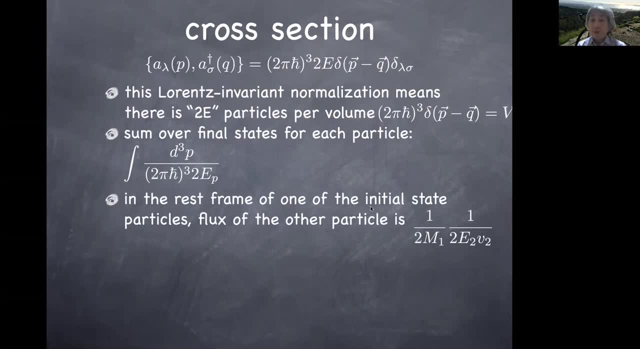 so if you're thinking about the scattering process where one of the initial state particle is at rest, then then the density of the particle per volume is 2e. where e is at rest, then it's mc squared. again, i'm setting c to one, so initial state has two and one particle in it, so the 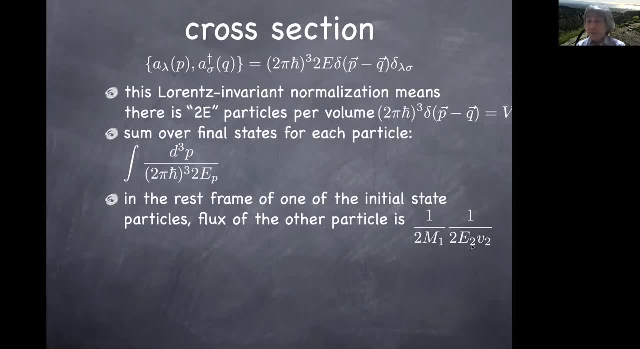 flux factor should be inverse of this. and for the second particle then that's moving and trying to hit the target. so this one is moving. so it's not rest energy but includes the kinetic energy in it. so you divide it by 2e2 for the second particle and to compute the flux you want to understand. 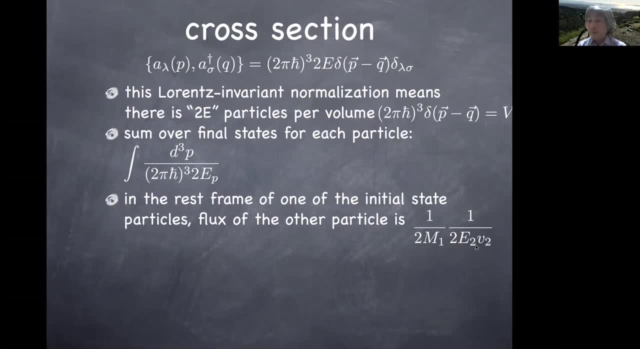 how many particles come per unit time. so you also divide it by the velocity of the second particle. so this is the flux factor. you need to compute the cross section. but this expression is kind of inconvenient because it's specific to a particular Lorentz frame where one of the particles is at rest. so you would like to generalize this expression. 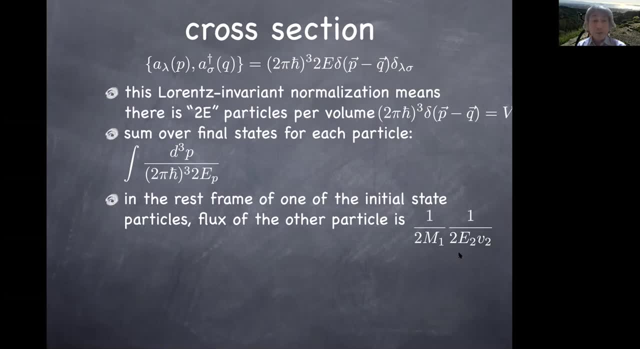 in a fully Lorentz invariant fashion and end result is the expression i remember in the following form: one of a 2s, beta bar i and s is the central mass energy squared, and beta bar i is a little complicated expression which depends on center mass energy squared s and mass of two particles. 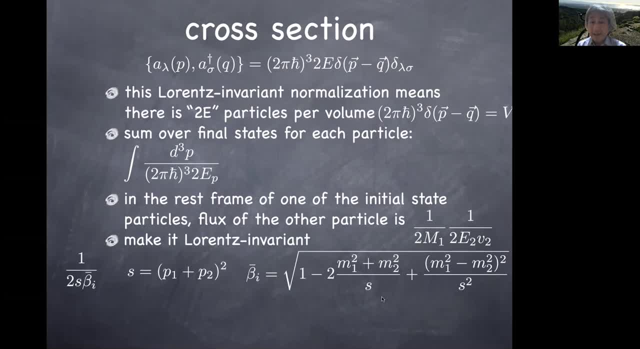 in the initial state. so it's a little complicated. but this has a definite meaning, because if you go to the center of momentum frame instead, then the center momentum frame, it has a total energy squared. it's nothing but this factor s and then in the center of momentum. 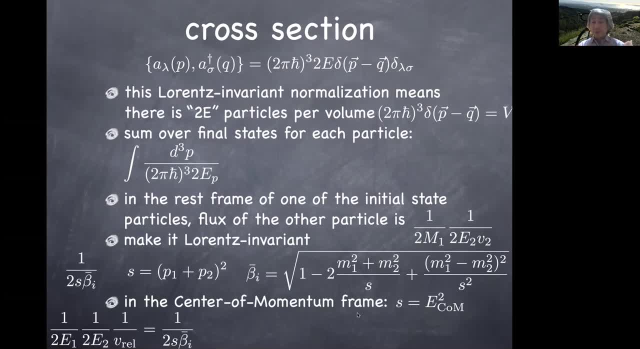 frame, both particles are moving. so this is the case of the collider experiments like the LHC. so each particle now has this number of particles, 2e. so firstachter particle 2e1,, second particle 2e2, and then comes now relative velocity, because both of them are 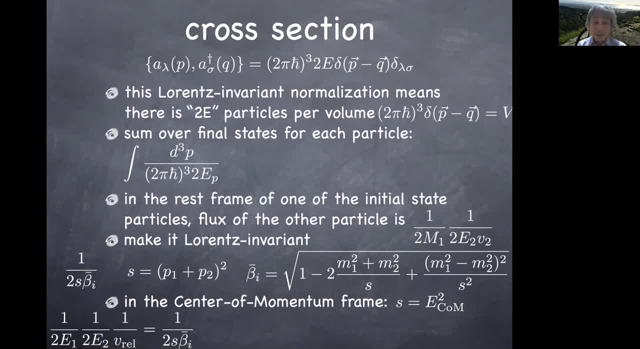 now moving And if you put them together it does turn out to be the same expression at the end of the day, because this is Lorentz invariant expression And in this frame this beta bar has a definite physical meaning. So, roughly speaking, center of mass energy is shared. 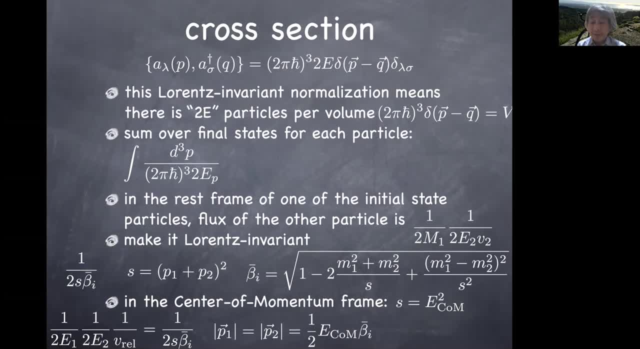 between two particles, So roughly speaking it's a half of it. The times beta bar is the momentum common for both particles, because in the center of momentum frame, by definition, two particles come with the same momenta in opposite direction. So total momentum is zero. 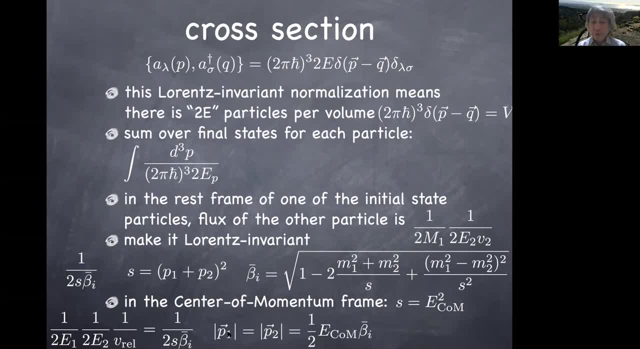 That's the meaning of center, of momentum frame. So both p1 and p2 are given by the same number and that number is where this expression- beta bar is beta bar- appears. So the velocity of relativistic particle is p over e. 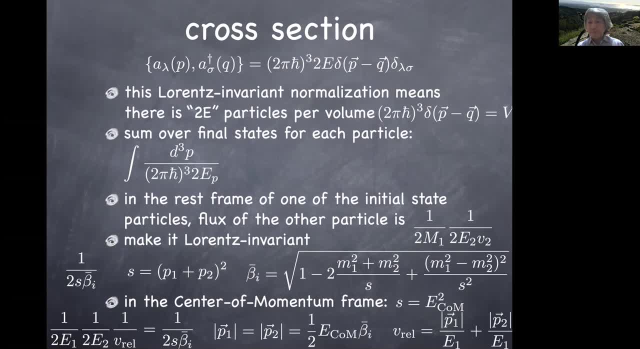 And so relative velocity is p over e for the first particle coming in, But also the second particles, p over e are coming in the opposite direction. So you sum them, That's the relative velocity, And if you put that into this expression, 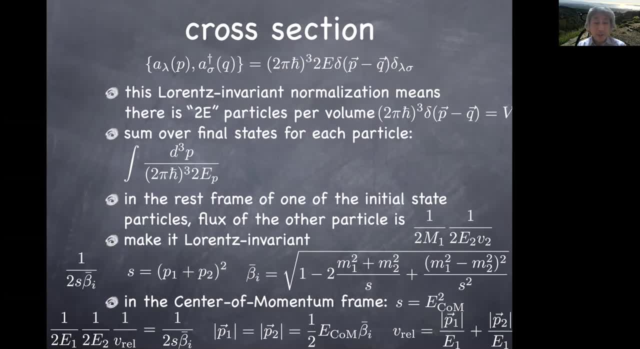 you can see that e1 and e2 combine with e1, e2 here and disappears, And then p2 is the relative velocity. And so, as you can see, P1, E2, P1, e1, also sum them up. 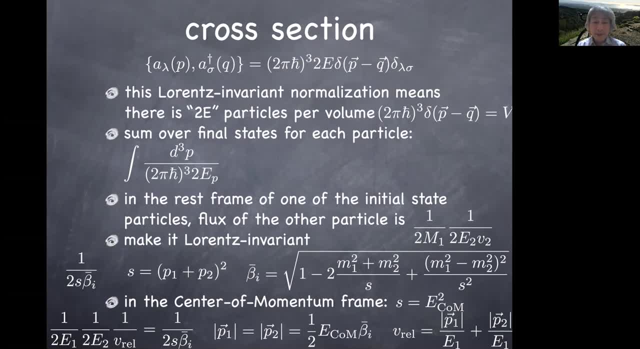 T is now rewritten in terms of beta bar, and that's how you can see this expression coming out. So the idea of using this expression 1 over 2 is beta bar i, which is not familiar to you, probably the first time. maybe you have seen it, but this is the expression that's. 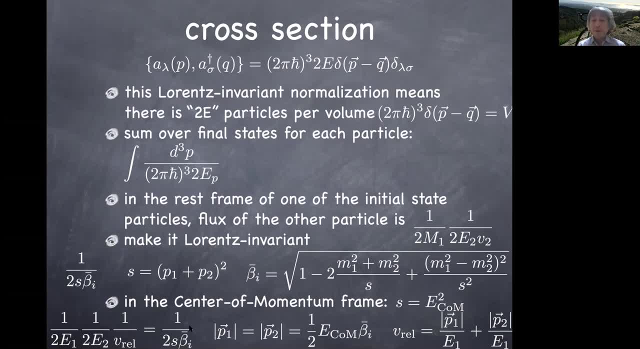 useful to remember, because this is true in whatever reference frame you are in, whether you are in the lab frame where one of the particles is west, or if you are in the center momentum frame, you have the head-on collision in the middle. Either way, this expression 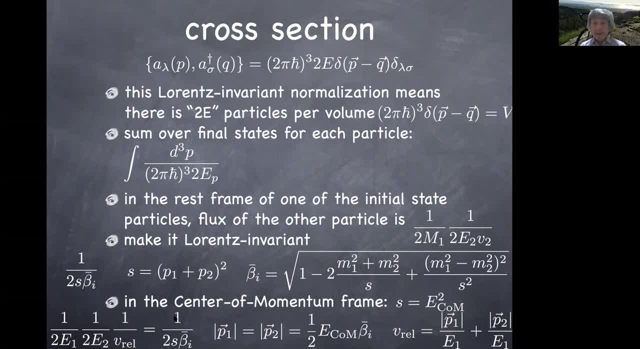 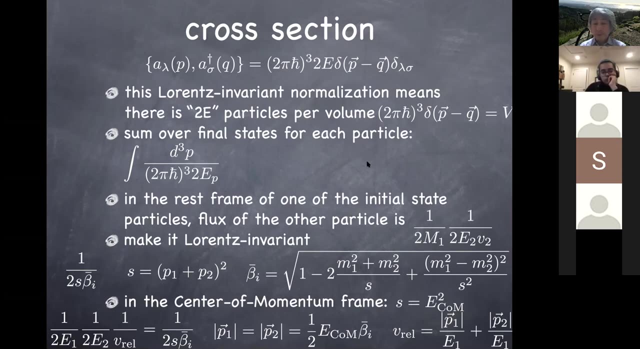 of 1 over 2 is beta bar, i is true, and then you can write down expression for the cross section right away. So this is a little technical stuff, but are there any questions about this? I just had a question about the integral that you defined. 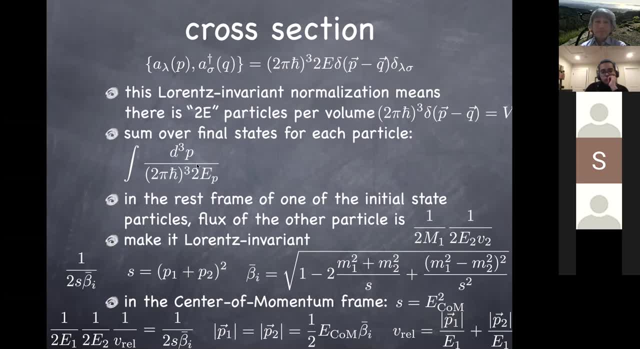 So this momentum integral? Yeah, So is this counting the number of particles over k-space or momentum space? This is counting the number of final states. So if you had done the box normalization a while ago, then in that case the momentum were actually quantized by integer labels. 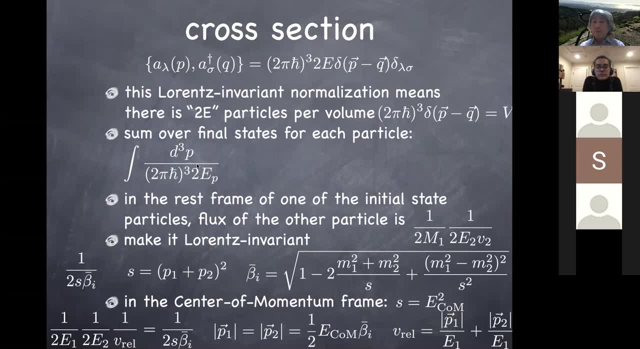 right, Because you have to be in this box. Then you sum over those integers to sum over all possible final states of the particles. So that was the sum in that case. But if you take the infinite volume limit, then we figured out that the sum of the final states is the. 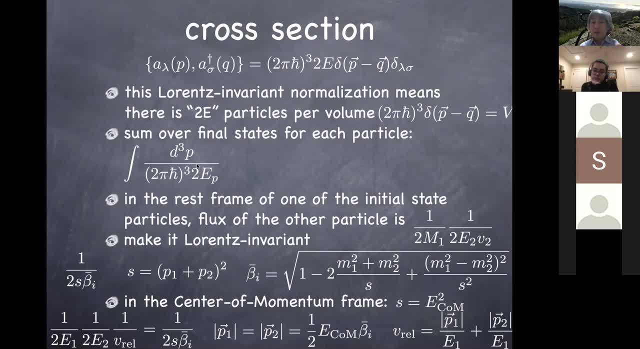 same thing as spatial volume times, momentum integral over 2 pi, h-bar q. So that's what we discussed already a while ago. So this integral is what corresponds to that. So instead of summing over the final states for discrete momentum modes, we have continuum. 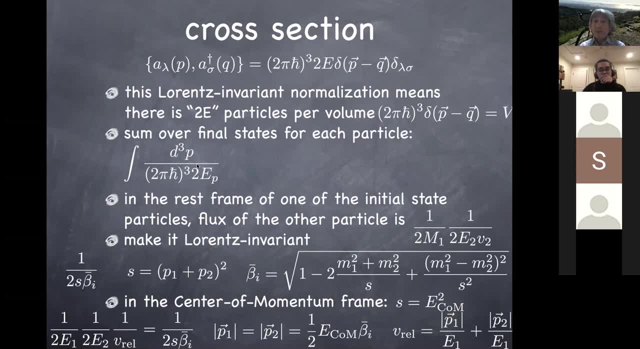 because we are looking at the infinite volume limit And that is an integral, but we have we have this weird normalization with 2e factor in it. so that's why the sum over the final states need to be done with this integral instead of the sum over the integer modes of the momenta. 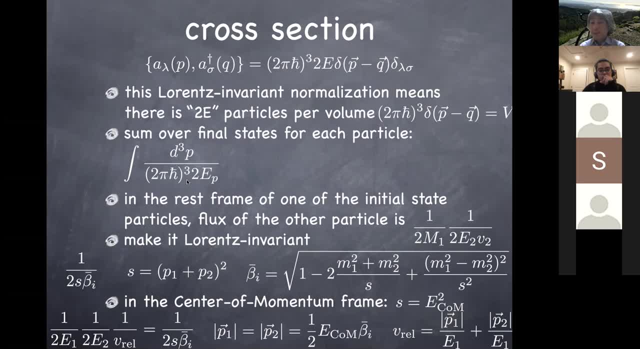 in box normalization. Does that answer your questions here? Yeah, I guess I'm just confused about this interpretation of having 2e particles per this volume defined by a delta function. Right, right. so this 2 pi h bar cubed delta function, roughly speaking, has this meaning of the 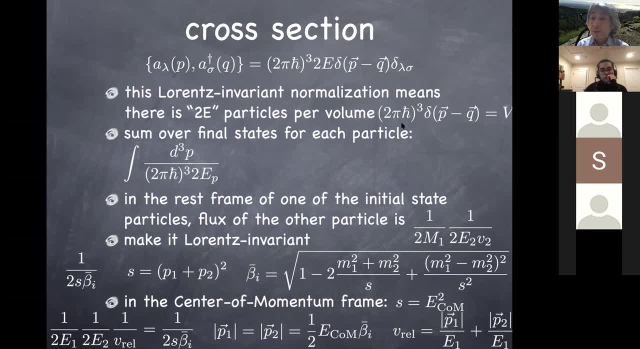 volume, in the same way that in Fermi's golden rule 2 pi h, bar times energy delta function had the meaning of time interval. So this thing here is basically volume. So a, a dagger is not one, but it's 2e times volume. that's what this is saying. That's why a dagger, a is the number. 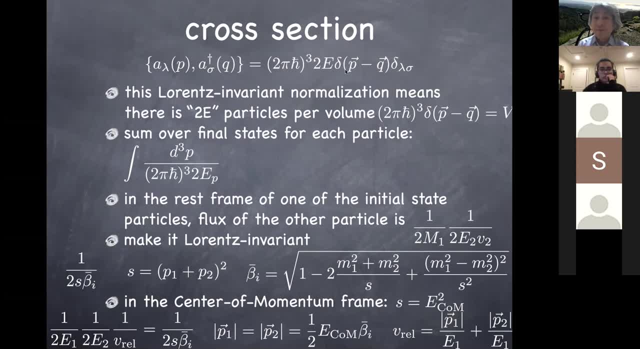 operator Which comes with the normalization of 2e times volume. Hence you have 2e particle per volume using this normalization of creationization operator. Okay, that makes sense. Okay, any other questions? So again, you know, you don't need to remember this argument at all. at the end of the day, All you need 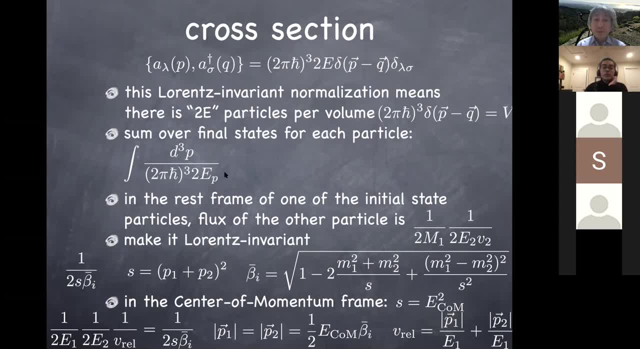 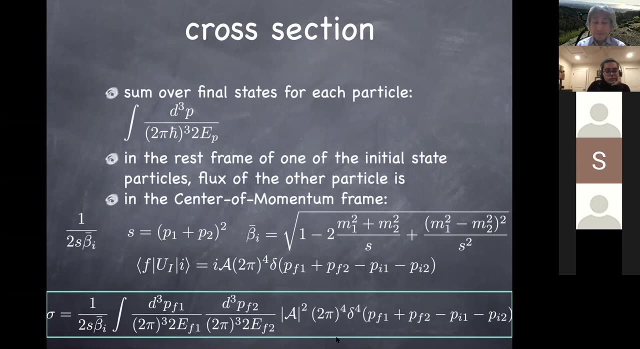 to remember is that sum over the final states is done with this Lorentz invariant phase space, And then the flux factor is given by this one over 2s, beta r, a bit of our i. So if you put all of these things together, here it is, This is the master formula. So you have this Lorentz invariant phase. 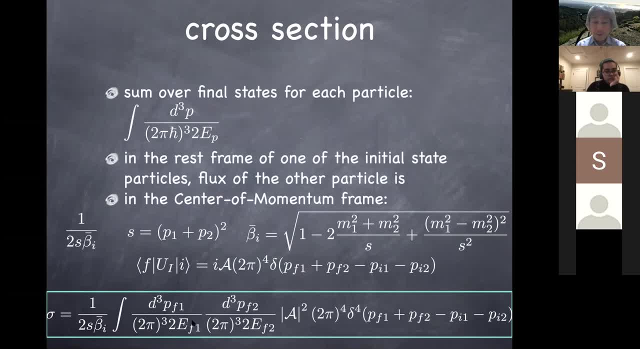 space for whatever final state particle you have. So in this case I'm considering 2 to 2 scattering process. So I have only two particles in the final state. If you have more, you just stick in more integration volumes to it for each particle. So you have to find the final state of the particle. So if you have more, you just stick in more integration volumes to it for each particle. 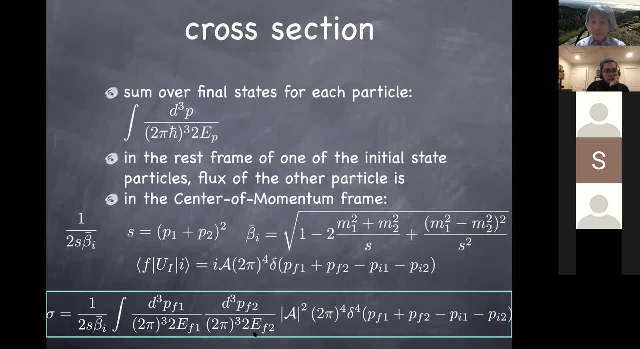 It's always d cubed p over 2, pi cubed 2e for every particle in the final state. And then comes this Feynman amplitude absolute squared for the probability, And then you have this delta function for the overall full momentum conservation. And then comes this flux factor of 1 over 2s, beta bar. 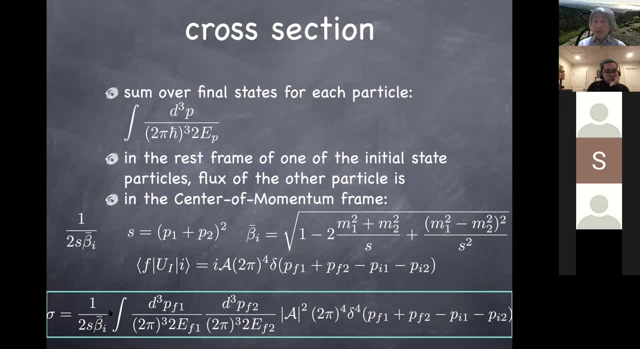 we just talked about, and that's it. So the idea is that once you draw a Feynman diagram, you know immediately how the amplitude looks like, And once you compute the amplitude, you stick it into this absolute square, because it's just a complex number, and that's how you get the probability And then use some of the final. 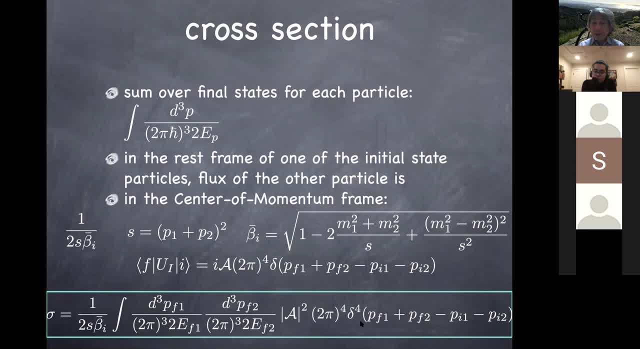 states, using this Lorentz invariant phase space together with this full momentum conservation, And divide it by this flux factor 2s, beta, bar i, and that's it. So this is the way you can compute cross-section for any process you like, once you know the Feynman rules and once you know what the 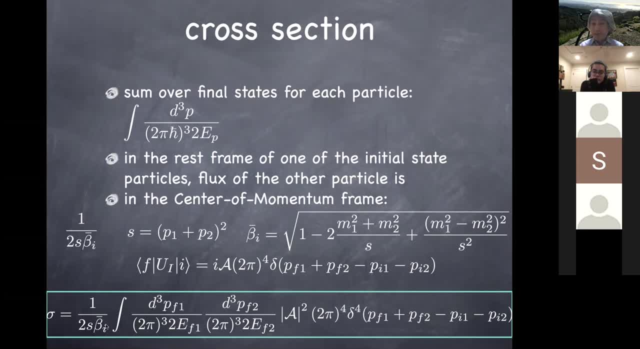 Feynman diagram looks like. So this is the way you can compute cross-section for any process you like, once you know the Feynman rules and once you know what the Feynman diagram looks like. So that's the idea, and so the Feynman diagram is a very practical method. 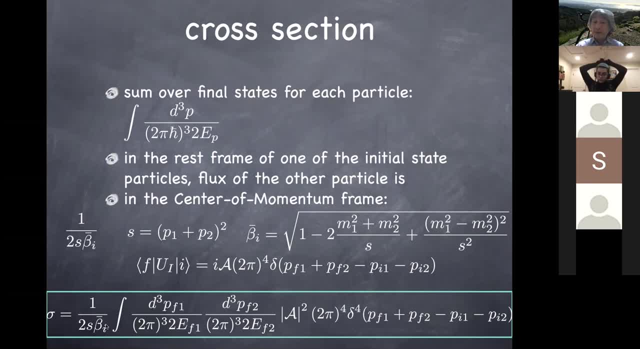 very intuitive, very useful, And then you can go ahead and immediately compute any process for the scattering cross-section using this master formula. Any questions about this? So I hope that gives you a better answer to your questions. again, How about using this sum over the final states in a practical fashion? 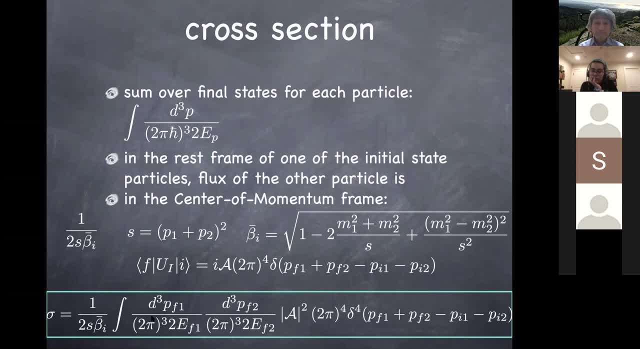 Yeah, yeah, okay, good, Any other questions? questions? So you will see this in action in a couple of slides, So hopefully you get a better idea on what's going on here. No questions? Okay, So, but this master formula still looks a little. 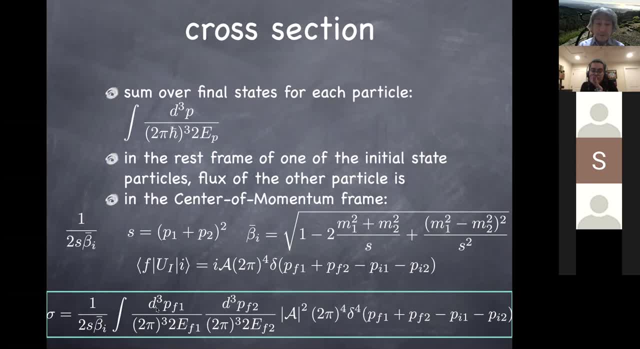 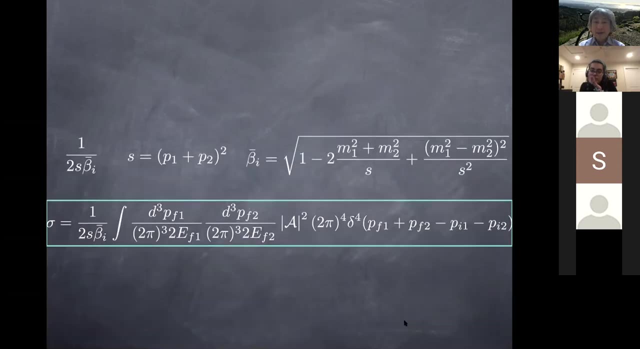 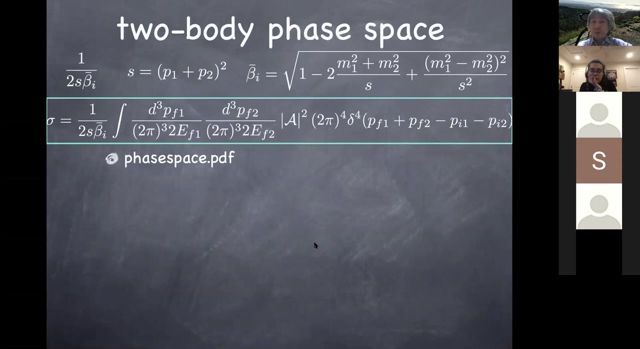 messy because of the delta function, And it turns out that this sixth dimensional integral- that sounds formidable but together with four dimensional delta function, is after all, just two dimensional integrals, right, And you can drastically simplify it. So- and that is actually done in my lecture on space based on PDF, And that's a new lecture. 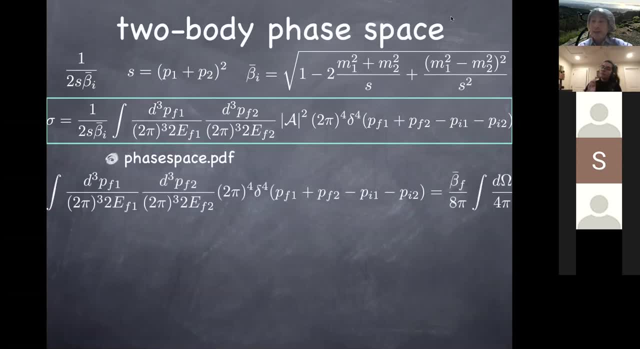 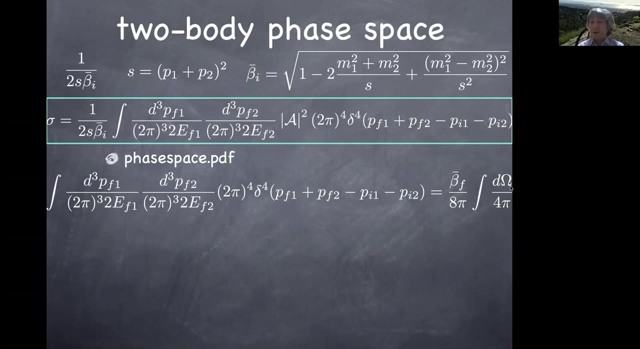 that I put up on the B courses. So please look at that. So there the calculation is shown very explicitly. But at the end of the day, this six dimensional integral with four dimensional delta function just becomes this solid angle integral in the case of the center momentum frame. 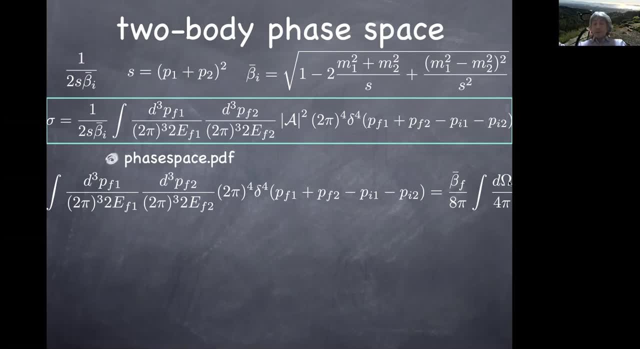 So when in the center momentum frame two particles come in and two products go out. So basically, the only thing you need to know is in which angle in the solid sphere the final state particles go, and that's given by this solid angle integral. So it turns out that 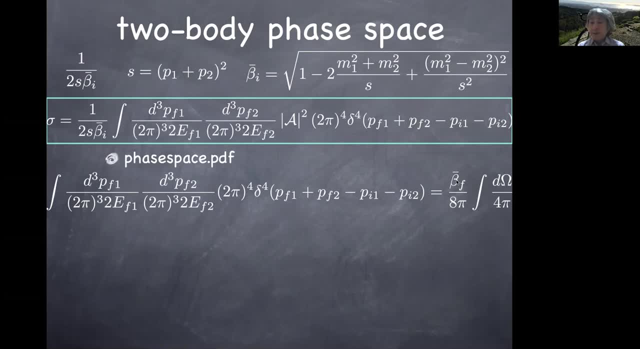 that's it And there's an order of magnitude. So you can see that this is a solid angle integral And there's an order of magnitude. So you can see that this is a solid angle integral And there's an over normalization here which is given by now, beta bar f. So this is the same expression as 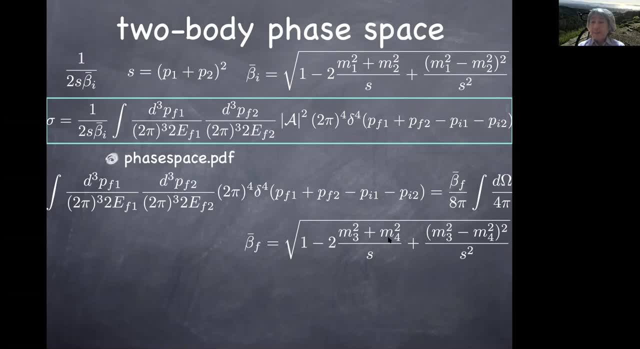 beta bar I, except that I have to put in the masses of the final state particles which are labeled by m3 and m4.. But same analytic expression And this beta bar f over a pi is the overall result of this phase space integral. And then you still need to take care of the solid angle. 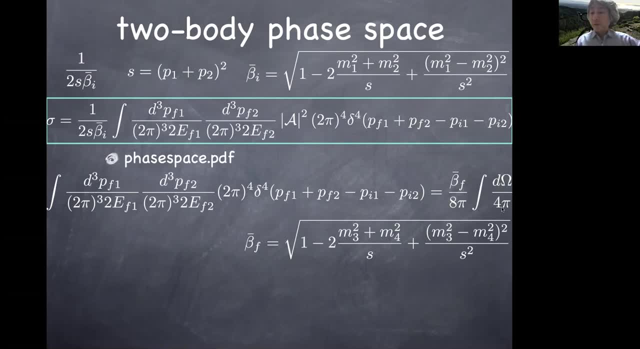 So dependencies of the amplitude squared are normalized of course by four pi. So for simple case of elastic scattering, then initial and final state particles are the same. So m1 is same as m3, m2 is same as m4, because beta bar i and beta bar f are the same analytical. 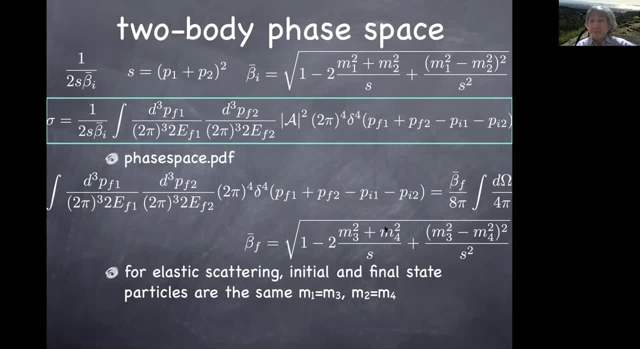 expressions. If the masses are the same, they are really the same. So beta bar f coming from the phase space integral and beta bar i in the flux factor cancel. So this case is really simple. Cross-section is 1 over 16 pi s. 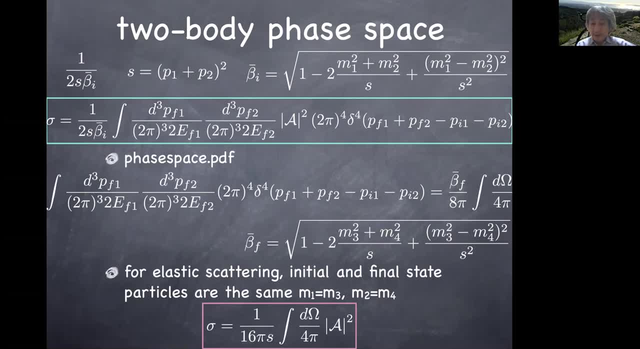 Again, s is the center of momentum, energy squared and sorted angle integral of the Feynman: amplitude squared, and that's it. So, using this expression, we will look at the electron-proton scattering again and also e plus, e minus, annihilation into mu plus, mu minus once again, and actually get the 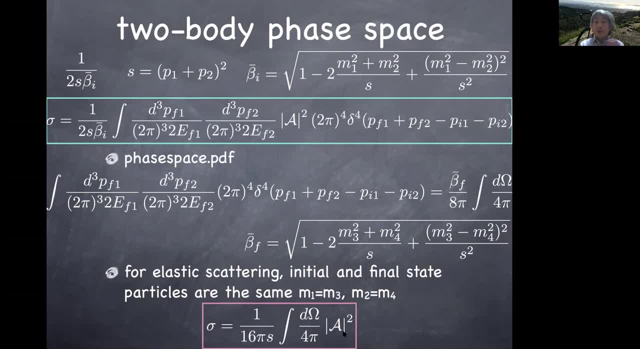 cross-section, Then that's a physical observable you can compare with the data. So that's the idea of this cross-section: how to actually work out the cross-section using Feynman, amplitude squared and the phase space, integral and for elastic scattering. 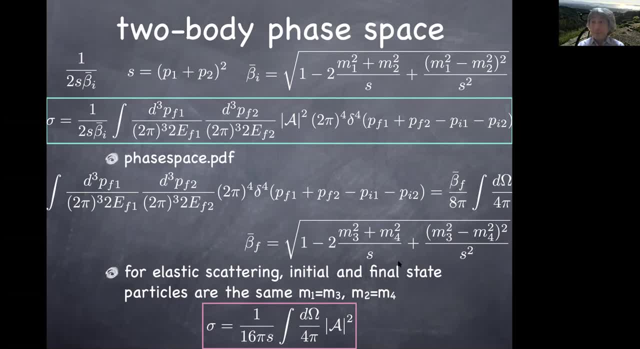 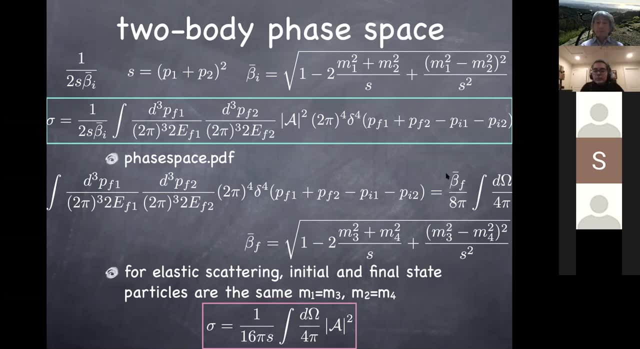 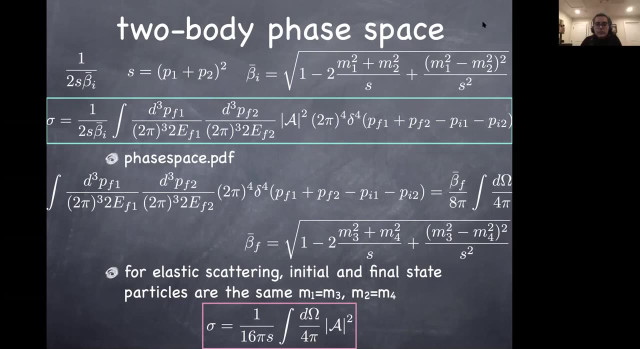 of the 2 to 2 process. it's particularly simple. Okay, any questions about that? Okay, Oh, I just I think that maybe the slides got cut off, Like I think the formula for the simplified integral got cut off. 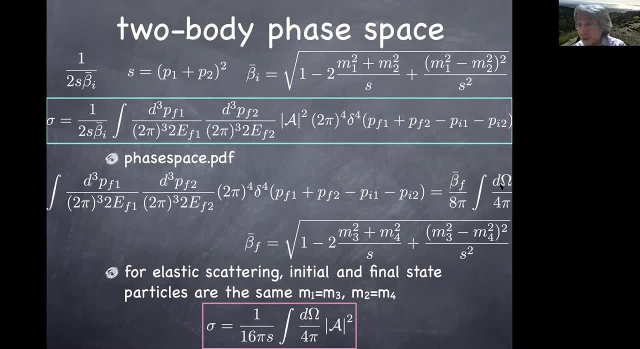 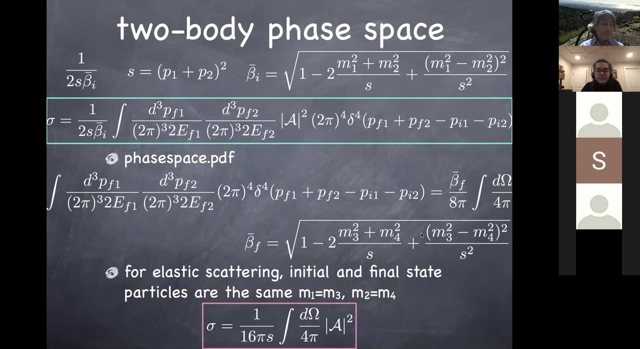 This one with omega. Yeah, This just ends with d, omega over 4 pi. There's nothing further, right? Okay, okay, Yeah, So this is really the end of it. I tried to squeeze it in Any other questions. Yeah, again, once you see this in action, you get a better idea. 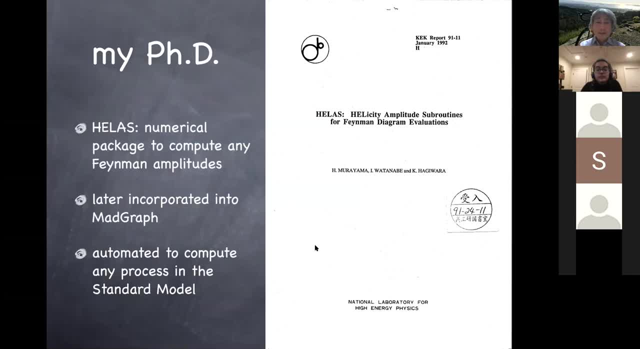 So let's actually get to an example. So, by the way, this is my PhD thesis. So when you actually do this Feynman diagram calculations, when you go to a little bit more complicated process of not the 2 to 2, or 2 to 3,, 2 to 4, and so on, really quickly 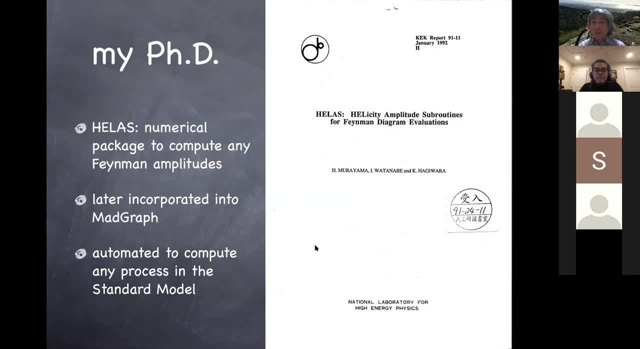 you find many, many diagrams. you can work them out by hand. you have to learn some numerical techniques. So we- I actually wrote a software package to compute the Feynman amplitudes for any quantum field theory by gluing these internal lines and vertices and so on as a package. 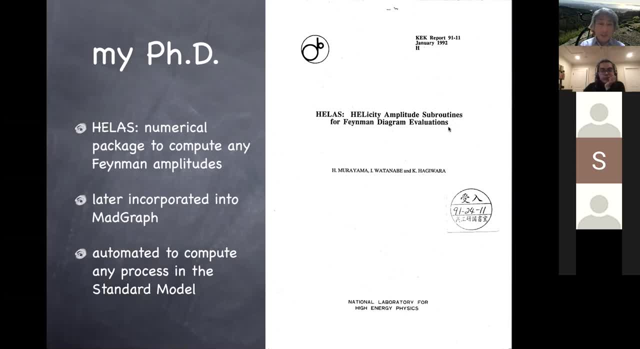 And I call that helus, which corresponds to helicity amplitude subroutines. And later this was automated and it became the engine of a bigger package which compute any process in a standard model automatically. Okay, And that package called MADGRAPH. 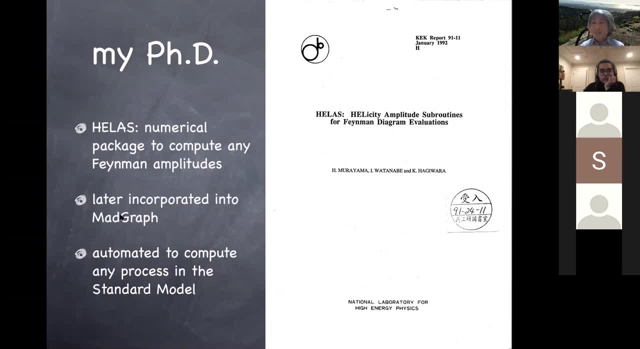 So MAD in this case is not mad. This is actually written by people at Madison University of Wisconsin, So that's why this is MADGRAPH, But anyway. so if you actually look it up you can find the software package you can install your computer. then you can compute any process you like in the standard model. 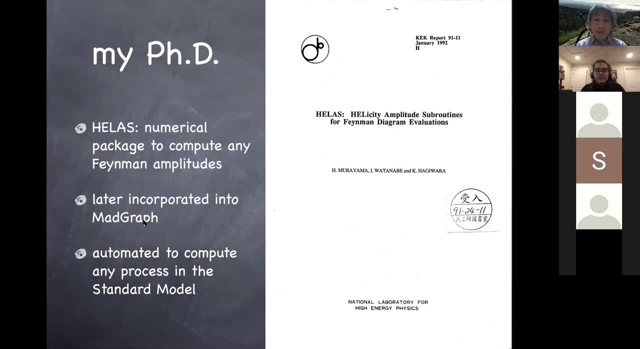 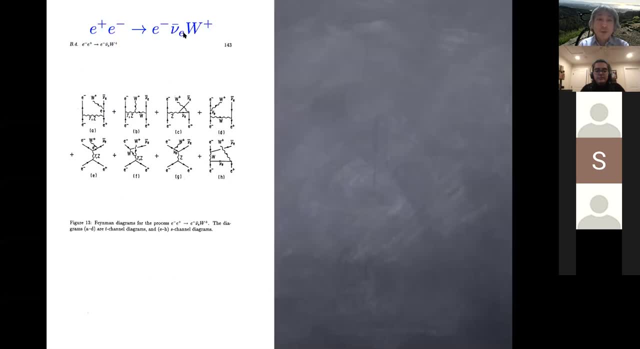 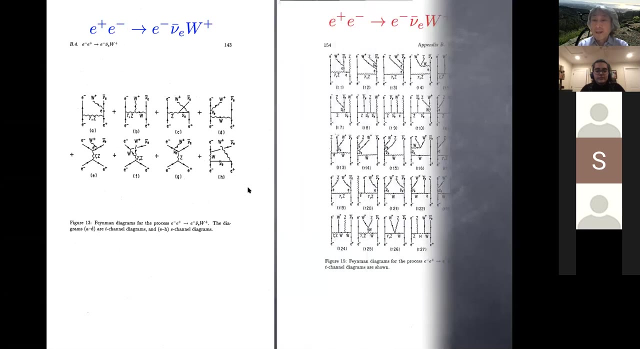 on your laptop using this package. So that was my PhD thesis, actually, And the reason you have to rely on numerical methods us is the minute you talk about, for example, two to three body process. you already have eight diagrams. if you go to two to four, you may have this many diagrams that you can't possibly do. 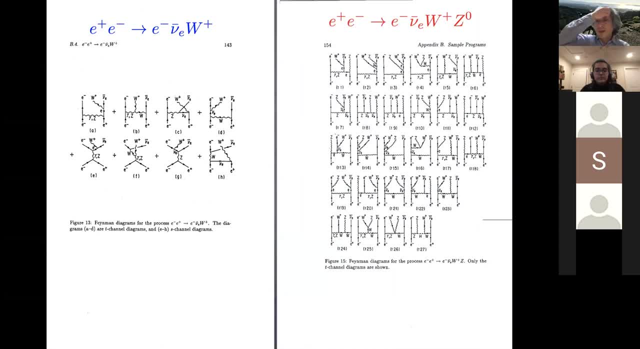 this by hand anymore, so that's why you have to rely on some numerical techniques, and this is the way you actually do the computation for more complicated processes. so today in class we only look at very simple cases where we can do things by hand, so that you get an idea how things work. 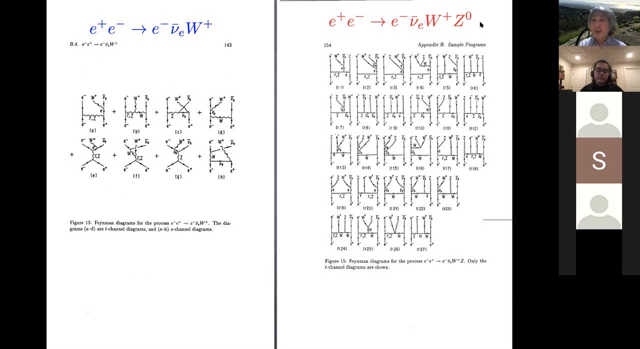 but in most practical situations you do have to rely on some other numerical packages to actually compute the Feynman diagrams, so you just need to be aware of it. so we're only looking at the simplest examples possible, but in practice you may have to do something different, because most cases you can't do this by hand. all right, 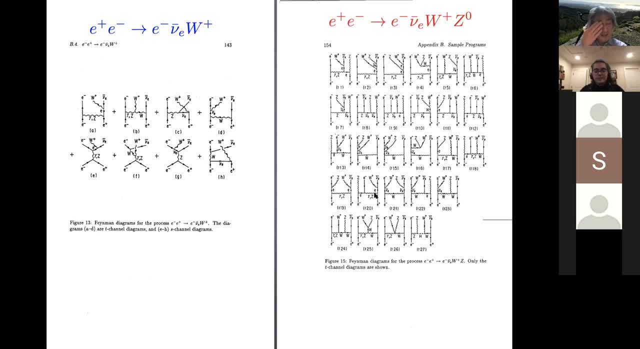 and, by the way, when I actually wrote my PhD thesis using this software package, I nearly failed my thesis defense back in these those days. people didn't appreciate how complicated these calculations can be. so the theorists on the committee said: well, this is not theory, it's just. 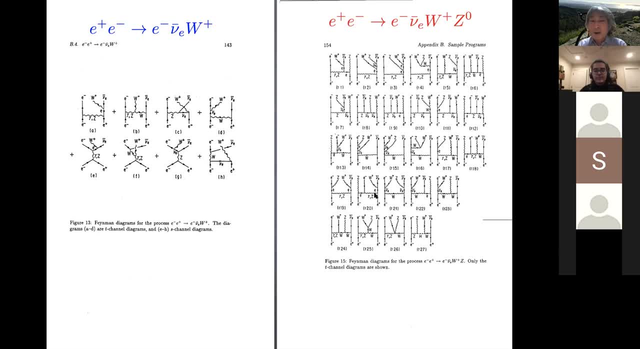 a computer program. experimentalists on the committee said: well, this is data, but not experimental data. so you know there was a huge argument apparently on the committee if this was both yphd. I nearly failed. fortunately there was one professor in the committee who defended me. so here I am with PhD and I am professor of physics. so you know I almost missed it. 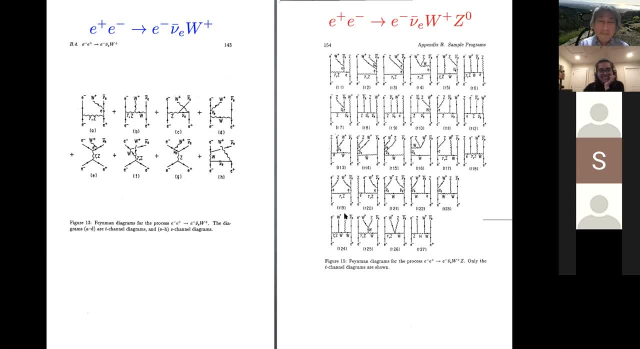 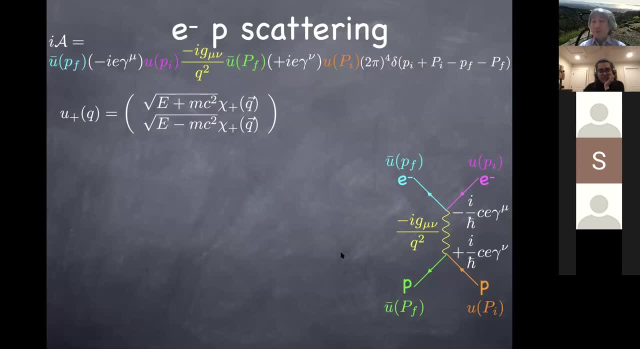 that's something, yeah, it might happen to you, so just be aware of that. okay, so now that we are now equipped with all the tools we need to compute the actual cross-section, so let's see that in action for the electron proton scattering. what we have here is: I can compute it by, and I can compute it by I is equal to the. 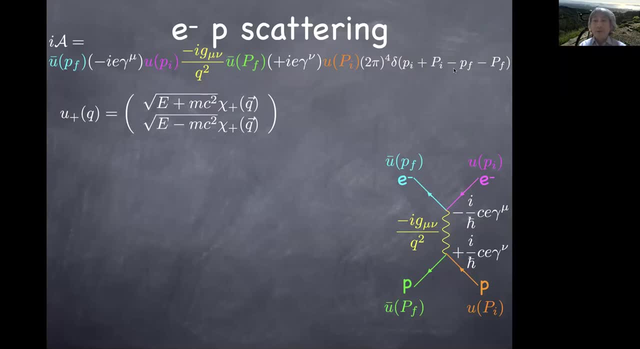 Δm psi. we already have it. we already figured out what the Feynman diagram is, and for this diagram, we could always figure out what the Feynman amplitude is. so the only thing then you need to put in is this: positive energy solution U right. 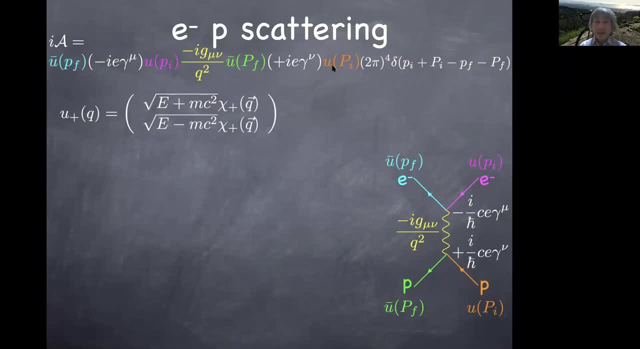 and that's all you need to do. so let's say: we do this in the limit of non-relativistic situation and then, in a non-relativistic situation, the positive energy solution simplifies the limit. energy is basically mc squared. You can ignore the kinetic energy which is suppressed by 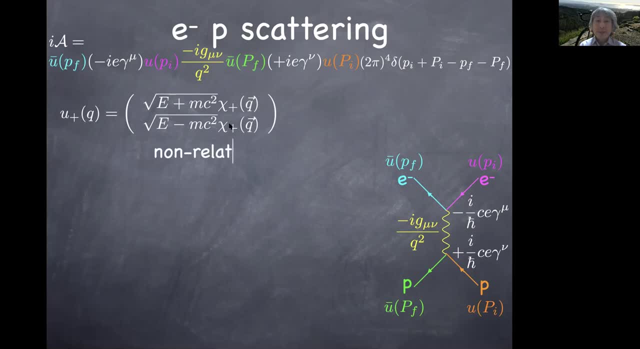 1 over m. So second piece here is gone. You only have the first two components with the normalization given by square root 2m, which is mc squared plus mc squared. I set c to 1 as usual. So that's particularly simple And because you have only upper two components, when you look, 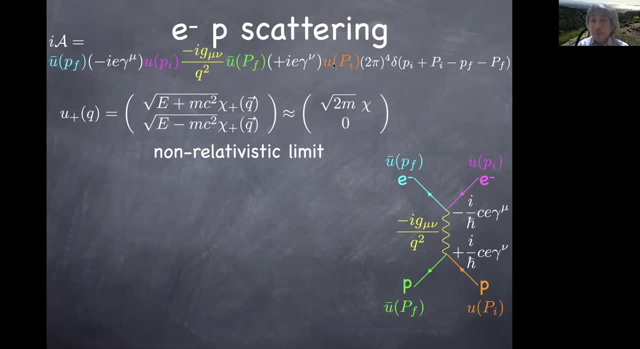 at this combination of u, bar, gamma, nu, u, gamma matrix for spatial components is off diagonal block. But for off diagonal blocks upper two components would go to lower two components, which is zero. so they disappear. So the only thing that survives is actually the time component. 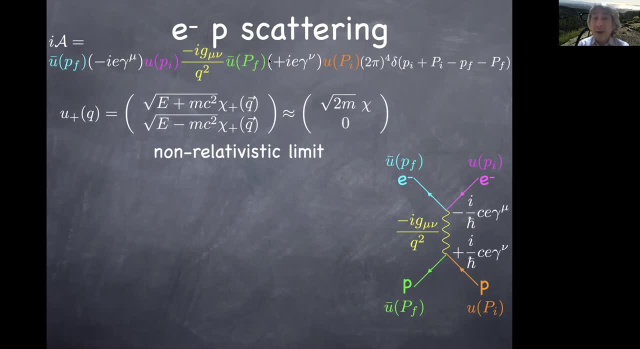 And u bar is u dagger gamma naught times, gamma naught, Gamma naught, gamma naught is 1.. So all you need to do is compute u dagger u And that's this combination over here for proton line or electron line. 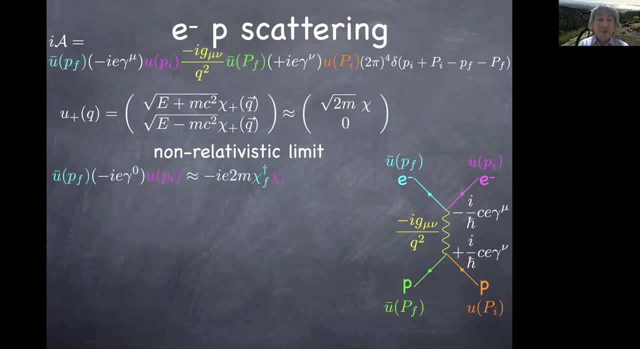 So this is particularly simple in this limit because for the electron line only the time component survives, which is minus, ie from this Feynman vertex times 2m. That's this normalization squared And final state 2m. So this is the initial state 2 component spinner. You can choose the helicity eigenstates. 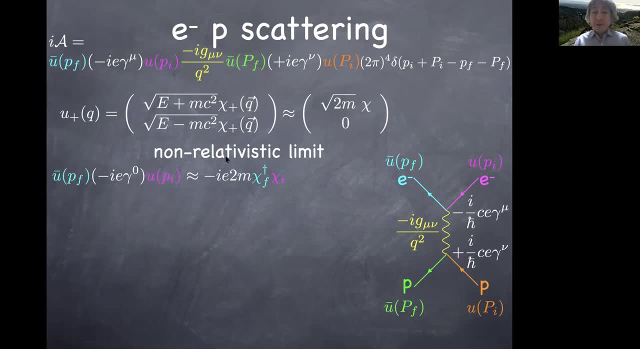 as we have been doing. But you don't need to do this because in non-normativistic limit the spin is approximately conserved, right? So you have done the homework problem. where you have the finite momentum, then spin is not conserved. You have to make sure that you look at the total. 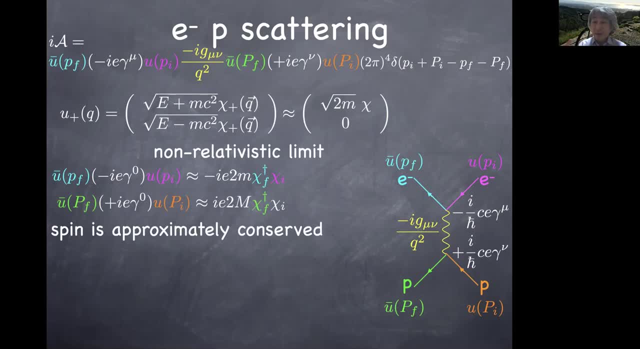 angular momentum together with the orbital angular momentum. But when p vanishes, Hamiltonian for the Dirac operator is mc beta And beta commutes with sigma, So spin is conserved. So I can take this initial state to be spin up. Then the final state is also spin up because of the inner product. 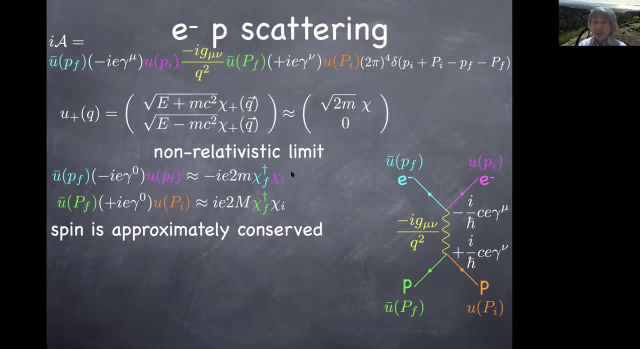 So you can forget about spin degrees of freedom as well that way. So everything becomes very simple. Same thing is true on the proton side. So u bar gamma naught, u gives you ie with the opposite sign, because proton has a spin Positive charge to capital. M for the proton mass, which is 2,000 times bigger. So I'm using capital. 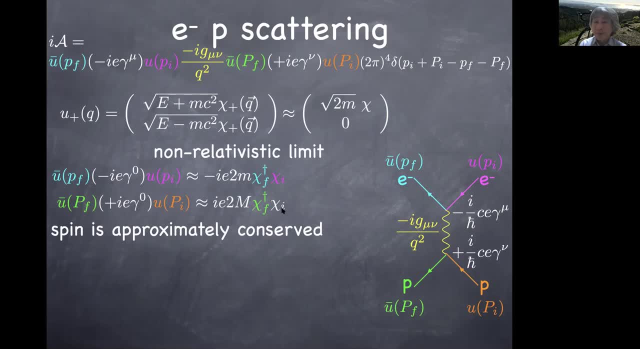 symbol for that. Again, spin is conserved. So I can set the spin wave function to be 1, just by assuming that spin up came in and spin up going out, Then chi, dagger, chi is 1.. So I can forget about the spin degrees of freedom. Then I know everything in this Feynman. amplitude, So amplitude. 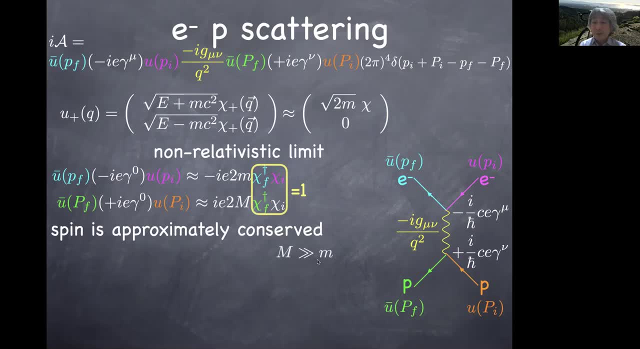 especially in the limit where proton mass is regarded to be much larger than electron mass, which is true, 2,000 times bigger. Then I can forget about the recoil on the proton side. Then kinematics also becomes simple. Initial state electron comes with velocity v. 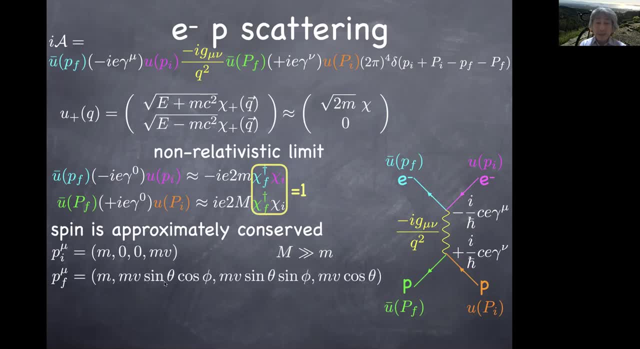 Final state electron also goes out with velocity v, but in some off direction, after the scattering which I described by the solid angles, by spherical coordinates. Then momentum transfer of this virtual photon. Again, I have to conserve full momentum at this vertex. So the q mu is the same as pi minus pf. I use pf minus pi rather here, And so then it can. 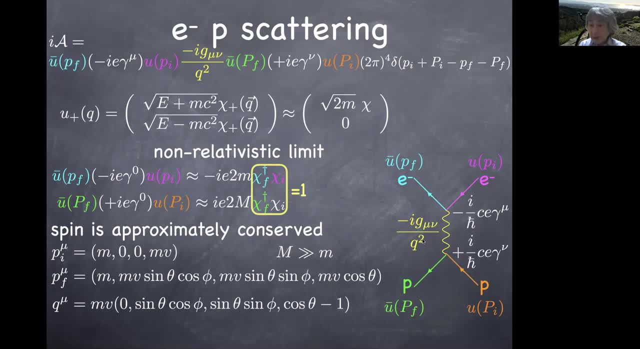 be written out explicitly, But the only thing I need is this: q squared, namely time component squared minus spatial component squared, So I can immediately compute what q squared is. That turns out to be this, And for some historical reason people often write this using sine squared theta. 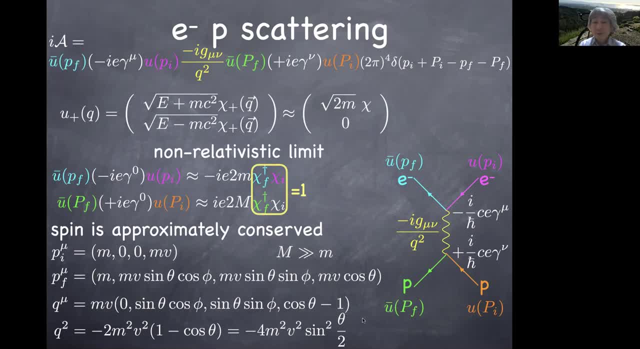 over 2 instead of 1, minus cosine theta, So that's the q squared. So now I know everything. So this piece here for the proton line, that's this Ie to m. This piece here along the electron line, this is minus Ie to little m. And then I have minus ig 0, 0, because both of them are time component. 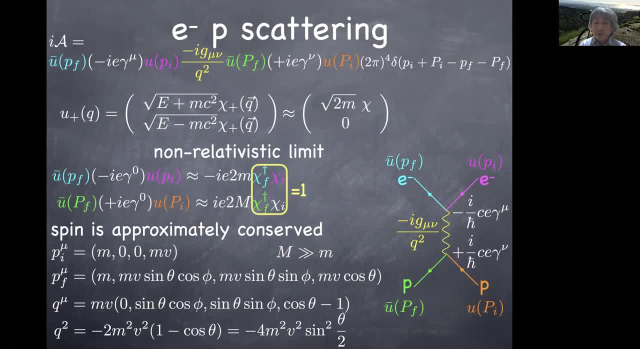 g 0, 0 is 1 over q squared, which is given by negative 4 m squared, v squared, sine squared theta over 2.. So I know everything about the Feynman amplitude. Then I put that into the master formula for this very simple 2 to 2 case which we worked out on previous slide And out comes: 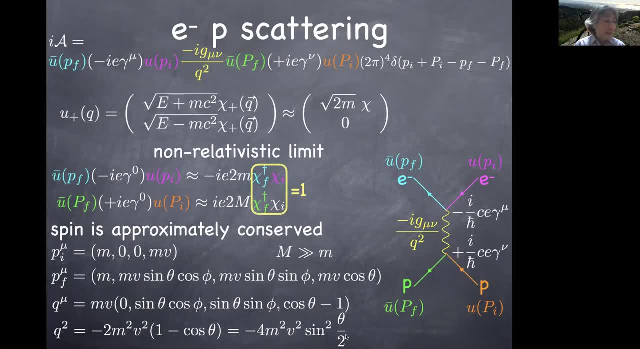 the cross section. So that's what I'm going to do on the next slide. Any questions about this? How exactly was q derived? Again, Yeah, So q mu is. you have to consider full momentum at this vertex. So the q mu- if I view q mu coming this way- is that pi plus q would equal pf. 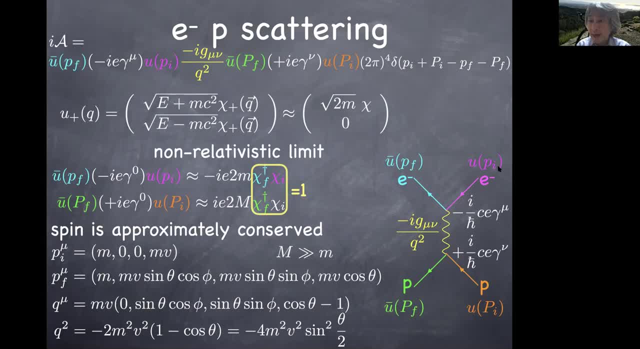 So q then is pf minus pi. So here's the pf, Here's pi. So I subtract pi from pf. That's why time component vanishes. So q mu doesn't carry any energy. And for the spatial components, this minus 0 is this piece. here I factor the mv up front. For the y component, this minus 0,. 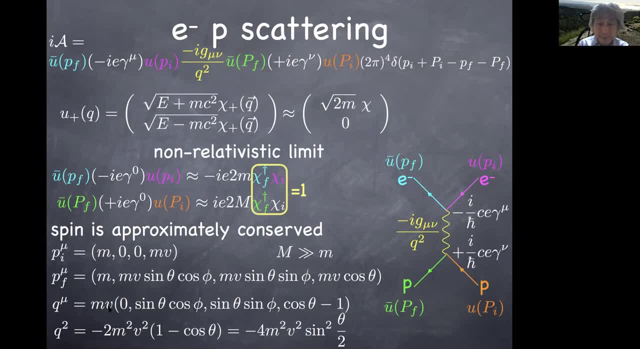 again is this piece. here I factor the mv For the z component. I have mv, cosine theta for the final state, But mv in initial state. that's why I end up with cosine theta minus 1 times mv up front. Does that answer your questions, Sahil? 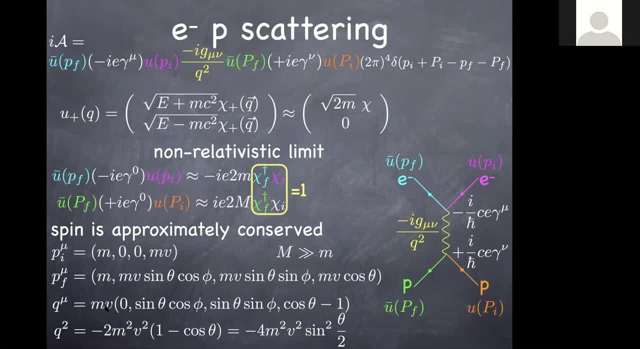 Yeah, yeah, You just applied it to the electron positron vertex. That's right. And if you do this on the proton side, you again get the same answer: because you conserve full momentum at this vertex, You conserve full momentum at that vertex. 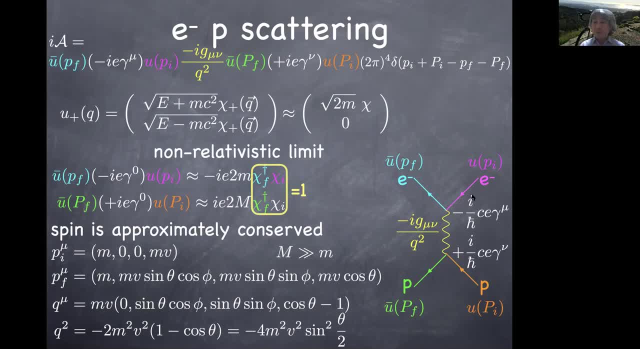 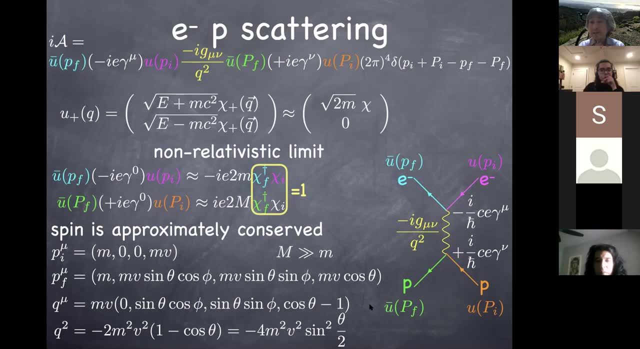 And everything turns out to be consistent, with full momentum conservation between initial and final states. OK, Any further questions on this? So now you're seeing everything in a OK. so now we're going to compute the amplitude of the amplitude. And we can see that, if you compute the amplitude of this amplitude, 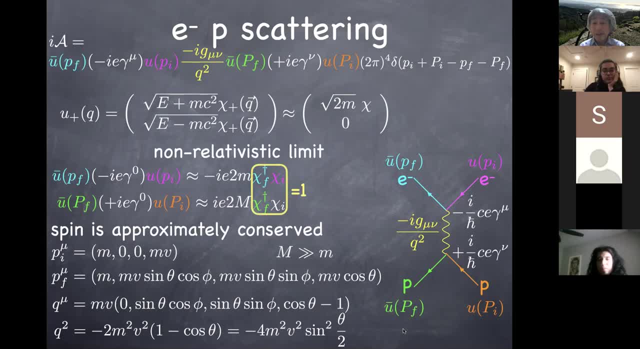 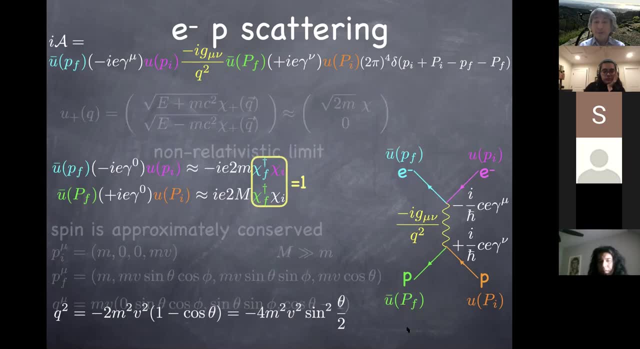 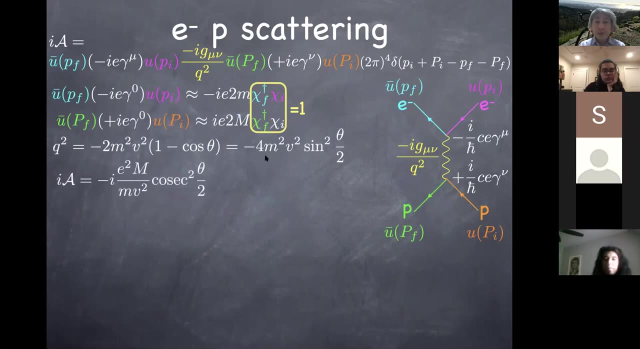 you can get the cross-section. So it's a 4-second cross-section And you see that all the ideas we talked about for QFT this semester is now coming into something really practical you can use to compute these scattering processes. OK, So now that I have this Feynman amplitude now already worked out, I just put that into the master. 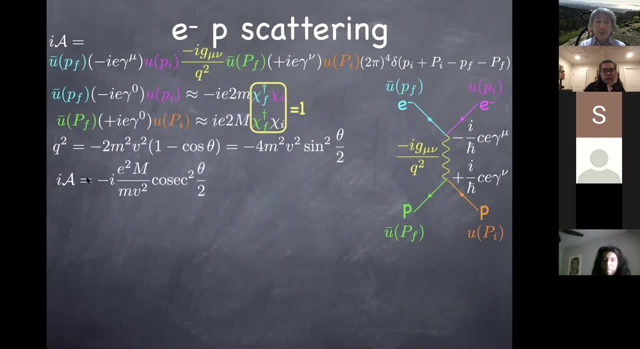 formula and get the cross-section squared And I square this Feynman amplitude to put that into this simple master formula for the cross-section. So you have this solid angle integral, So differential cross-section. d, sigma, d, omega then comes out to be this: And S is a center of mass energy, squared because both of 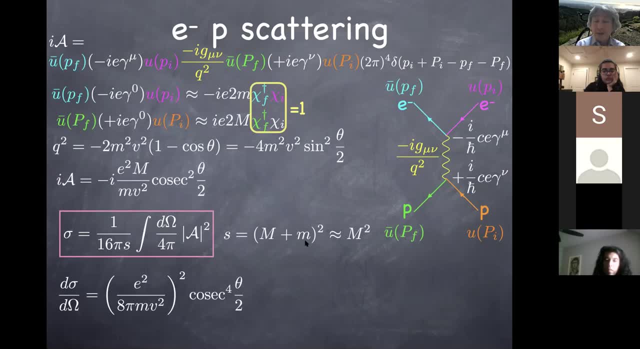 them are non-retrovistic. Center of mass momentum, sorry, center of mass energy- is just some of the two energies MC squared and MC squared for electron and proton. You square that We are in the limit where little m is much smaller than capital M. So this is approximately capital M. 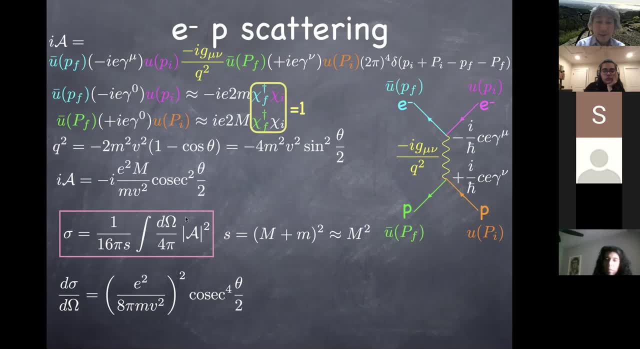 squared. That's this flux factor over here. But Feynman amplitude has capital M upstairs, So that gets squared. So capital M dependence cancels out. The only mass dependence then is actually mass of the electron. So it's basically that, if you actually retain, 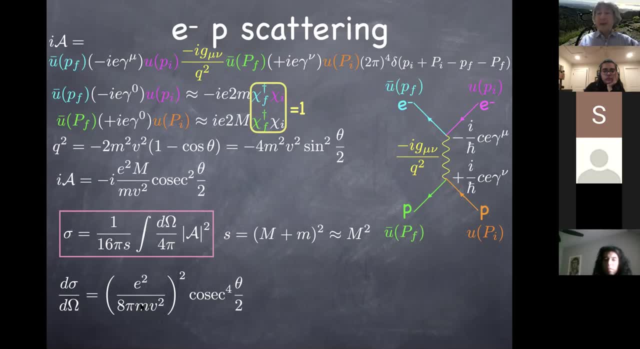 both of these, you can actually get the mass of the electron. So it's basically that if you actually retain both of these, you can actually get the mass of the electron. So it's basically masses correctly, this m is the reduced mass of this little m plus capital M system. 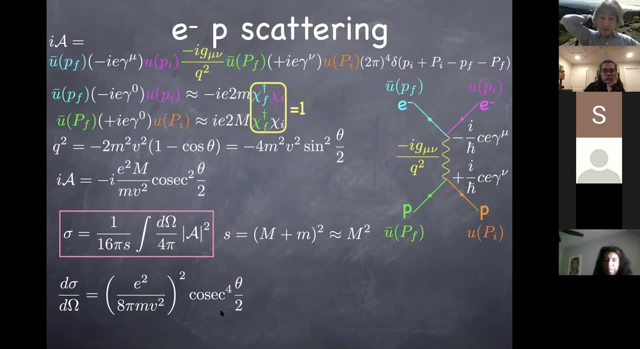 And then you find this dependence of cosine. second, fourth, the theta over two, And if you recover c and h bar, it turns out for this formula that c and h bar is not needed to get the correct mass dimension. Only thing you need to put in is this: 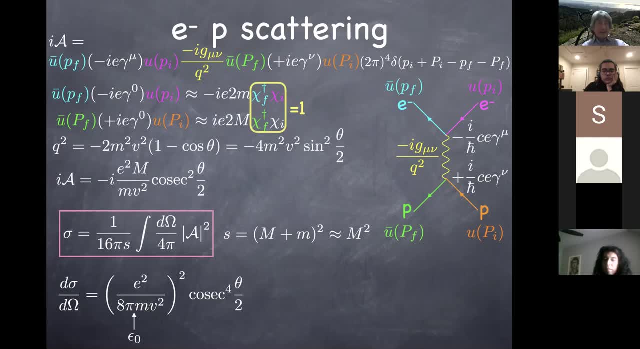 not magnetic permeability, that wasn't even permissivity of the vacuum, And that's the only thing you need to provide to get all the units back. And once you have this expression, you might say: oh, this looks familiar because this is exactly the same expression. 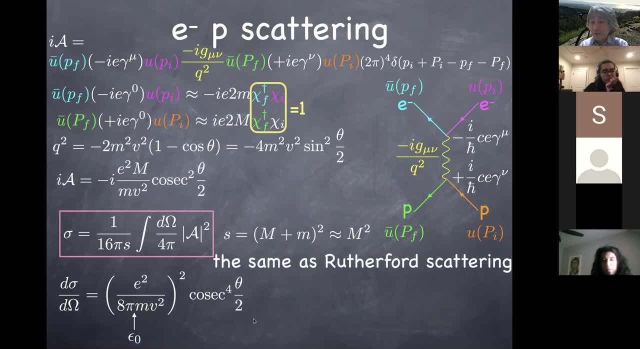 for the weatherport scattering. you have worked out in classical mechanics class And this is a new revelation. So classical E and M: we talked about forces in classical E and M and solved the Newton's equation and work out the cross section. 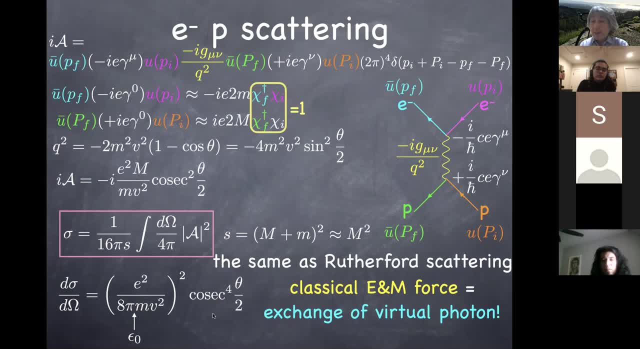 and comes out this weatherport scattering formula. But classical E and M is actually obtained by exchange of a virtual photon. So when we think of forces in classical mechanics we think of a quantum field theory as an effect of exchange of virtual particles. So given this idea, we say photon is a force carrier of electromagnetism. 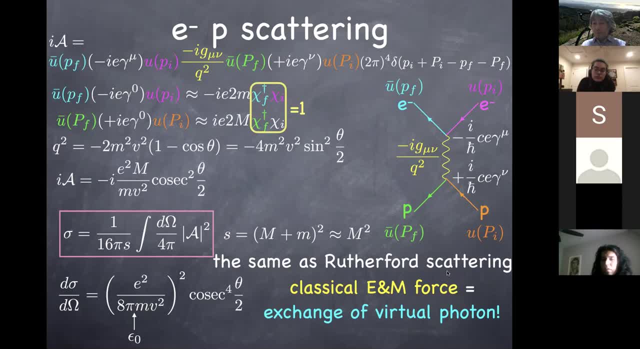 Weatherport scattering, of course, happens because of the Coulomb force between electron and proton, And we now understand the Coulomb force as a result of exchanging virtual photon, And that's the way QFT describes a force, And this turns out to be fairly general When you talk about the weak force. 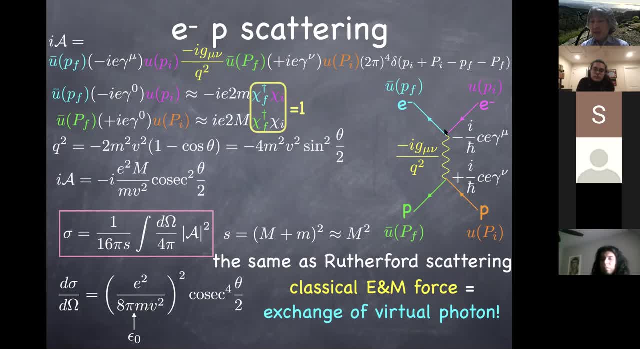 which is responsible for the nuclear beta decay. you exchange a different particle called the W boson or weak boson. So W stands for weak, And by sending a virtual W boson you mediate the beta decay of neutron into proton, electron and anti-neutrino. We briefly talked about that. 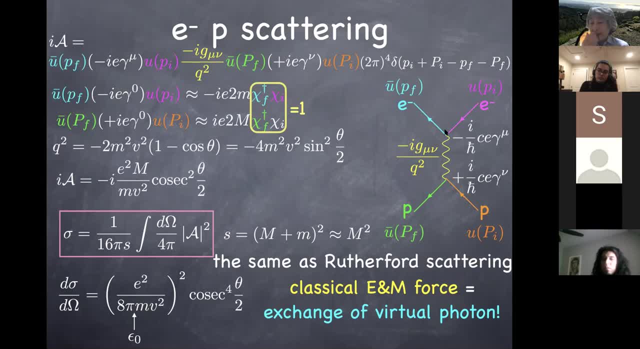 So force, which we learn in classical mechanics, is actually due to exchange of virtual particle. Force comes with this force carrier particle And for electromagnetism, force carrier particle is the photon. Exchanging virtual photon is the true nature of electromagnetic force. That is the description in QFT. 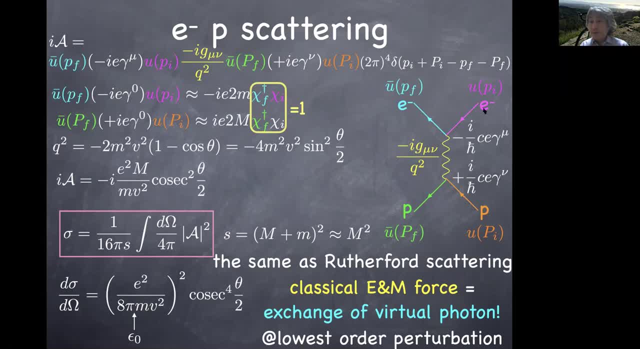 But there's a little caveat. We worked out this Feynman amplitude at the lowest order and perturbation theory. So if the exchange of virtual photon at the lowest order and perturbation theory is what corresponds to classical electromagnetic force, higher order and perturbation theory give you corrections. 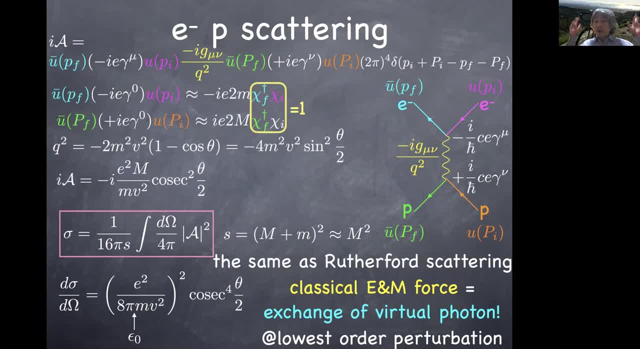 of classical description And that will be the quantum corrections to the classical theory. And you will see some examples of this quantum correction very briefly towards the end, But anyway. so this is a new idea And this is quite natural in QFT, of course, because QFT is supposed. 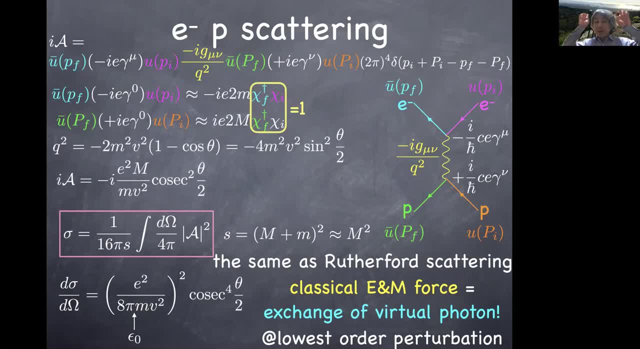 to unify the idea of particle and wave. Everything is particle and wave at the same time. So this is again the theory of quantum correction, So that's the formulation built into quantum field theory, And everything that happens in nature then is described by sending particles back in force. 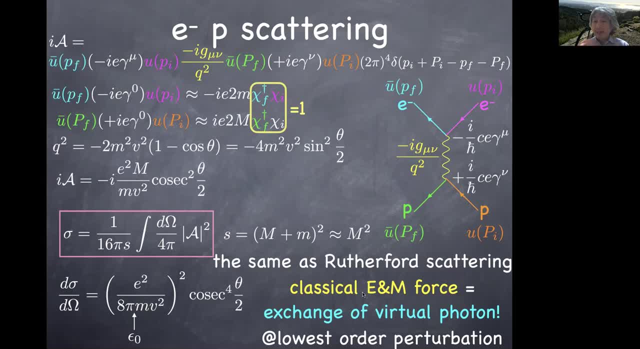 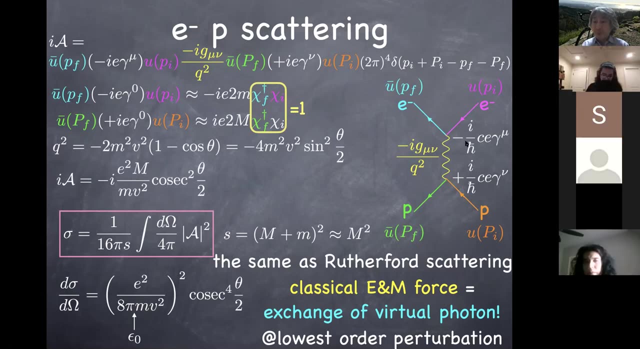 like in this Feynman diagram And that ought to describe what we know already in classical theory as a limit. And here it comes, You do get the correct limit at the lowest order- and perturbation theory. So the Coulomb interaction or in general classical electromagnetic force is now described. 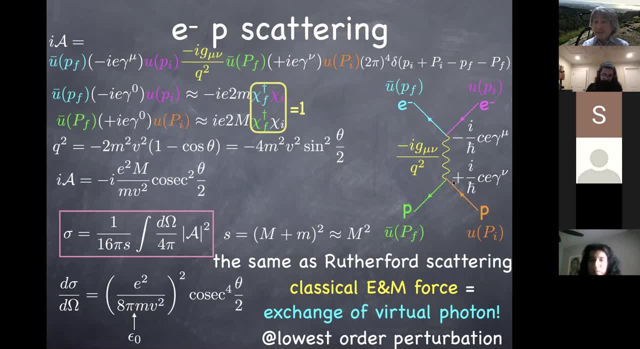 by the exchange of the virtual photon. That's a new concept But we didn't have to put in this new concept. It just came out from the formulation of the quantum field theory. But I'm just emphasizing that we now have a new view on what we think of a force really different from what 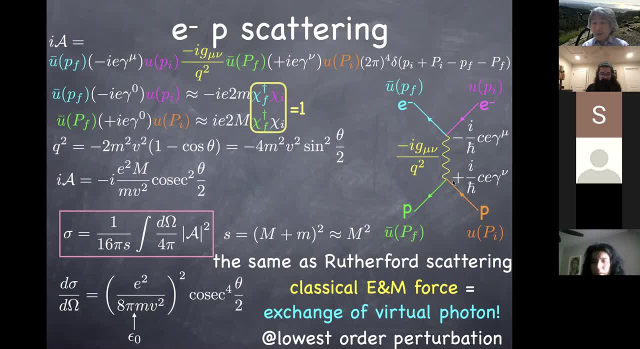 we used to think in classical mechanics: Okay, any questions about this. This is a kind of philosophical point, So I'm sure you've got questions about that And this might be a little bit tangential. but is there a connection between like. 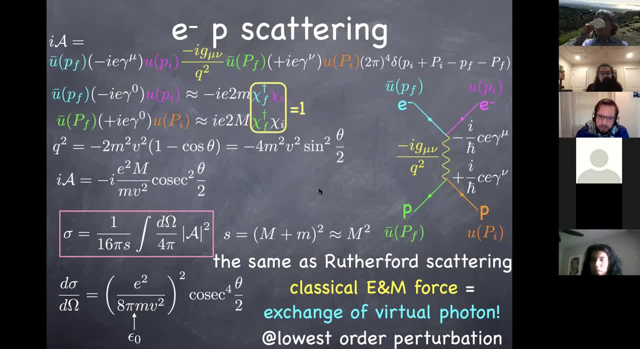 what order an electromagnetic effect takes, Like what rank of susceptibility tensor? we would need to describe it And something about the Feynman diagram that describes it. I'm sorry, I don't quite understand this question. Can you repeat that? So if we have nonlinear optics effects, 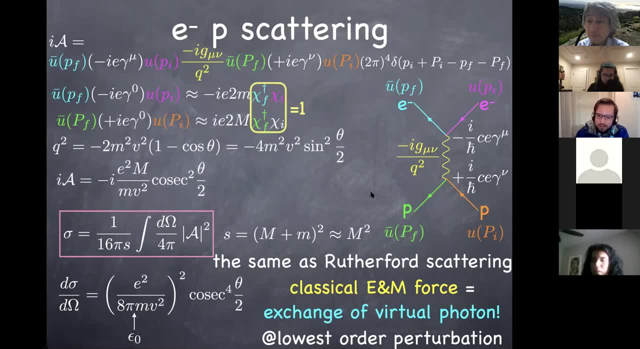 a lot of them seem to have names that imply they would be described. That's a nonlinear effect described by more complicated Feynman diagrams, like two-photon absorption. Is there like some formal rule we can draw between, like the rank of the susceptibility tensor associated with some? 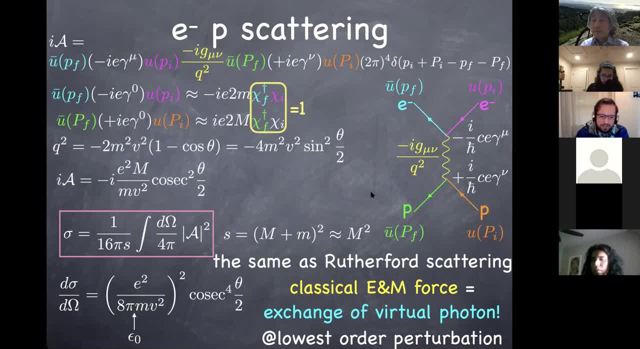 non-linear optics effect, the Feynman diagram associated with it. Okay so non-linear optics effect is definitely a quantum effect. So in the case of this proton scattering, when end result end up not having any h-bar in it, right? So that's why this is the same as a 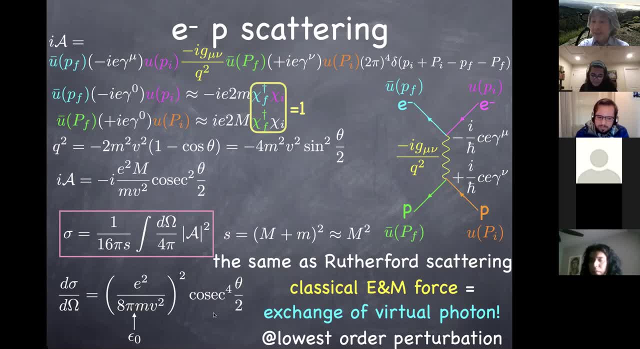 classical result. But when you go to high-order processes, like in non-linear optics, then you end up having other pieces which do depend on h-bar because it's high-order in perturbation theory, and then you see that that's genuine quantum effects which you don't have in classical. 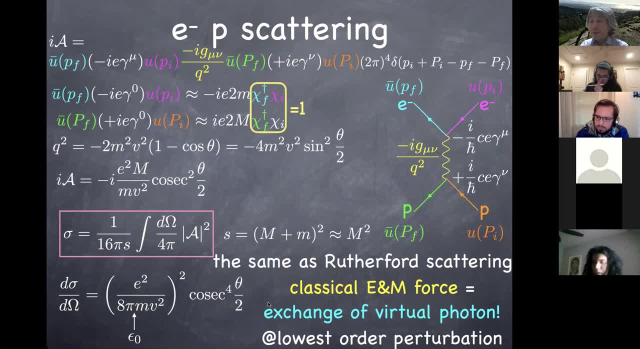 description. Am I answering the question? Yeah, Not quite. Well, we do come back and talk very briefly about these high-order effects and genuine quantum effects later on, so maybe you can ask the question at that stage. Is that okay, George? 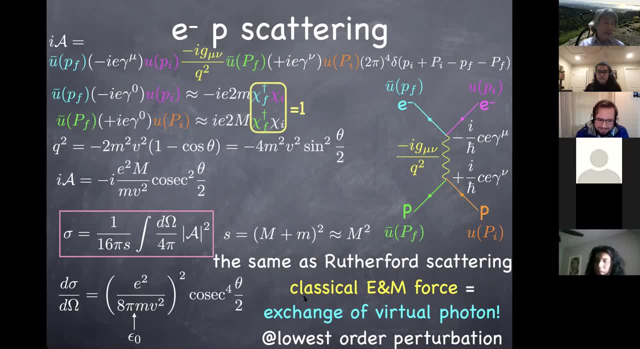 Sure, Okay, Any further questions on this slide. Now you see everything in action, Just like physically. is there any interpretation of this virtual photon? I mean, I guess it makes sense in theory, but in terms of like physical reality, how should we best interpret it? 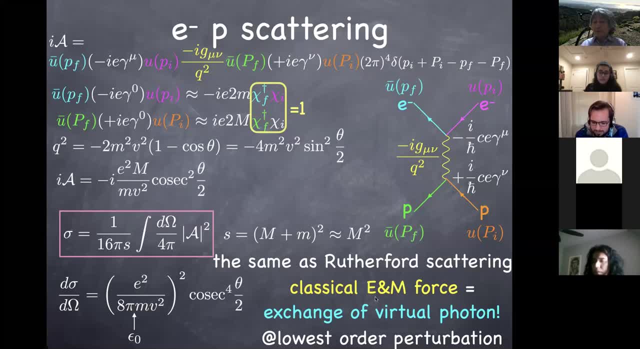 Yeah, So in some sense electromagnetic field is a coherent state of the virtual photon. When you have a, for example the Coulomb potential, the Coulomb potential is static potential, But when you have actually particle moving, then of course Coulomb potential elsewhere. 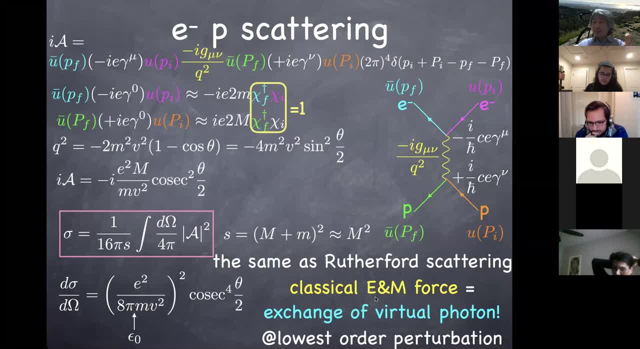 cannot catch up because there's no information going faster than the speed of light. So information has to propagate from something moving from here to there, or something else is going to interact in the Carrie to where your, in particular, movement in the bottom right of the spectrum. 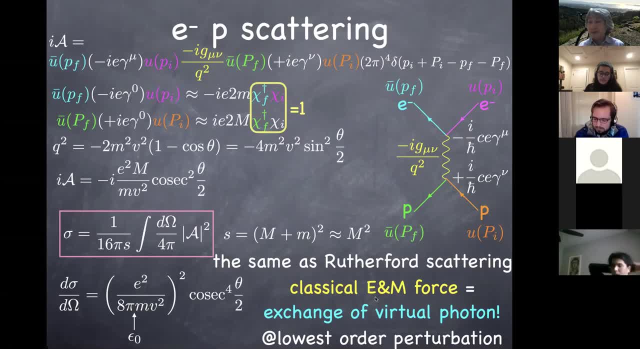 to where you're measuring. so there is something actually moving from here to there And that thing is actually the virtual photon, intuitively. Does that make sense? I see so it's. it's like the queria. I guess It makes sense. it's like the carrier. that. 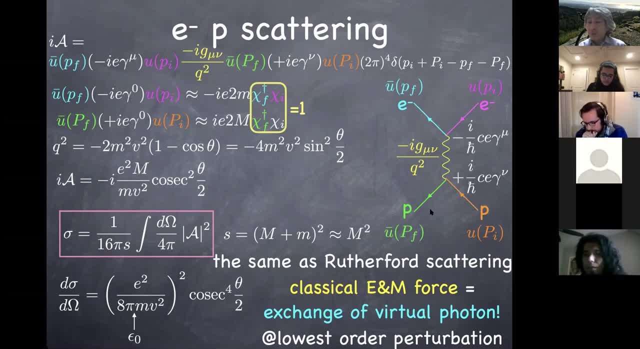 sends that Coulomb potential to another location, That's right. Right. then the electron gets affected by it. So you need to send that information using virtual photon from proton to electron, so that electron knows how it should get scattered as a result. 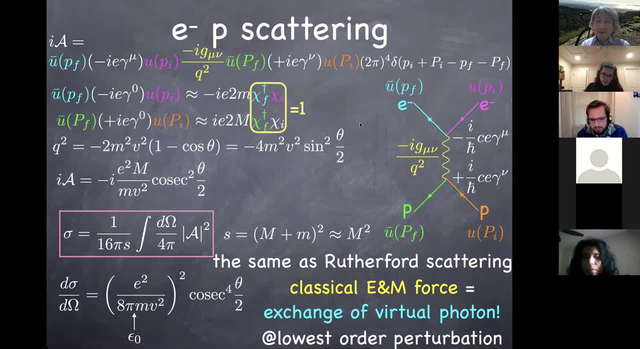 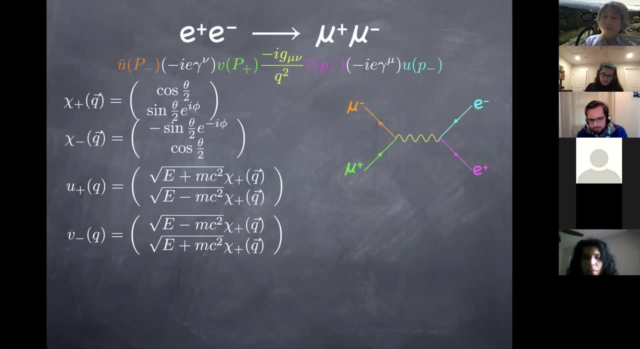 So that's sort of the intuitive picture of this. Yeah, that makes more sense. Okay, So let's look at the other example of this: electron positron to mu plus, mu minus, And in this case I take the opposite limit of the massless electron, mu one. 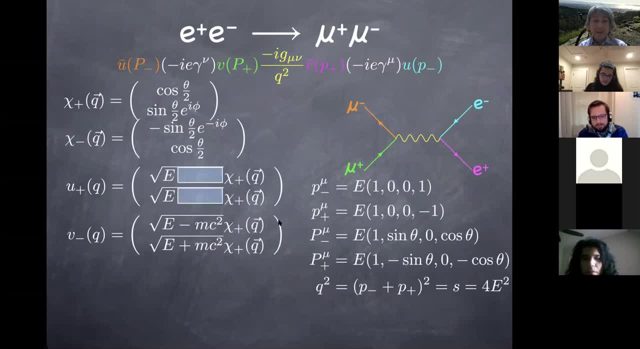 so that I can forget about mass terms. And then again the spinors simplify And full moment also can be written in a very simple way. in a center of momentum frame, Electron, positron come into the center from both direction. That's a collider experiment. 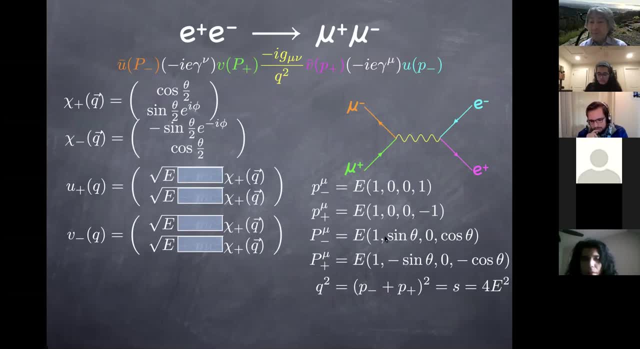 And mu plus, mu minus go out from the center in some off direction given by this polar angle theta. I took the frame where polar azimuthal angle is zero, just for the purpose of convenience, And then you know you can just again. 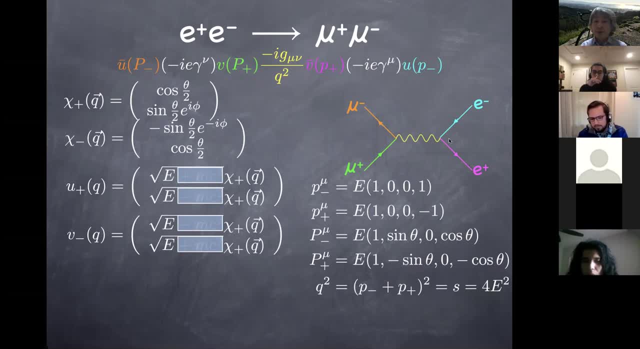 just put in these positive energy solution, negative energy solutions, as we described in the solution to Dirac equation, into this formula, And in this case Q squared has energy but no momentum Because if you look at the initial state, energy is E, momentum, E for the electron. 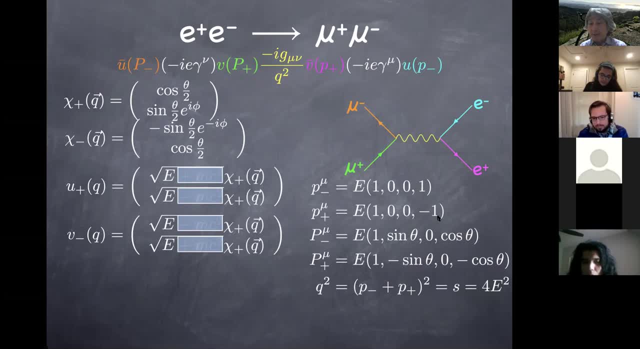 And for positron comes in opposite direction. so momentum is minus E, So spatial components cancel, but the time component remains. That's the total energy: 2E now. So the Q squared for the full momentum of the photon is 4E squared, which is nothing but the center. 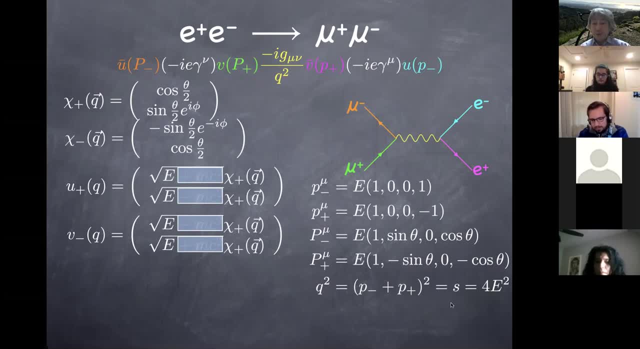 of momentum energy squared, which is the variable S I introduced earlier. So again, you know everything in this expression. You just plug them in and compute it. Here I decided to take particular helicity combination, that particles, electron and muon have positive helicities. 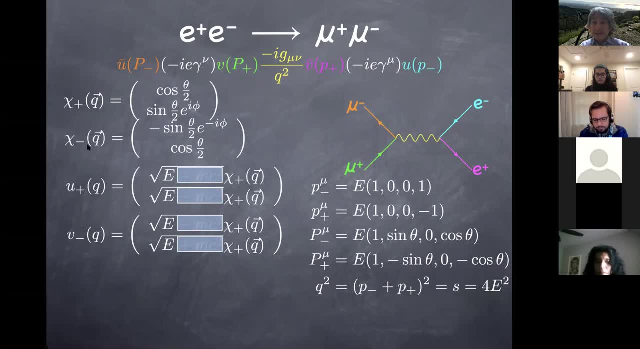 Antiparticles, positron and antimuon, have negative helicities. Then you just plug them in here and amplitude is very simple: IE squared one plus cosine theta, And you can understand this behavior. one plus cosine theta. because I chose this helicity combination. 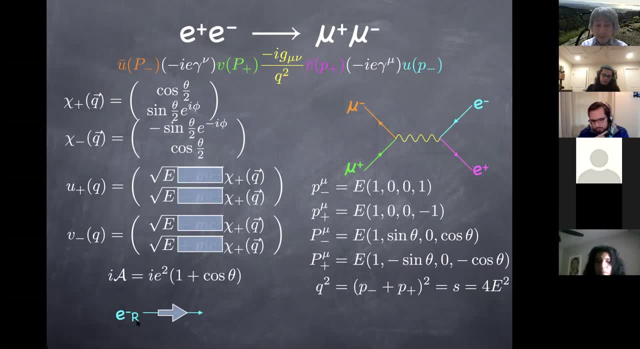 that electron has positive helicity right-handed, positron has negative helicity left-handed. So if you look at this direction along the beam, the two spins add up, so there's a negative helicity and that's the angle of momentum one. 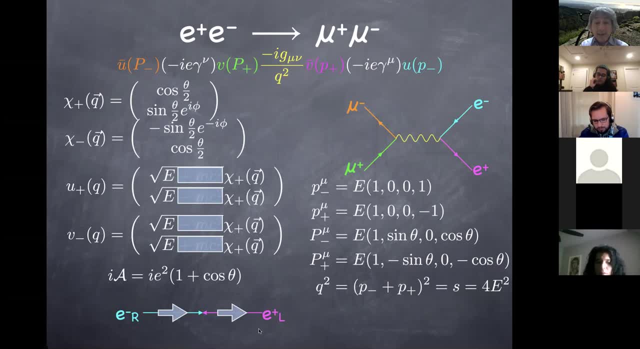 along this direction of the beam And from here electron, positron, annihilate, disappear from the universe and then out comes a muon and antimuon, And again I chose these helicity combinations. So there's again net spin, one along the direction. 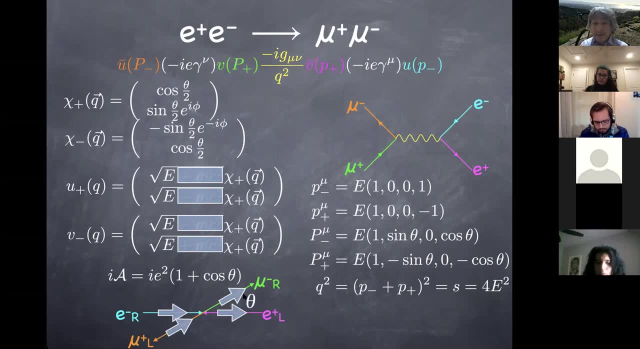 of the muon momentum And theta is this angle over here. So initial spin one along this direction has the maximum, maximum overlap with spin one along the muon direction when this angle theta vanishes. But when theta goes all the way to 180 degrees, initial state has spin one in the positive. 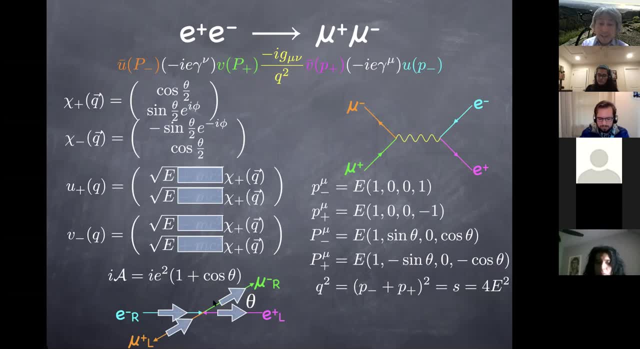 z direction. final state would have spin one in negative z direction. then angular momentum wouldn't be conserved. That shouldn't happen and therefore amplitude vanishes when cosine theta is minus one. So this behavior of one plus cosine theta in the amplitude makes sense. 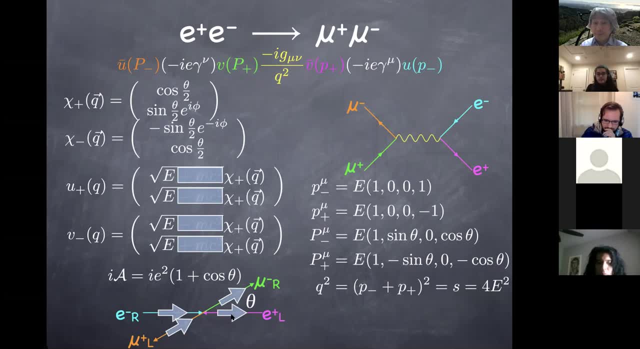 from the conservation of the angular momentum conservation. So amplitude is very simple. Again, you stick that into the master formula and out comes the cross section. Any questions about this? I have to wrap that very quickly. Okay, so then I put that into a 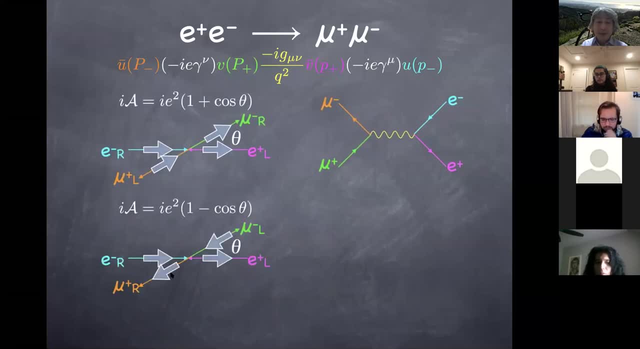 formula for the cross section. And if you have the opposite helicity combination for muon, again it's clear from this picture that I end up with one minus cosine theta instead. So when you compute the cross section like this, you don't have the polarized beams typically. 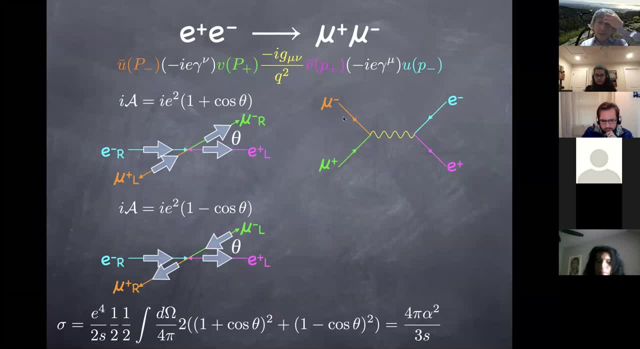 So you sum over both helicities of incoming particles, you sum over both helicities of the final state particles, and because you sum, then you have to do the averaging over spin for the initial state. So that's one half for electron, one half for positron. You put all of these things. 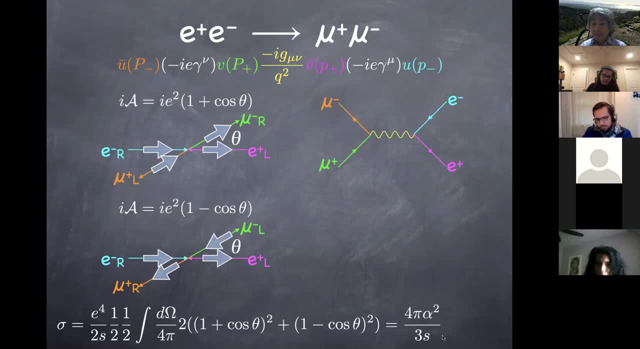 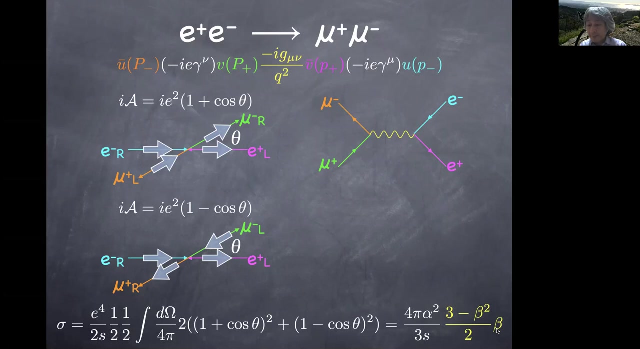 together and out comes the total cross section. And if you actually retain the finite mass for the final state particle, then you have this beta factor. So in this case, beta really means the beta of the relativity, namely velocity over speed of light. And so it starts. 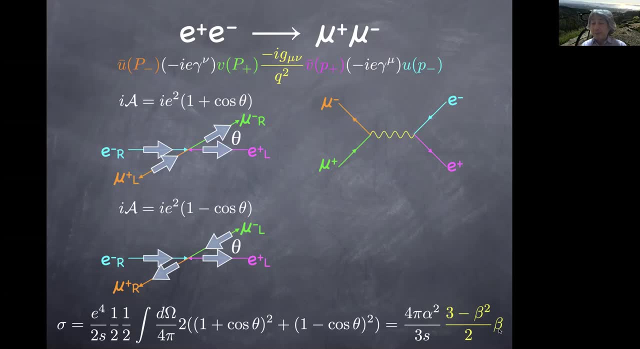 with beta, which means that when the total energy of the system is just enough to produce the sum of the particles and the velocity over speed, then velocity vanishes, cross section vanishes. so cross section rises from zero as beta and starts to saturate, and then 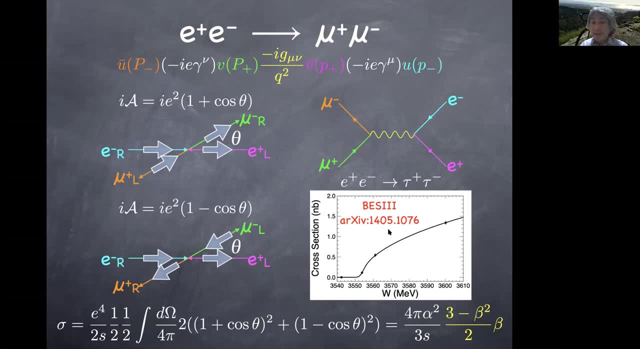 eventually starts to go down. And this is an experiment: data from an E plus E minus collider accelerator in Beijing, Beijing Synchrotron, and producing yet heavier version of the muon called the tau. And this is a third particle- So tau is meant to be tertiary- which is originally discovered across the bay at Stanford, at SLAC. 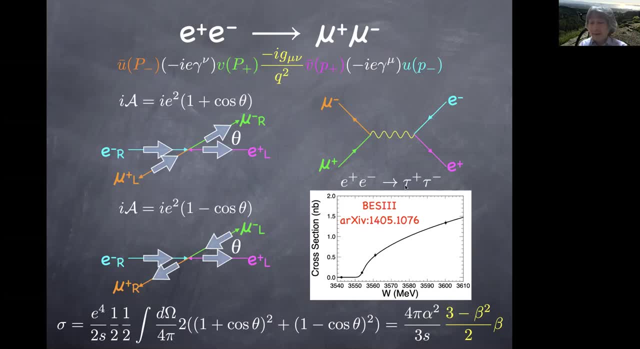 And so using this tau, which has a fairly heavy mass, even heavier than proton, you have this beta behavior coming in. This is something you can compute yourself if you retain the finite mass of the final state particle And then experimental data and theoretical curves exactly match on with each other. 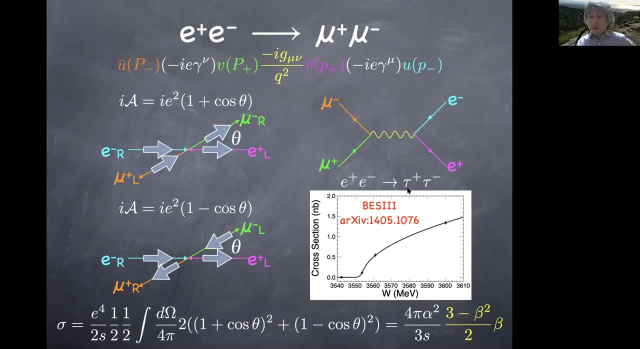 And this is the way you can actually measure the mass of this particle called tau. So that's how you can compute this process, which you could never deal with in quantum mechanics, because particles disappear, particles do appear. But now you can talk about this kind of process and you know how to compute the physical observables for that process as well. 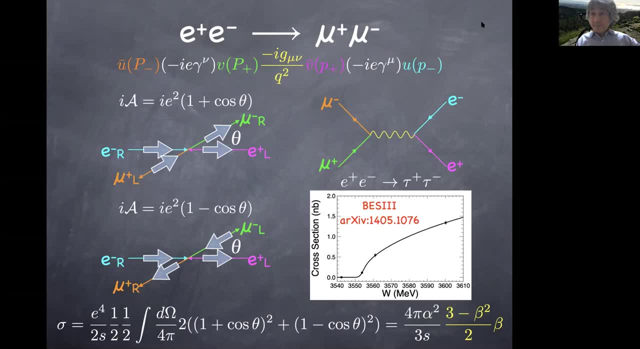 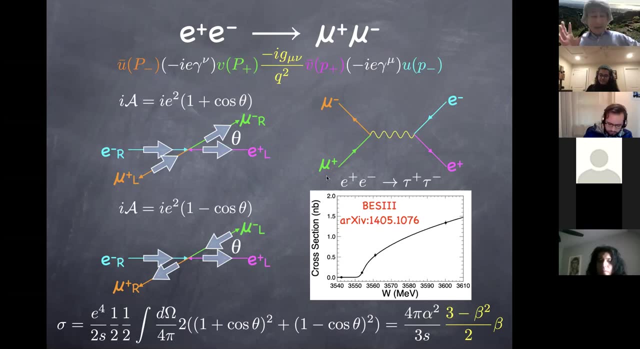 Any questions about this? Okay, so I apologize, but let me spend maybe five more minutes to go through what may be coming in the graduate level, QFT, where you actually do study these quantum corrections George was asking about. It's not the same example, but something similar. 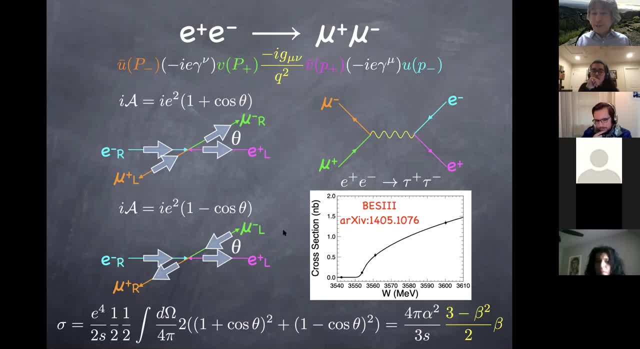 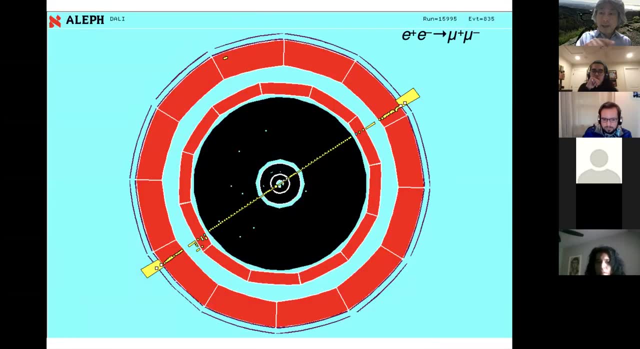 But before going there, I'd like to show you that this process really does. It does happen experimentally, and here we go. So electron beam is coming from your side into screen. positron beam is coming from the other side of the screen to the screen. they meet right in the middle. 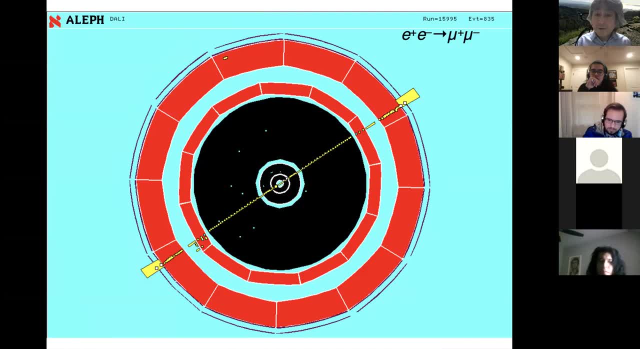 And then out comes pair of muons and this track means it's a charged particle, but it seems to penetrate all the layers of detectors to the very end, which means this is a very penetrating particle and it has to be a muon. 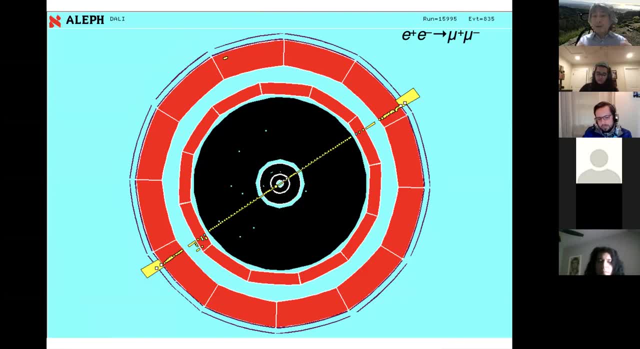 And so this is how, From positron in your experiment, really disappear from the universe and become a brand new particles, namely muons, created from the creation operator in QFT. and you're observing that- And this is clearly different from E plus E minus, going to E plus E minus, where electrons don't annihilate, because electrons shower so much energy in the material and they stop here. 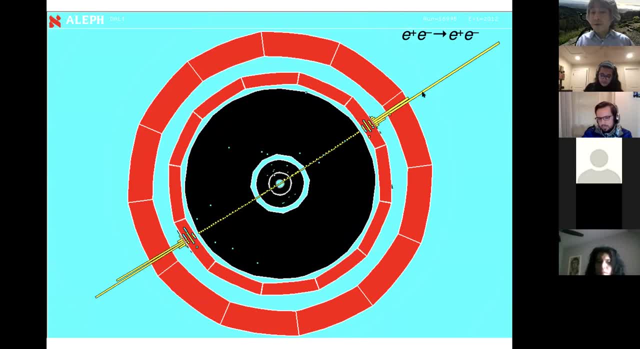 This is called Electromagnetism, Electromagnetism, Electromagnetism, the calorimeter, and it doesn't go all the way to the end of the detector layers. So this is the case of the electron. So we know the previous picture is not electron In the case of tau. 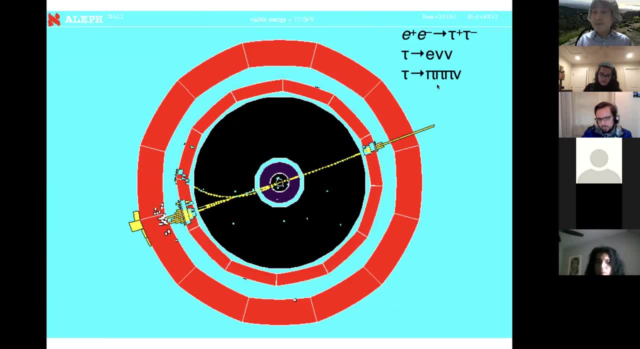 it happens in a very similar way, But tau is an unstable particle that can decay fairly quickly, within about a picosecond. So it happens within the detector volume And what you're looking at is the decay products of taus. But once again, you have a very clear interpretation. 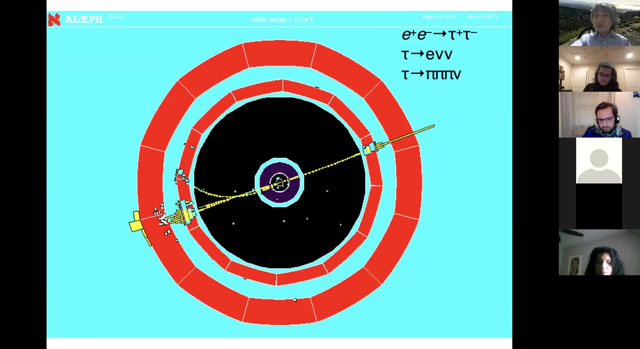 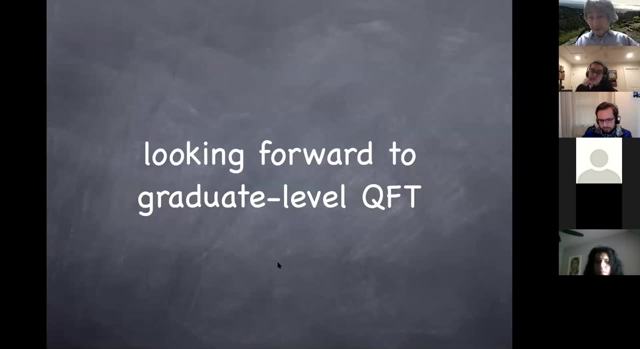 And if you look at the angular distribution, that actually does match up with the angular distribution we worked out in the Feynman diagram. So these things really do happen experimentally. So let me just very quickly give you some upshots on what you might expect. 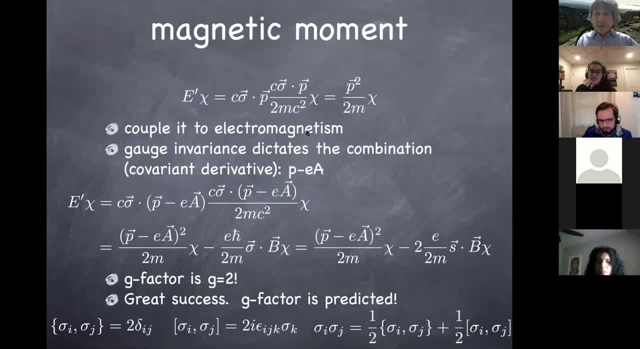 when you go to the graduate level, QFT. So we talked about g factor being two. Now that we learned that all the forces have to do with a virtual photon, that magnetic field is also a virtual photon. So g factor: you compute it in your homework problem. 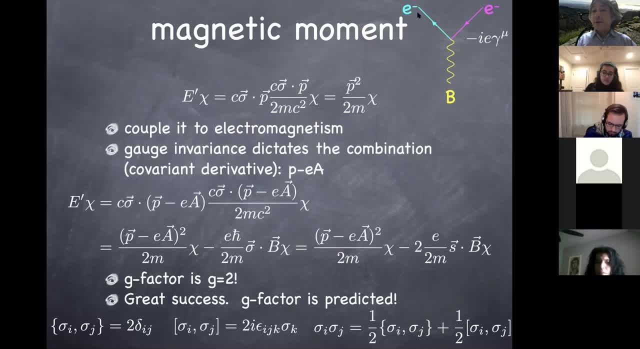 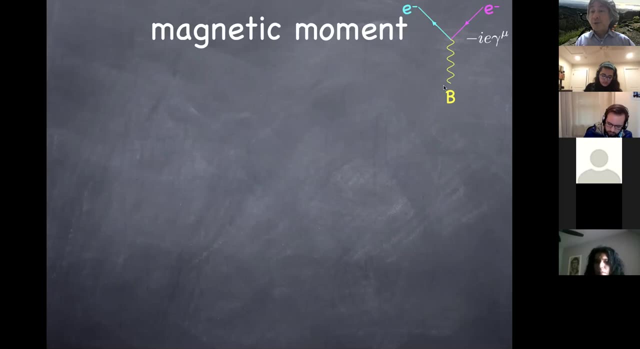 basically corresponds to this diagram of electron feeling, the external magnetic field, which is basically this virtual photon. But this is the lowest order perturbation theory, as I emphasized. If you go to higher orders, you have this process too, where you exchange virtual photon between initial and final state. 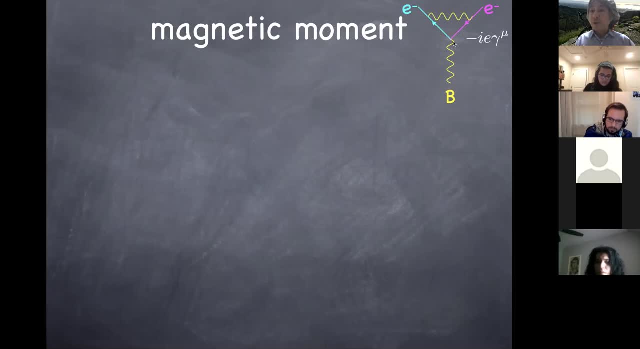 And this is what is called the loop diagram, because you have a closed loop in the Feynman diagram. If you go ahead and compute this, it turns out the g factor is no longer two, And I think Wendy was asking this question that you heard. the g factor is not two. 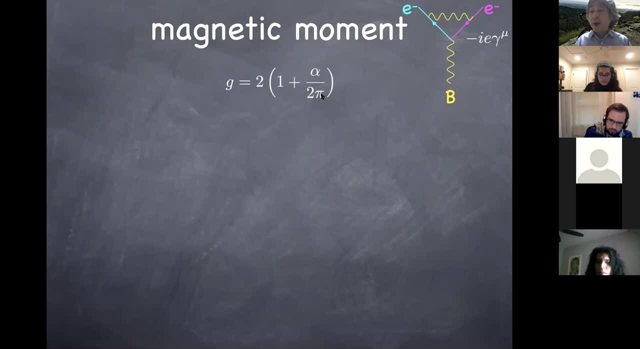 exactly, but there is a correction by alpha over two pi. that disorder perturbation theory. This is something you can work out. It's a definite prediction of quantum electrodynamics And of course this is the first correction at order alpha. 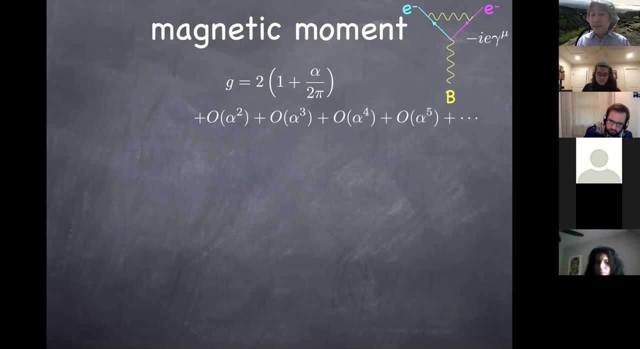 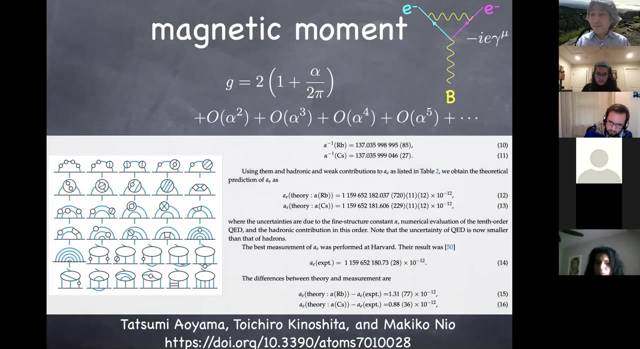 There are further corrections at higher orders in alpha And amazingly, some people do compute these things by looking at Feynman diagrams like these. It's amazing Some people actually compute these guys. But having done these computations you get very precise prediction on the g factor of electron with an accuracy of 12 significant digits. 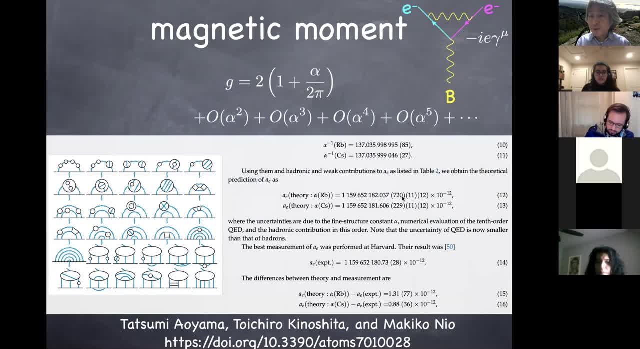 and there is uncertainty in theoretical prediction and that's because we don't know fine structure constant that well, which relies on experimental measurements. so if there were no experimental errors on the measurement of alpha, then you would have the theoretical prediction on the g factor with 12 significant digits. also, amazingly, people have measured the g factor of 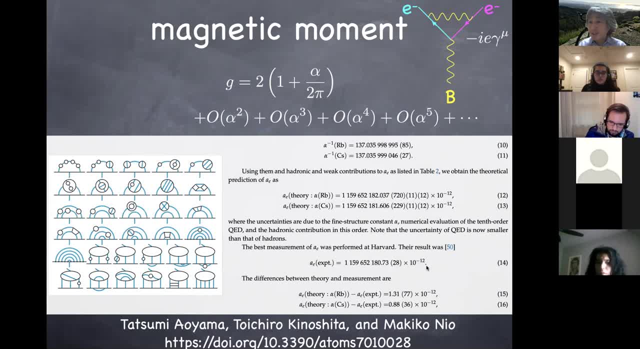 electron with 12 significant digits and within the errors in alpha itself. they all agree. here is the difference between theory and experiment relying on two different measurements of the fine structure, constant, but both of them, basically, are zero within the error, maybe two, three sigma error here within 12 significant digits. it's incredible. this is the level of 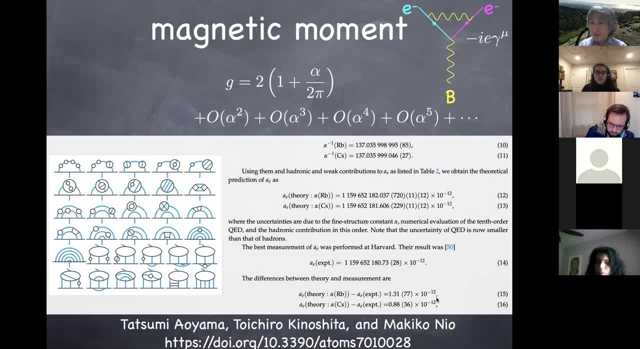 success you get out of quantum field theory. it's a probably the triumph of the entire 12th century physics, and this calculation is now still going on in 21st century. so QFT is really amazing and successful. so QED is the best physical theory ever. 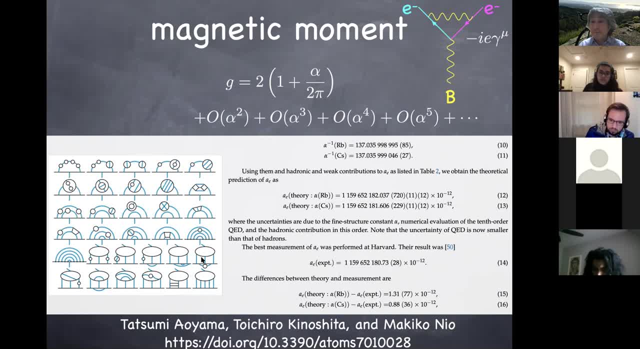 and that's why people came up with this acronym of QED, I believe, and these calculations have been pioneered by Toichiro Kinoshita at Cornell University, and he is now old and retired, and it is now carried on by his student, Makiko Nio. so he is. 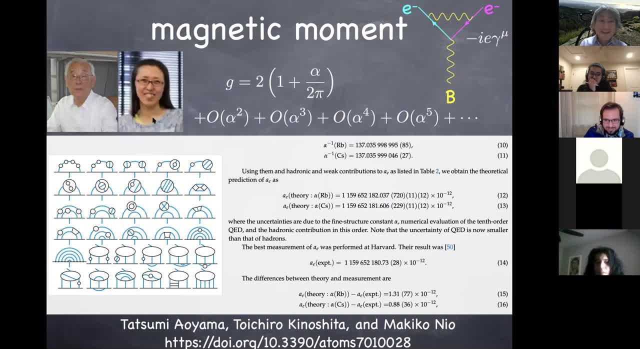 the Kinoshita. so the karate master, sensei and his disciple Makiko, is now carrying on to the next generation and they are now looking at this. five loop diagrams and so and so forth. you have to do supercomputer for this, but anyway. so this is the level we can test. quantum field theory. 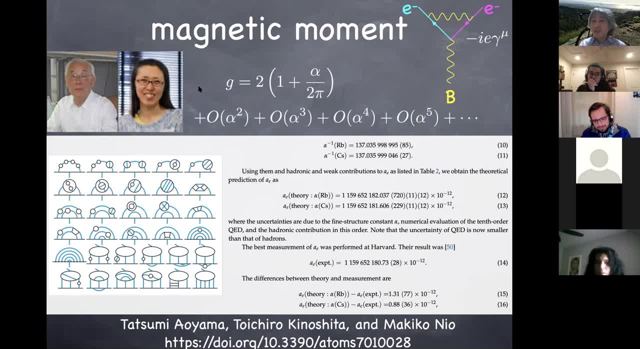 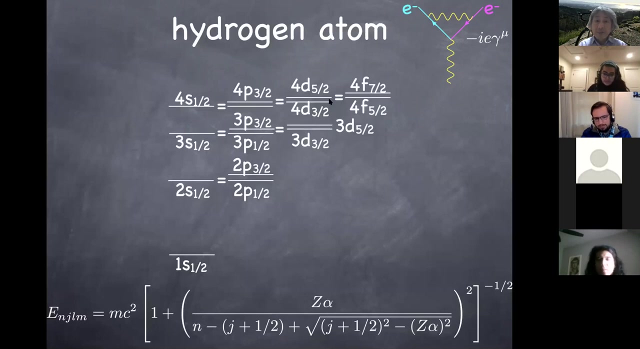 an incredibly successful theory. so here you see this example that classical electromagnetism is really the lowest order. you do have higher corrections coming from quantum effects, but they are predictive in perturbation theory, in quantum field theory, and they work incredibly well. here's yet another example. I talked about Dirac equation in in coulomb potential and one thing: 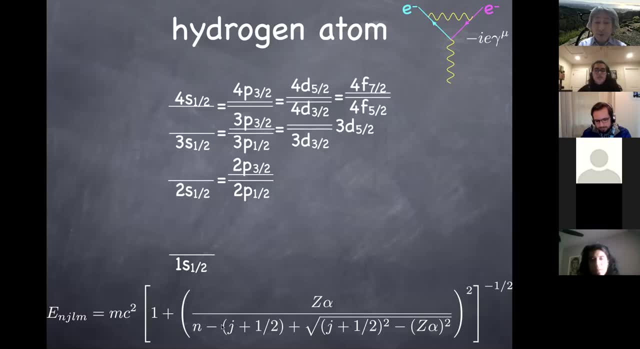 that was remarkable. there is that energy levels depend only on j, so that you had exact degeneracy, for example between 2s 1 half and 2p 1 half. but again because of this quantum correction, with the exchanging photon, now in the virtual photon given by the coulomb field, electric field. 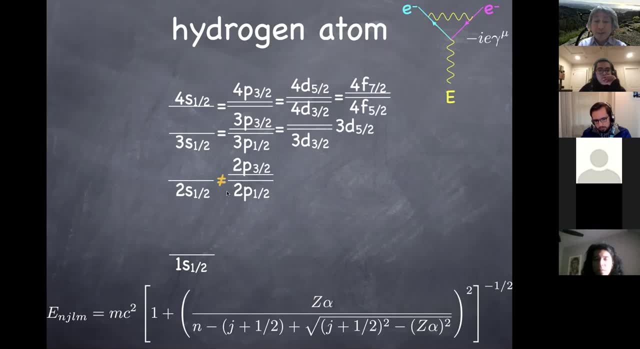 it's the same diagram, but that actually ends up making the states not having the same energy by lifting up the s-state just a little bit, and this difference in energies is what is called the lamb shift, which was measured in radio. it turns out to be about one gigahertz. so this is another. 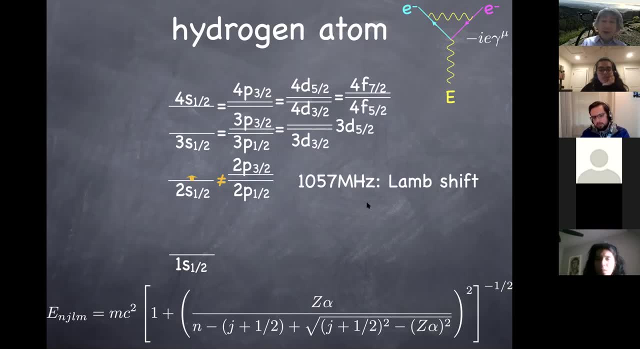 quantum effect and the lamb shift was measured right after world war ii. because unfortunate history is that many physicists walk around the world and they don't know what they're doing, and so we can actually tell that they're doing something better. they're doing something that's 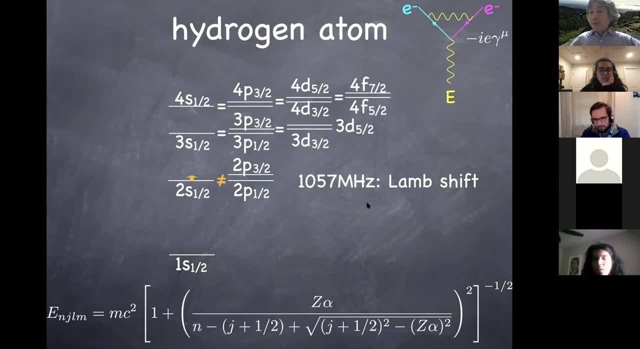 more precise, because some of the measurements of the energy見ers in the sky we can see they're not completely zero, but they're coming very close to zero. it's kind of a very nice example, and so it's the same thing, for the lecture is to be able to measure how much. 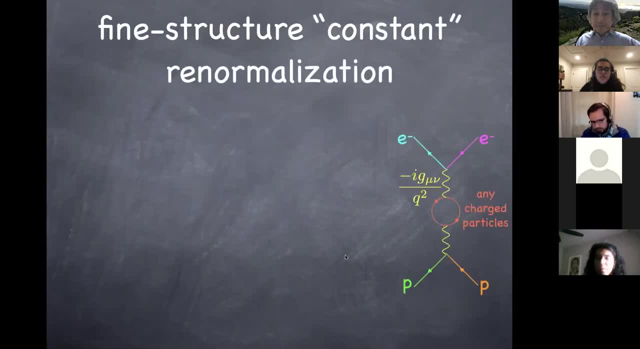 you're actually measuring with the laser, but you're also measuring how much energy. you're actually measuring based on the beam of light, and so on and so forth. so that's part of that. the is different. what you're even going to work on is to look at the measurement of the energy using the. principle of the thermal field and you're actually measuring the distribution of the energy and the temperature of the energy from the transit. so it's very interesting and I would like to the product that we have here. it's the mass of the energy which requires a certain of a huge amount of energy. 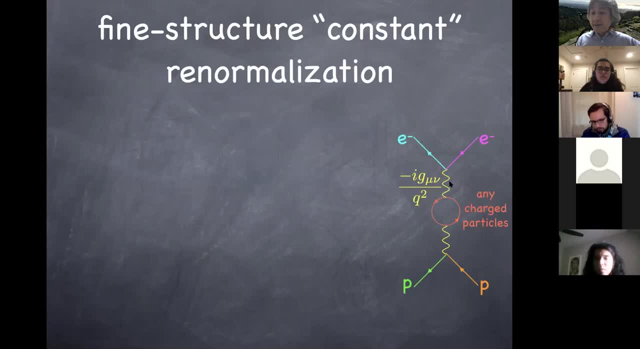 And the last example I'm going to talk about is that, again, this is the high-order diagram in electron-proton scattering. So this high-order diagram would basically make the fine-structure constant, not a constant anymore, but it changes as a function of the momentum transfer. 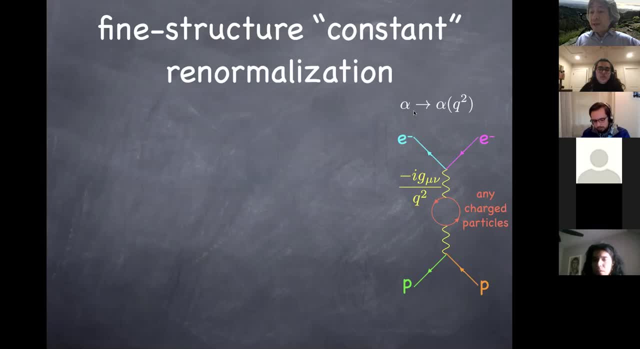 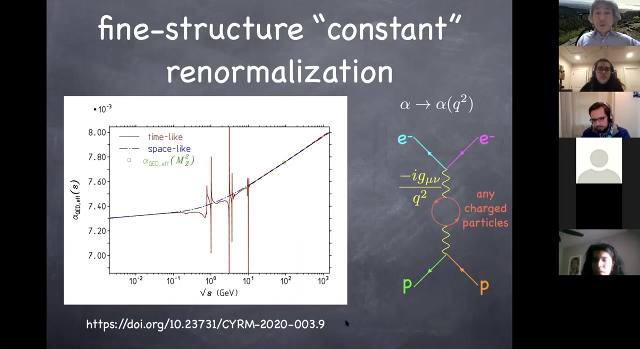 So the strength of electromagnetism is measured at zero momentum, in quantum Hall effect, for example, But when you actually measure the strength of electromagnetism at finite momentum transfer, the number turns out to be different, Which you can also compute, depending on whether Q squared is positive time-like or negative space-like. 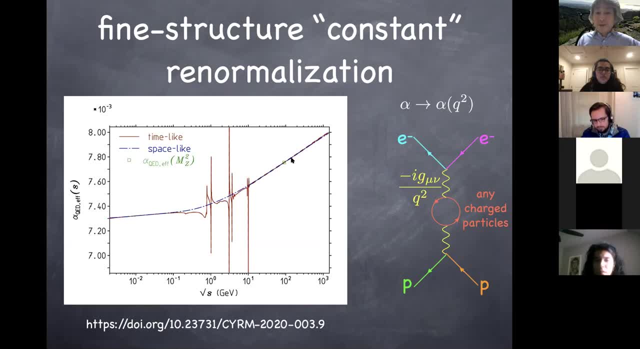 You get different predictions, But asymptotically they look more or less the same: 1 over 137 is at zero momentum transfer. But here's one data point, measured at E plus E minus collider at 0. So this is the strength of electromagnetism. 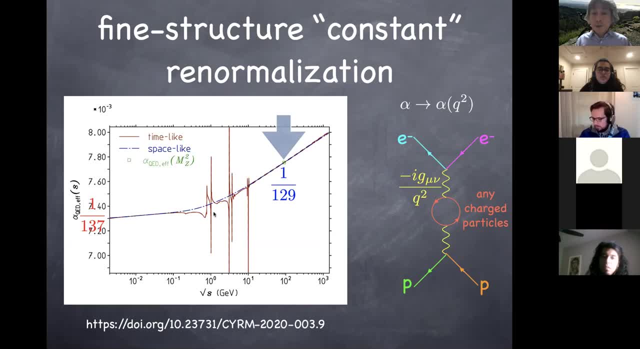 And the number is different: 1 over 129, as a course of these quantum corrections to the strength of electromagnetism, Because electromagnetism, now we understand, is a consequence of exchanging virtual photon. Virtual photon can polarize the vacuum. 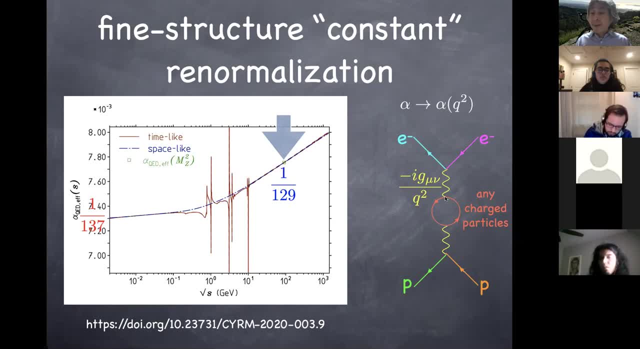 This is called the vacuum polarization diagram. in a way that depends on the momentum transfer. So the strength of electromagnetism does change. This is a function of momentum transfer And again, theory and experiment do agree. So that's yet another quantum effects that's coming. when you take the graduate-level quantum field theory class using these loop diagrams, 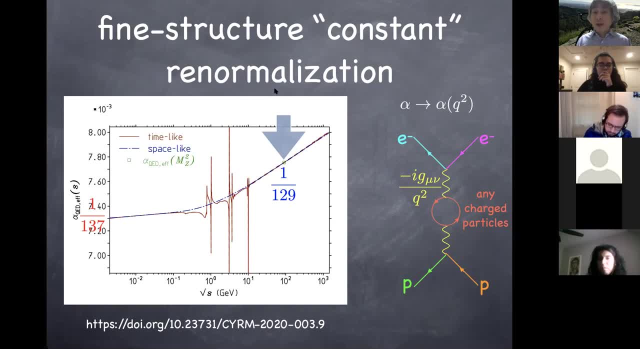 So this is one example of the process called renormalization, which you will hear a lot when you go to the more advanced quantum field theory classes. Okay, so that sums up everything I wanted to talk about. I talked about this stuff first half. 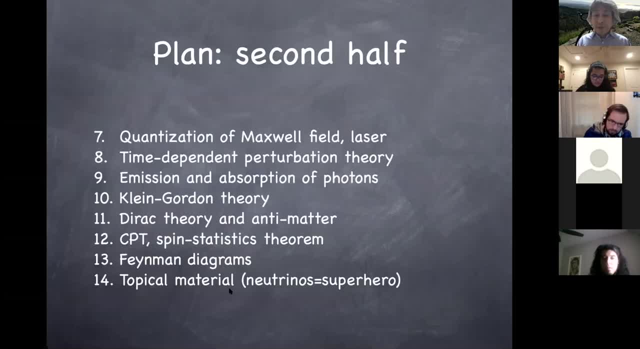 This stuff, the second half For topical material. I chose to talk about neutrinos being superhero who might have saved us from the complete annihilation, right, So that was a topical material. But now you see everything I have advertised at the beginning. 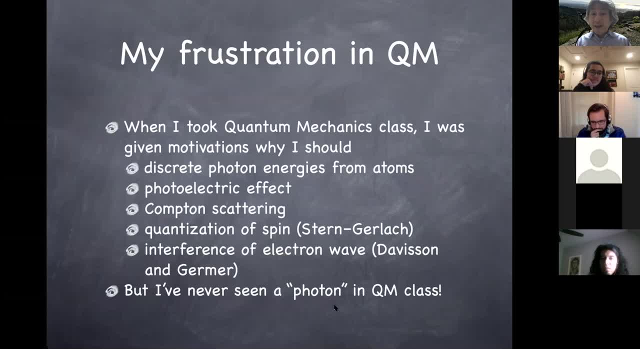 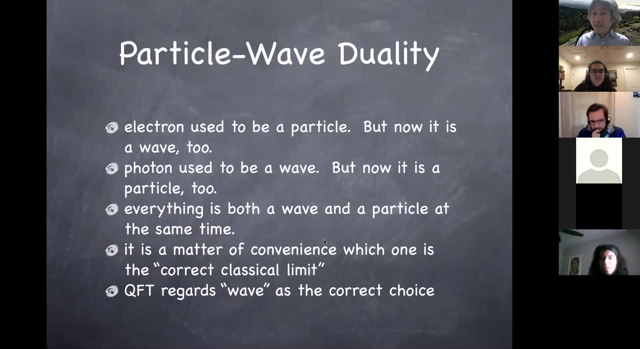 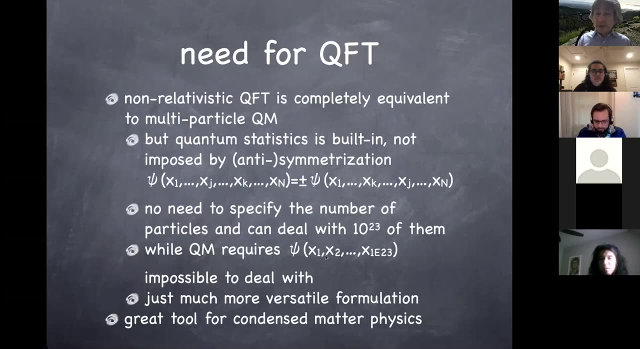 So I said, you never see a photon in quantum mechanics class. Now you do see a photon a lot in QFT And particle wave duality is built in In QFT. Antisymmetrization in quantum statistics is also built in. 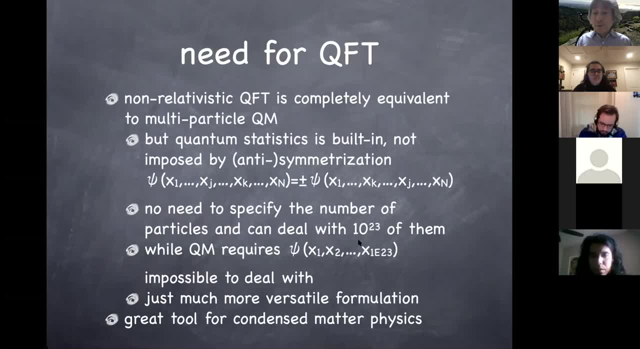 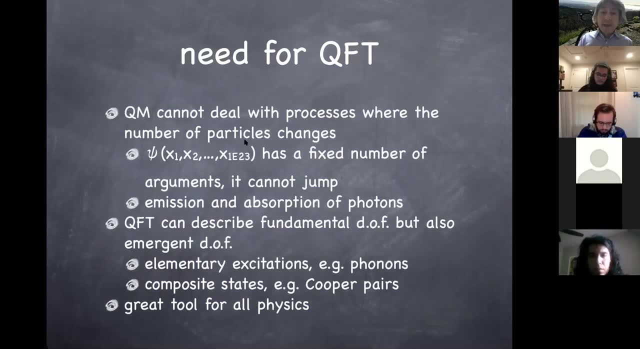 And you can deal with macroscopic number of particles without any problems using QFT formulation. It's a great tool for condensed matter physics And you can now talk about processes where number of particles can change. We just computed electron positron disappearing from the universe, leading into some other particles appearing. 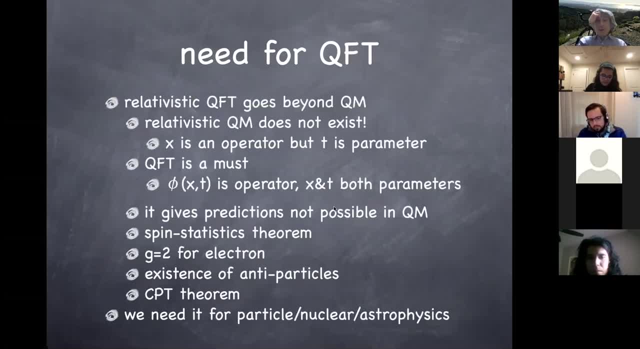 So you can talk about the process. And then relativistic QFT goes beyond quantum mechanics for sure. So now position is demoted from an operator to a parameter. Field is an operator instead And gives new predictions like spin statistics, theorem, G-factor of the electron. 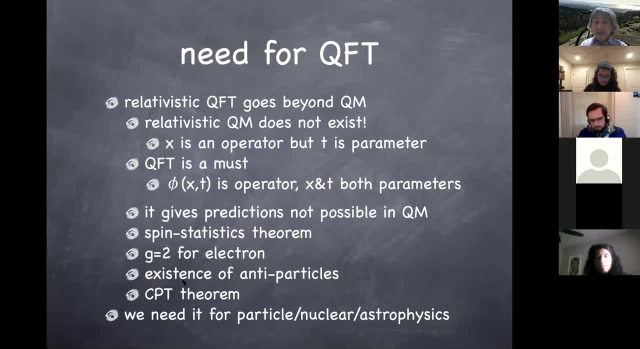 Two at the lowest order, Corrections at high orders. Existence of empty particles: predicted by Dirac, It was confirmed by Anderson. cosmic rays: We talked about CPT theorem. So we need this for really many, many different branches of physics. So that's the summary of QFT we talked about today. 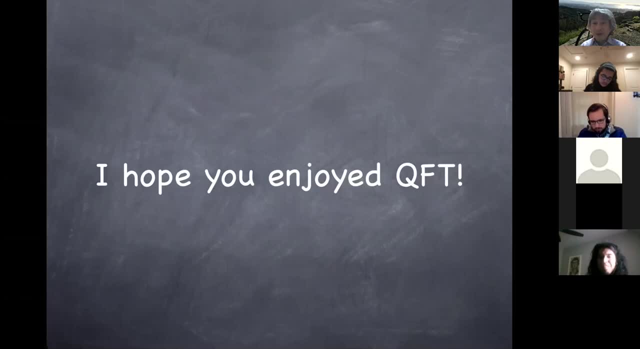 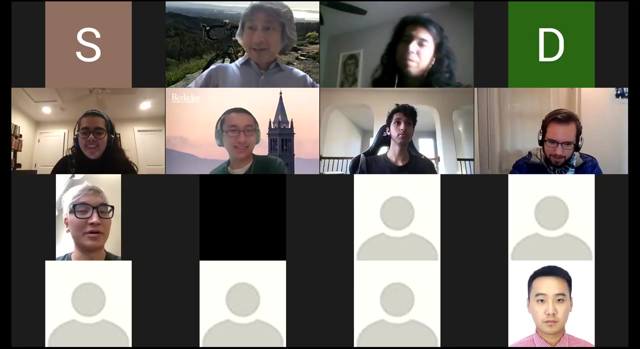 So I hope you enjoyed quantum field theory And I hope you continue to study the subject at the grad school sometime in the future. Okay, That's it. Thank you everybody. Thank you, Thank you. Any questions? I went over time. 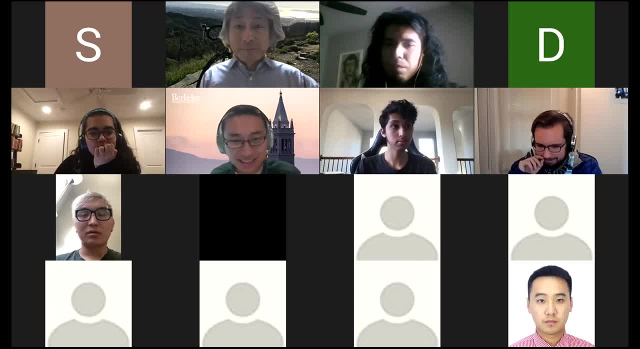 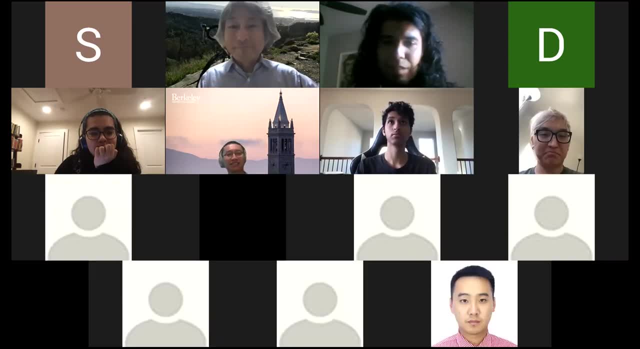 But I still welcome questions if you have any. Oh, you're welcome, Elijah. Okay, You're always welcome to send me emails or Piazza or B courses. So if you have any questions, just don't hesitate to ask me, Okay. 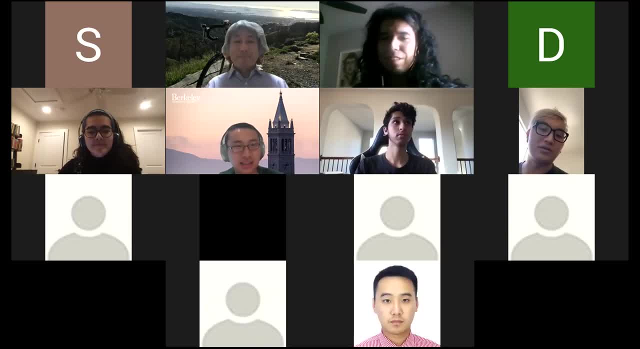 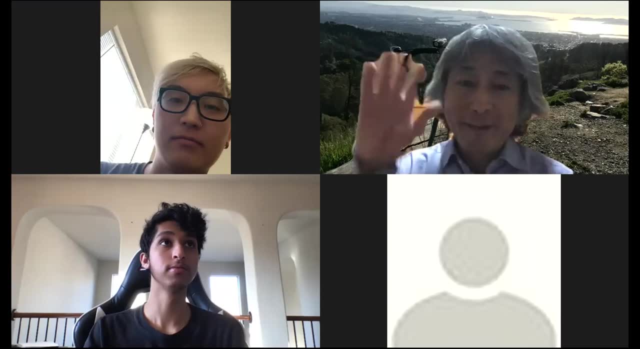 Have a good weekend And good luck with your exam, Thank you. Thank you, Take care, Thanks. Thank you, You're welcome. Bye.